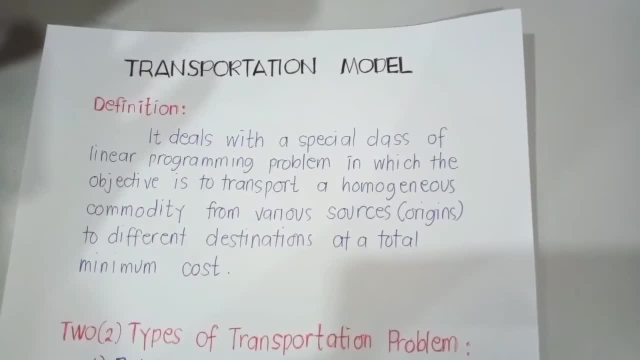 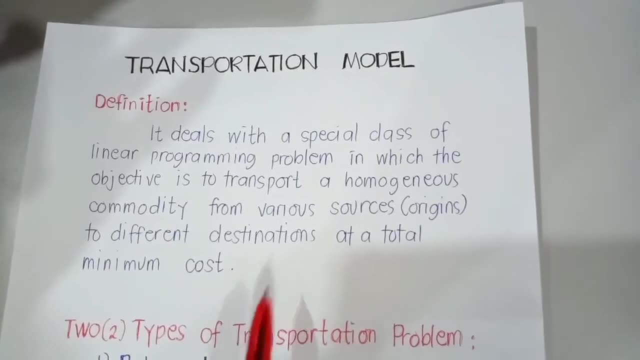 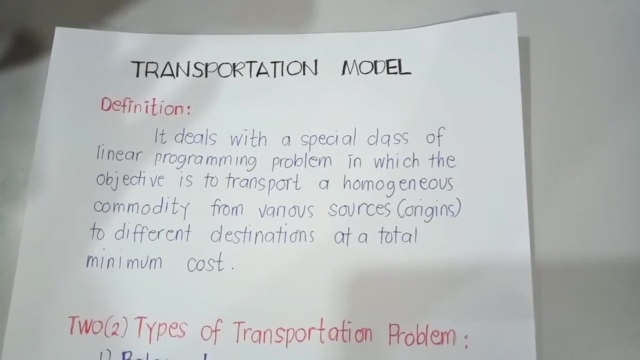 most of the time, as you can notice, companies are logistically challenged when transporting their products from one place to another or from one destination to another. okay, And for this matter, the ultimate goal of transportation model is to find out the optimum transportation. 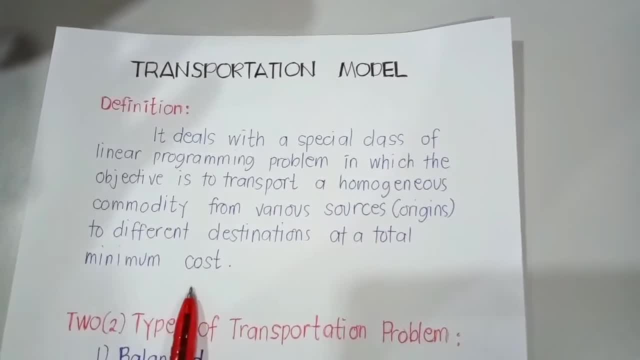 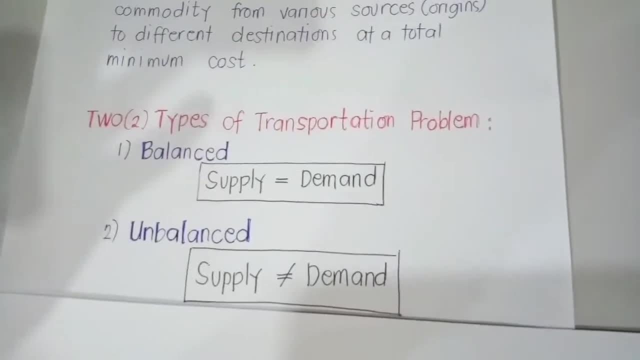 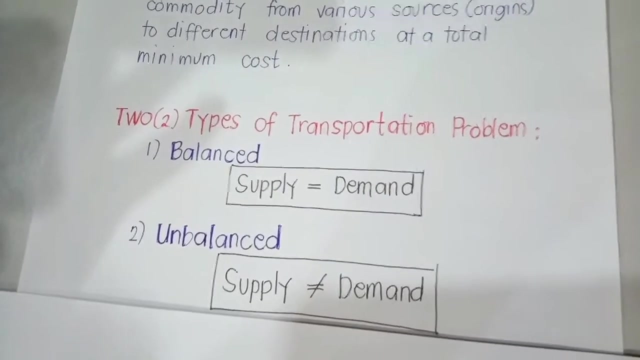 schedule, keeping in mind the cost of transportation to be minimized or to be at minimum. Now there are two types of transportation problem. First we have balanced and second we have unbalanced transportation problem. When we say balanced transportation problem, 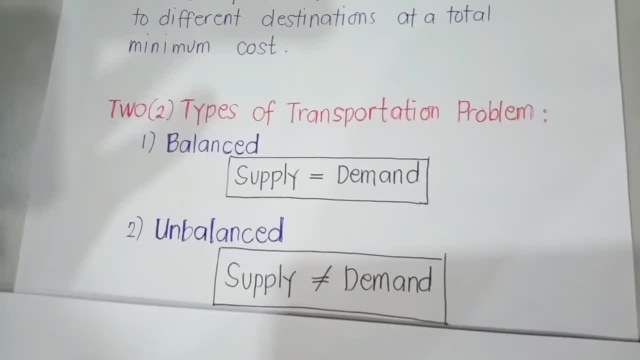 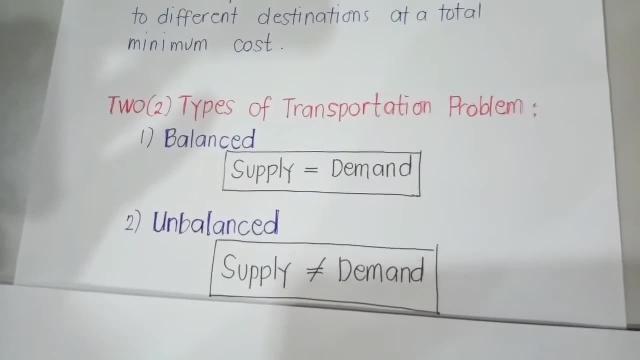 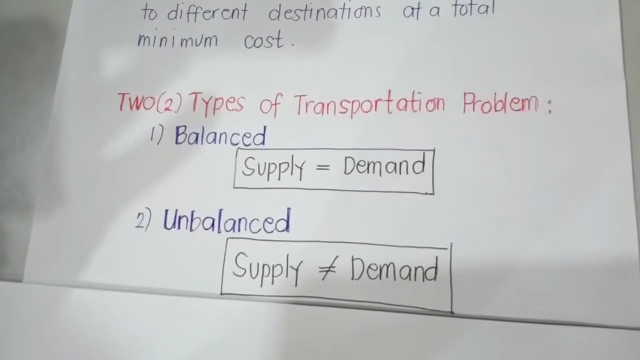 this is where the total supply equals your total demand And, on the other hand, unbalanced is where supply is not equal to a total demand. And so, for this matter, in order for us to better understand the difference between the two, let me present to you an example. So this is how. 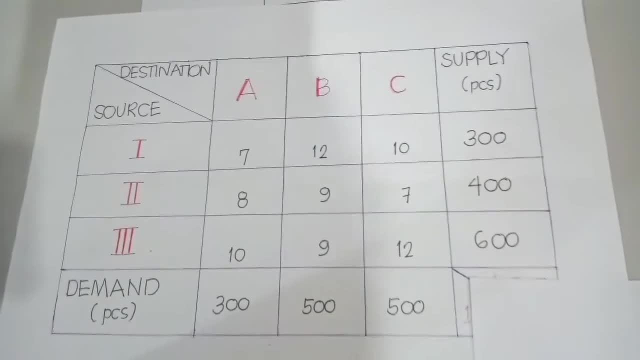 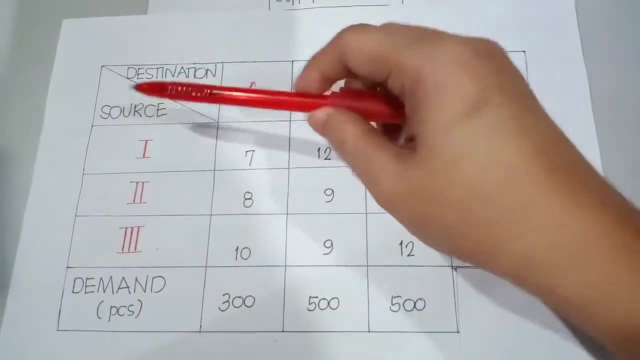 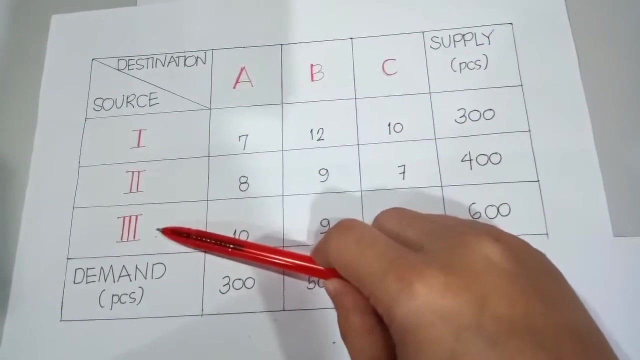 our example looks like Now. as you can see on the tabulation presented, it is composed of five columns. right, We have your source column and, in regards to your source, you have source one, two and three respectively, And for the second, third and fourth columns. 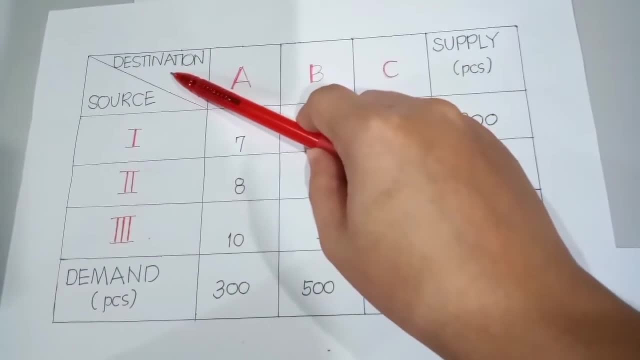 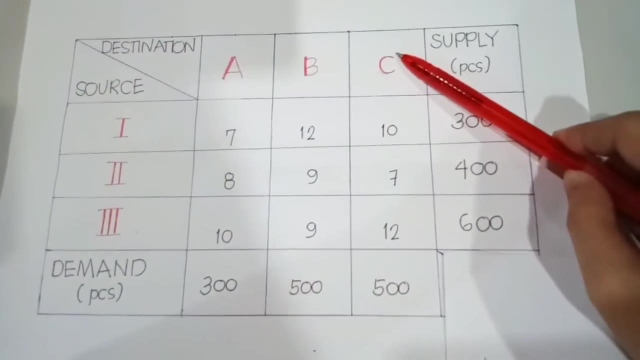 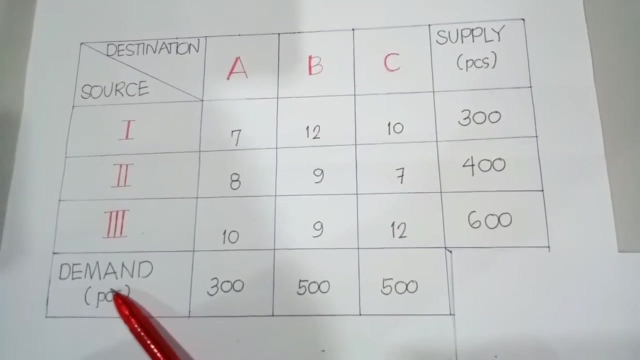 these are your destination columns, And your destination is denoted as point A, point B and point C respectively, And for the last column, you have your supply column in pieces, And for the last row, you have your demand row okay, in pieces as well. And 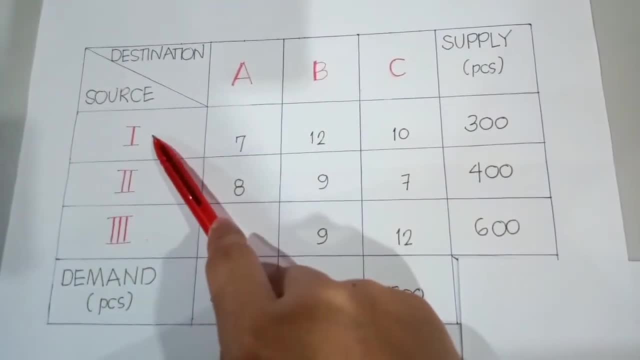 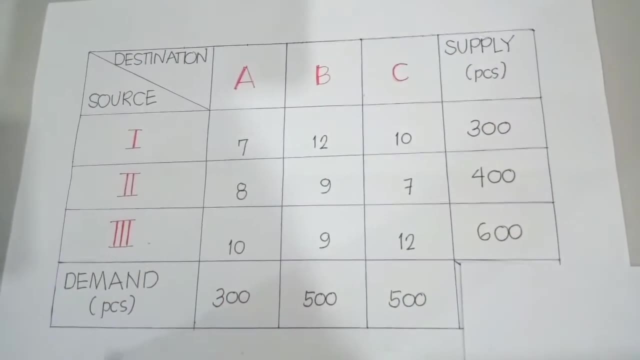 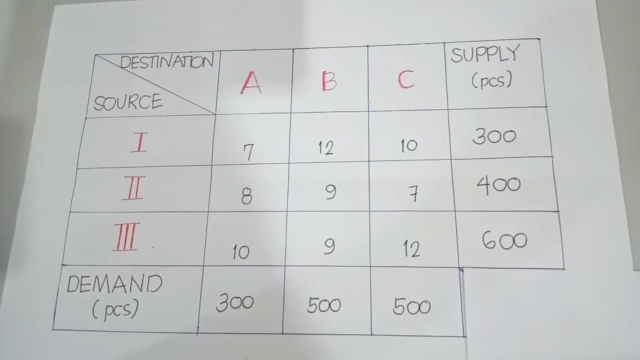 as you can notice, with respect to your source, each source has some supply and each destination has some demand. Now, in order for us to determine if this problem is a balanced or unbalanced problem, let us try to evaluate if we come up with 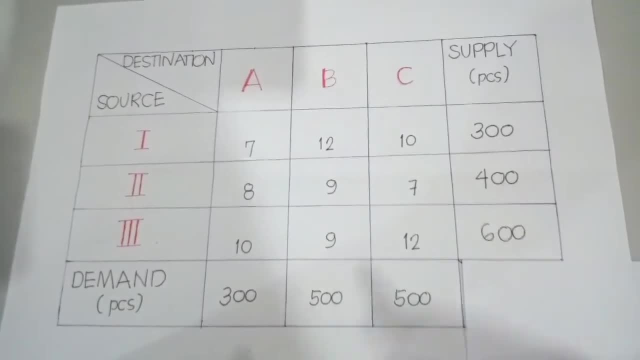 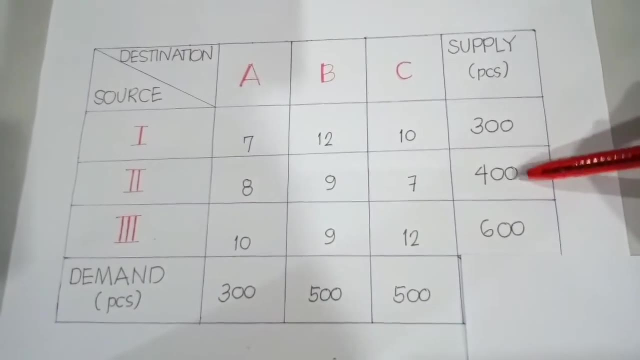 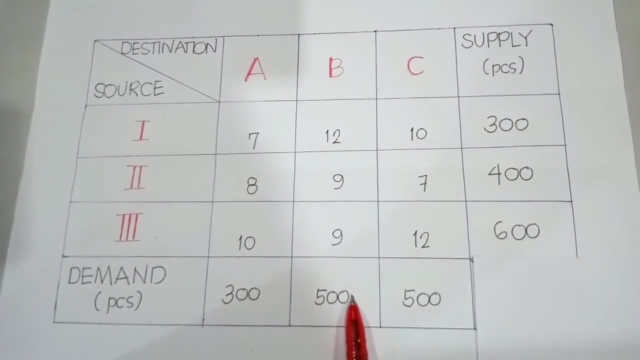 a similar amount of your supply and demand. Now, in terms of your supply, you have a total of 300 pieces, 400 pieces and 600 pieces respectively, And for your demand, that's 300,, 500, and 500. 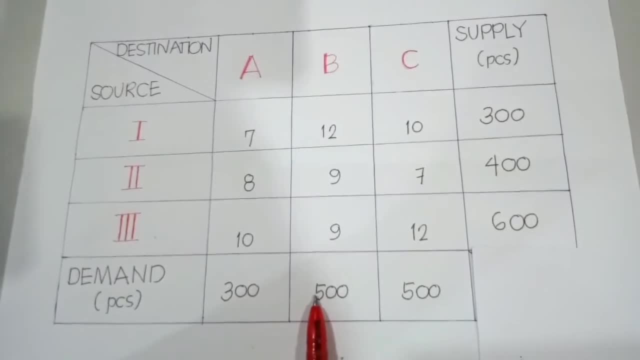 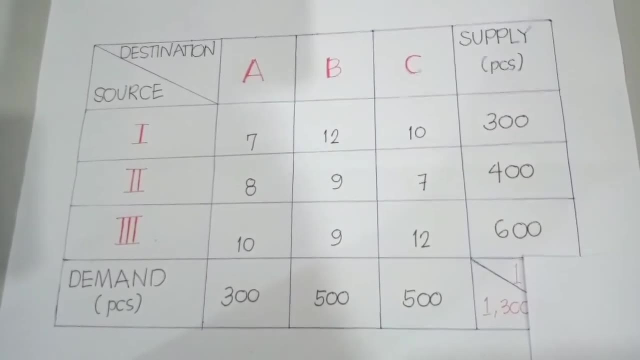 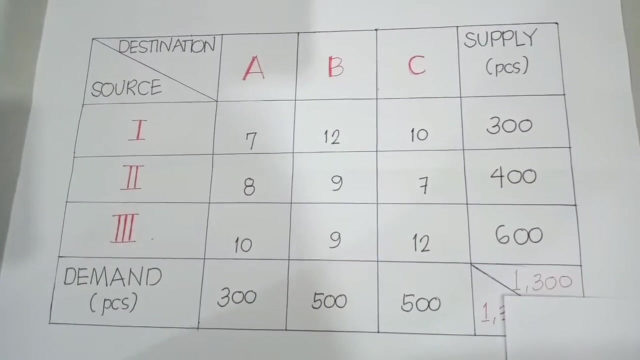 So 500, 500,, that's 1,000, plus 300,, that's 1,300 pieces. And for your supply you have 300 plus 400,, that's 700, plus 600,, you also have 1,300.. 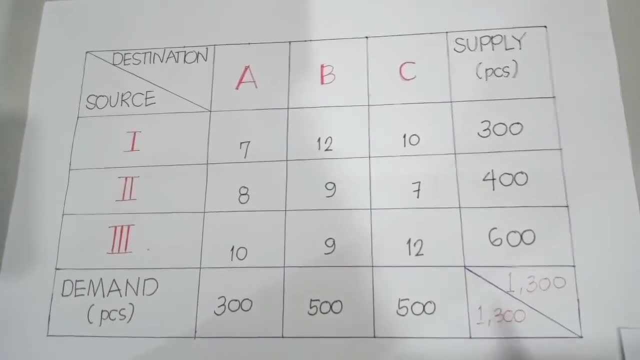 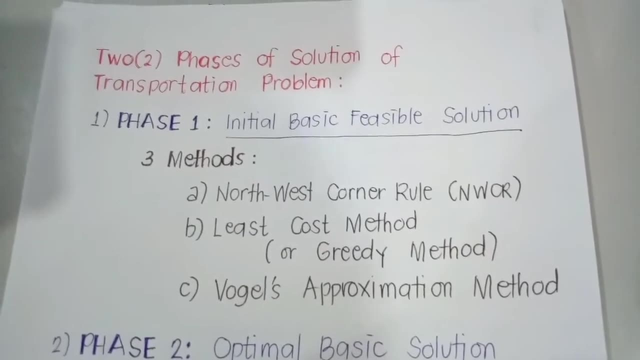 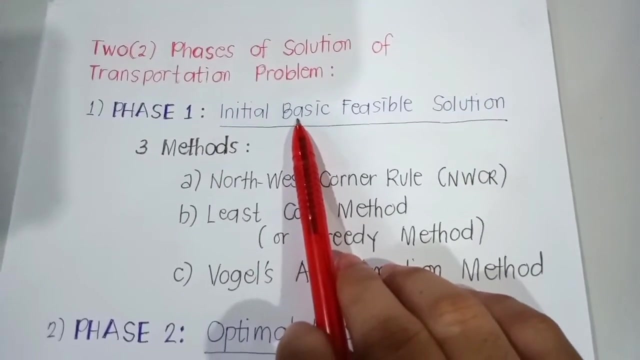 And therefore this example is an example of a balanced transportation problem. There are two phases in solving transportation problem. First we have phase one. Phase one is our initial basic feasible solution And phase two is our optimal basic solution For phase one. 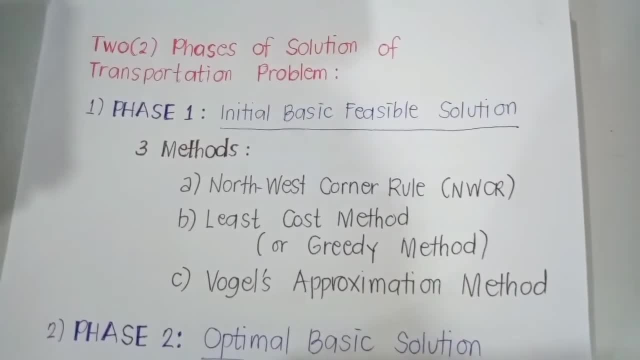 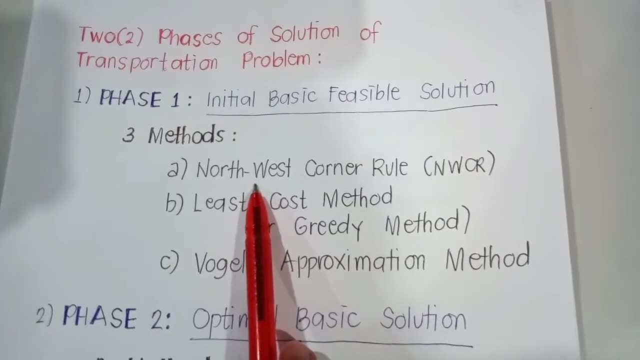 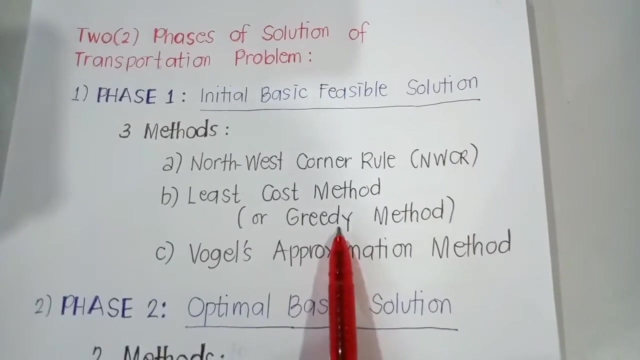 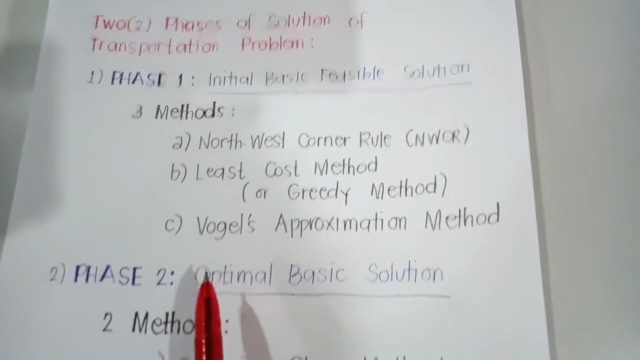 there are three methods that are normally used in establishing the initial basic feasible solution. We have the Northwest Corner Rule method, or NWCR. Second is the least cost method, or also known as the greedy method, And lastly we have Vogel's approximation method, or the VAMS method, And in phase two, 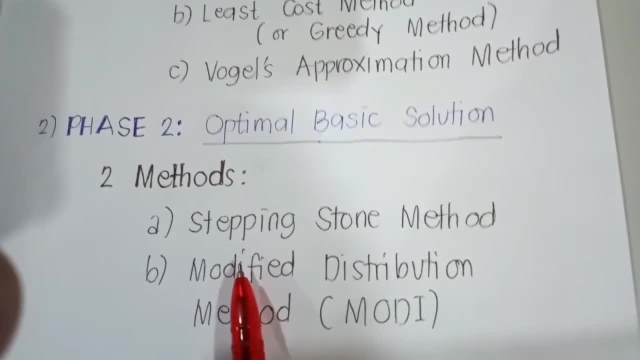 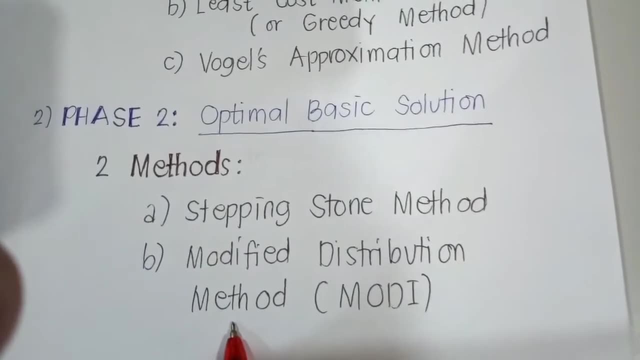 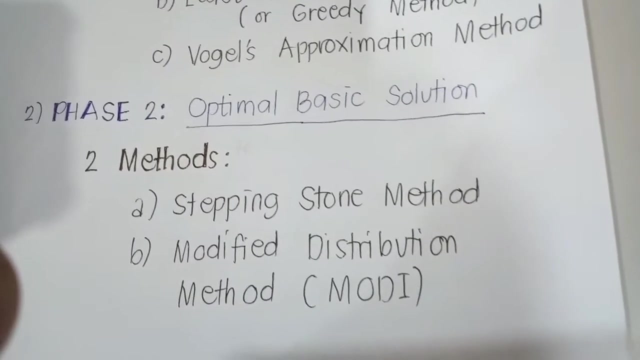 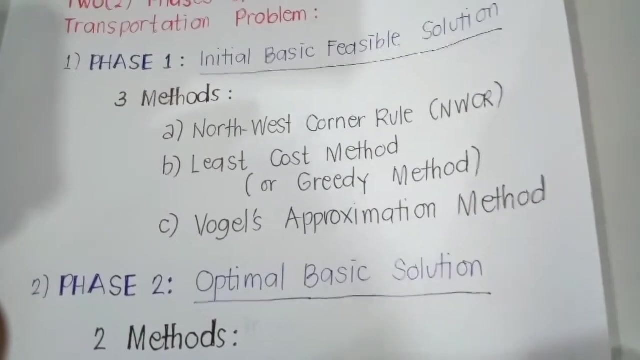 the optimal basic solution. there are two methods in establishing phase two. First, we have stepping stone method, And second is modified distribution method, or MODI. Now, this can be best explained and understood by giving you practical examples, And so, for this matter, let me start by discussing the first. 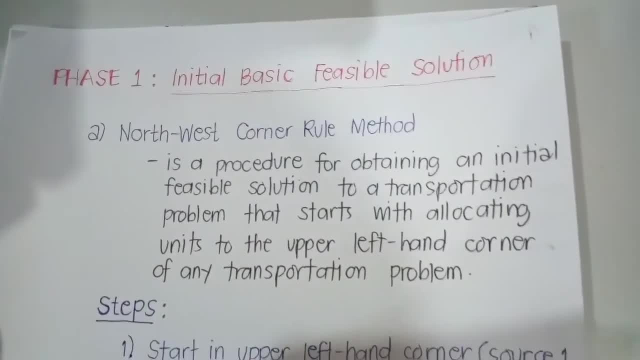 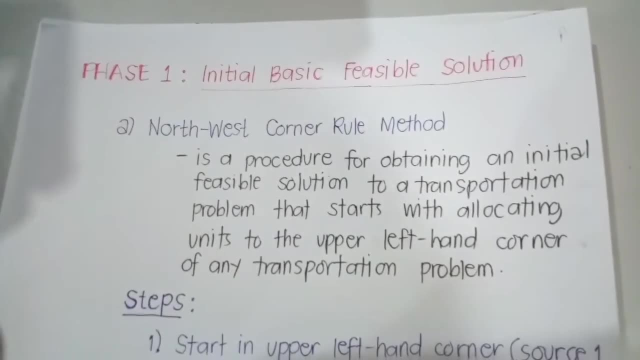 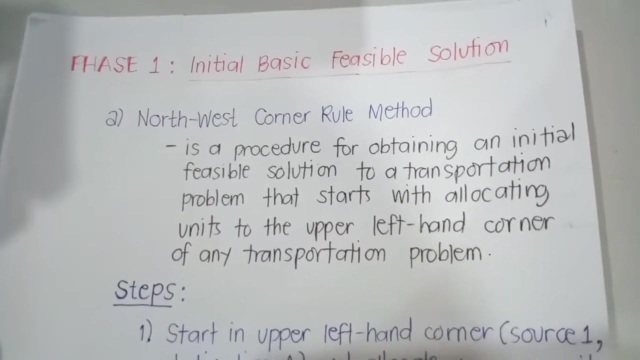 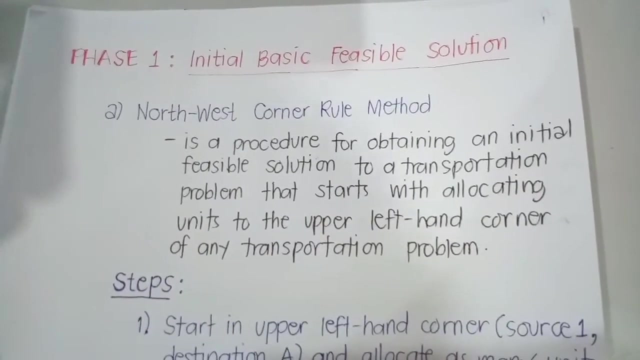 method, And the first method is what we call the Northwest Corner Rule method. Now, what is meant by this method? When we say Northwest Corner Rule method, it's a procedure for obtaining an initial feasible solution to a transportation problem that starts with allocating units to upper left-hand corner of any transportation problem. In other words, 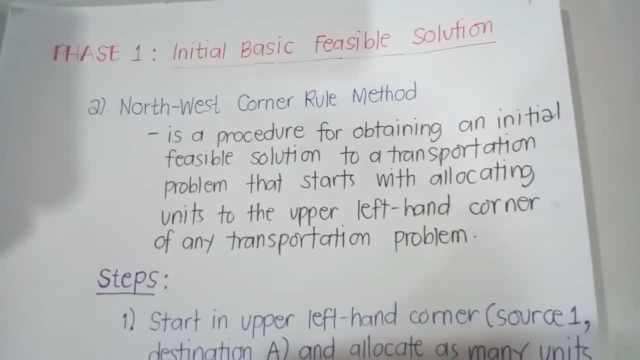 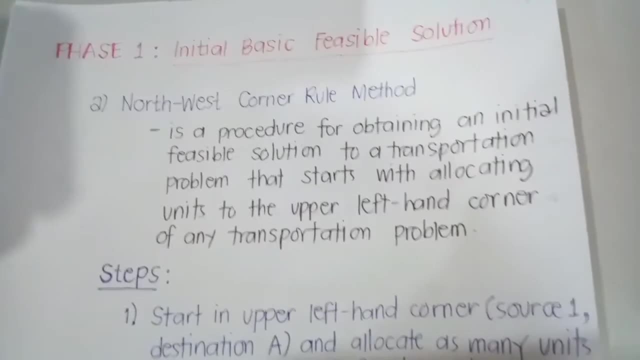 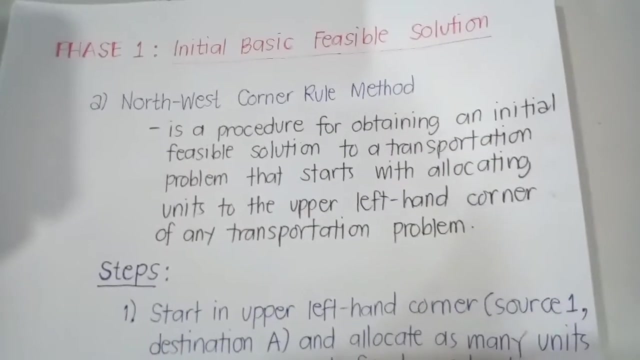 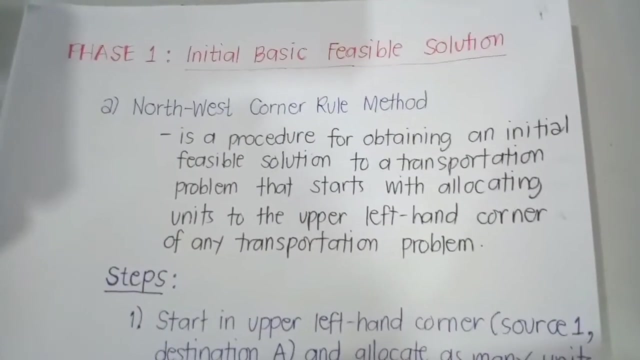 this is a method adapted to compute the initial feasible solutions of the transportation problem, And what's interesting about it is that the main northwest corner is given this method because the basic variables are selected from the extreme left corner, And so if we are given an example applying Northwest Corner Rule method, 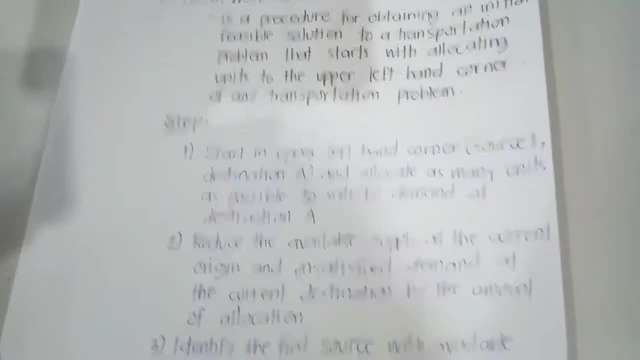 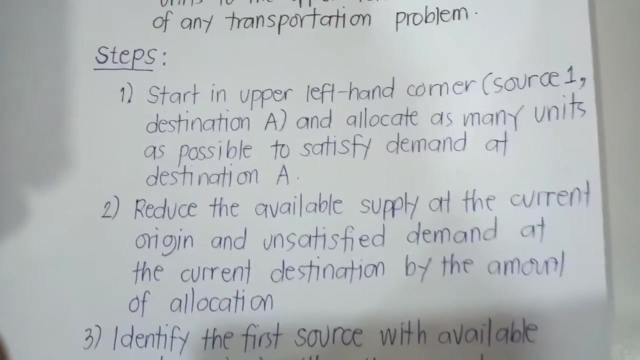 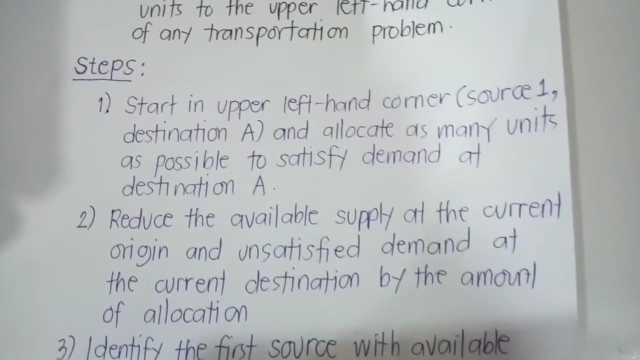 this can be done by strictly following the six steps, And these are the following six steps. First step: you have start in upper left-hand corner or source one destination A and allocate as many units as possible to satisfy demand at destination A And for step two. 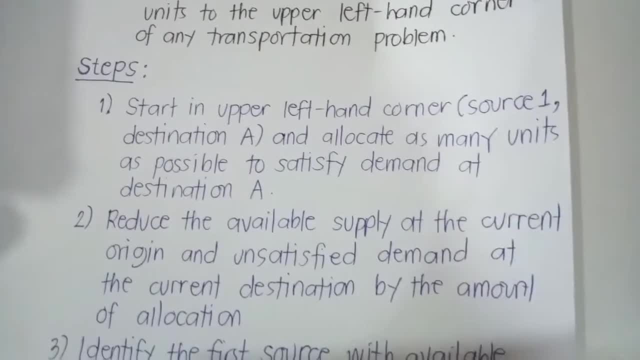 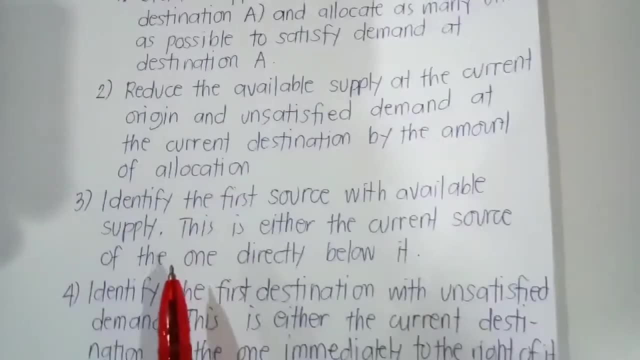 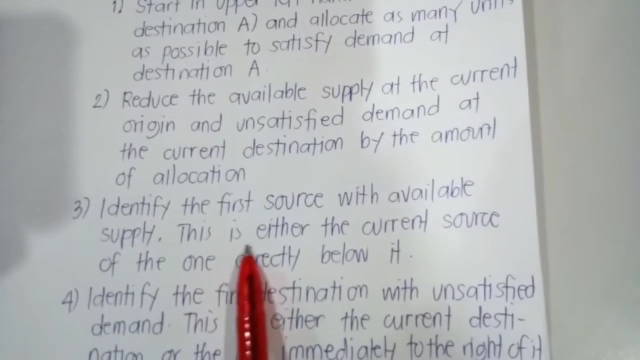 reduce the available supply at the current origin and unsatisfied demand at the current destination by the amount of allocation. For step number three, you need to identify the first source with available supply. This is either the current source of the one directly below it. 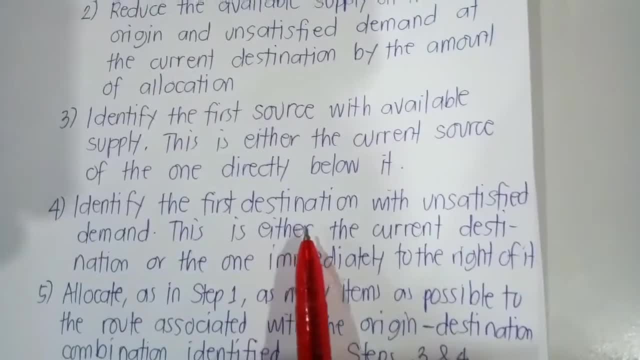 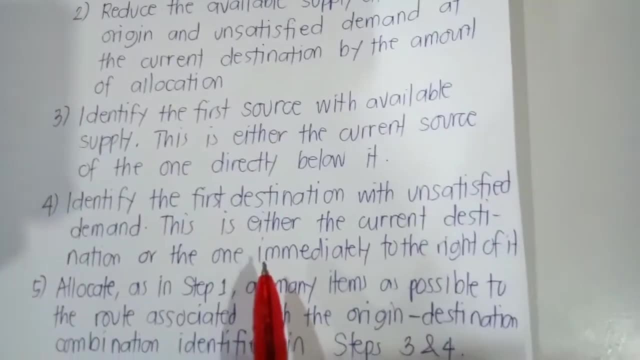 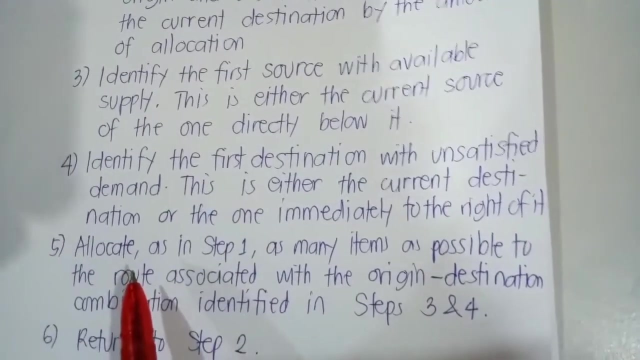 And step number four, we need to identify the first destination with unsatisfied demand. This is either the current destination or the one immediately to the right of it. And number five step: allocate, as in step number one, as many items as possible to the route. 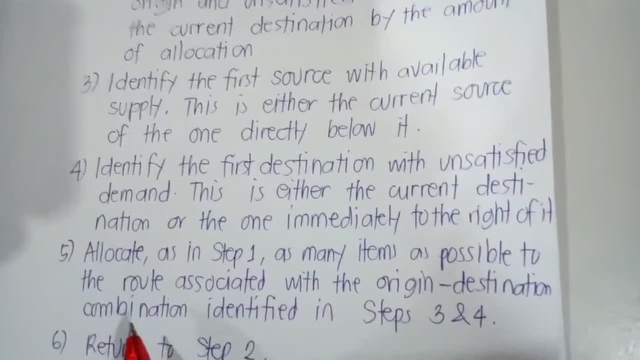 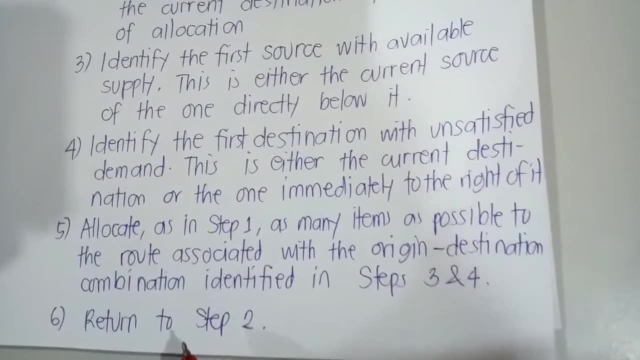 associated with the first destination. And for step four, you need to identify the first destination associated with the origin-destination combination identified in steps numbers three and four. And last step is to return to step number two. Now, in order for these six steps to be meaningful, 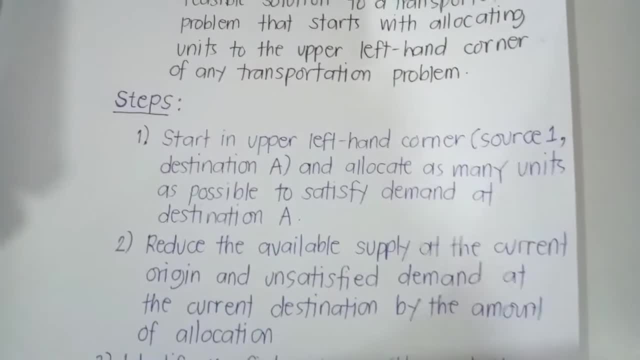 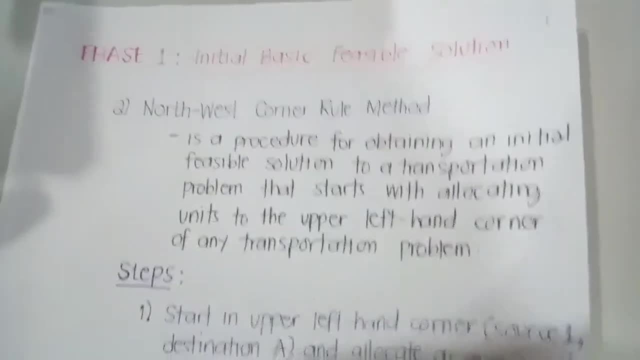 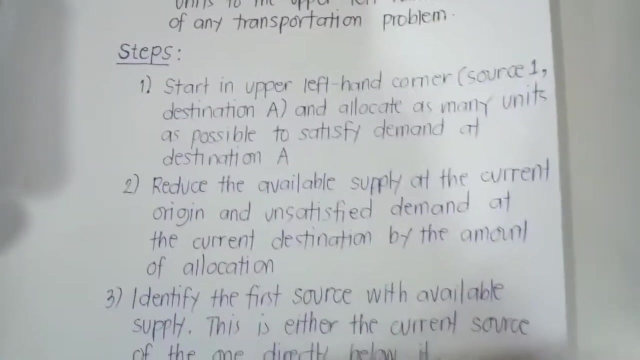 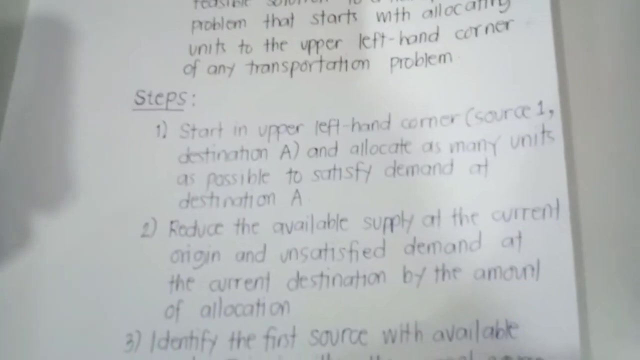 I will give you a practical example and we will try to apply the first phase, first method, which is the corner or the northwest corner rule method. Now, in order for these steps to be meaningful, I will be providing you practical examples and we will apply the first phase, first method. 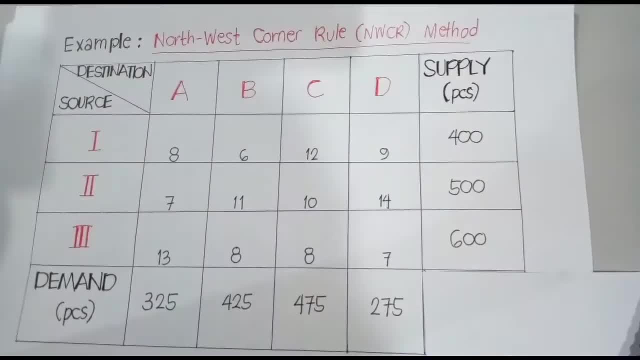 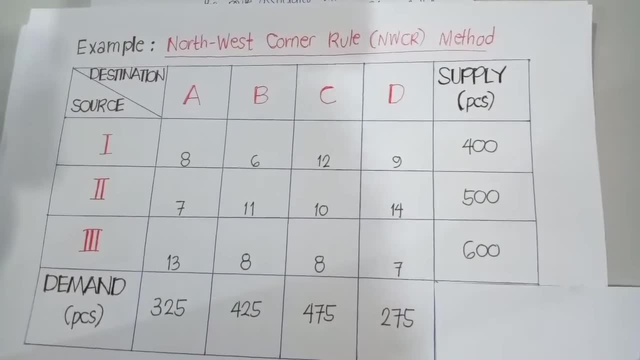 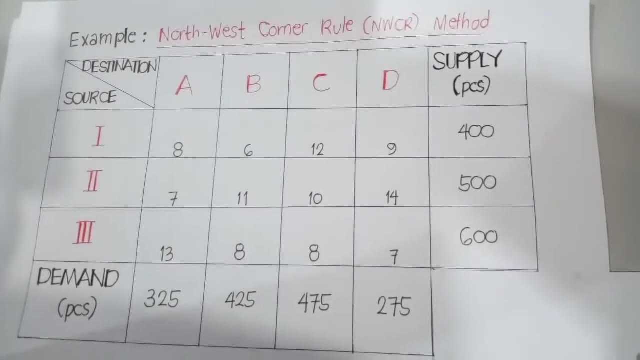 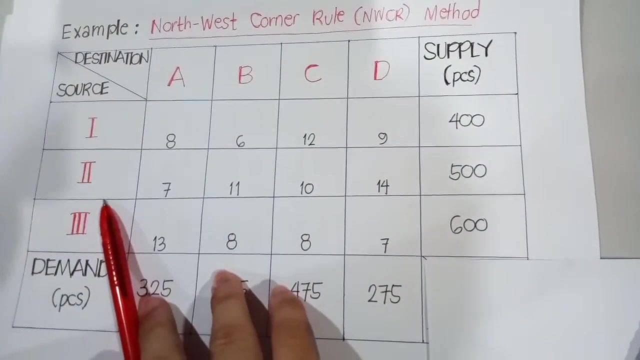 which is also known as the northwest corner rule method. As you can see, this is an example of northwest corner rule or NWCR method, And, based on the tabular presentation, there are three different available resources. You have source 1,, 2, and 3, respectively, And also there are four. 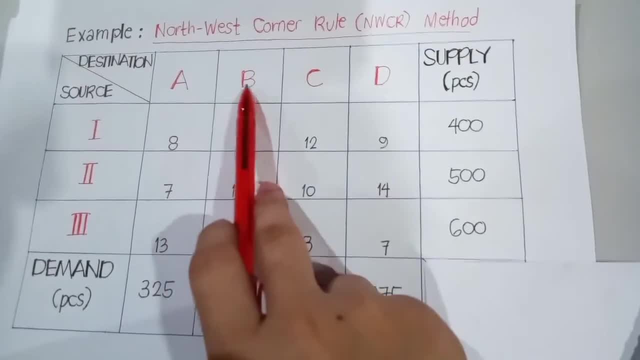 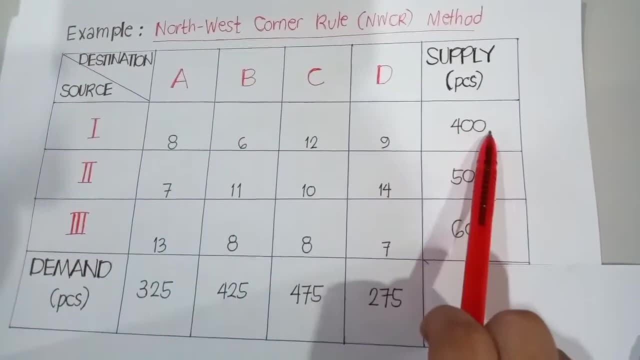 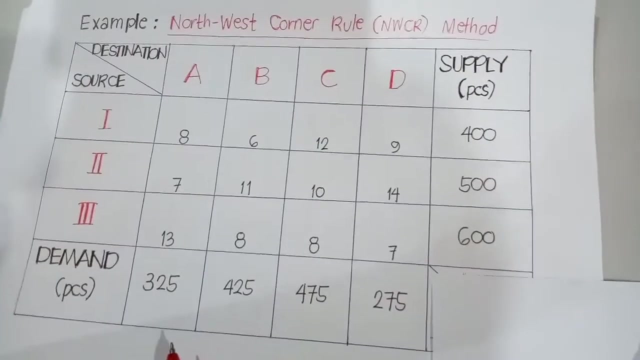 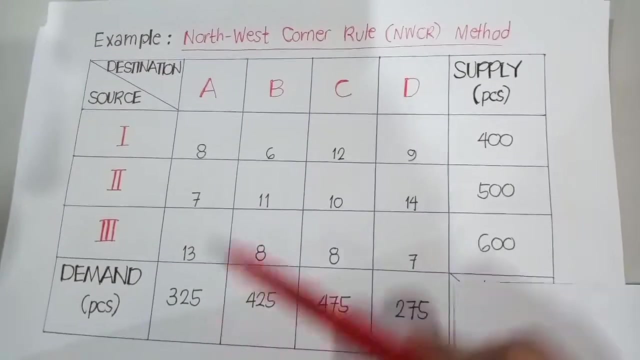 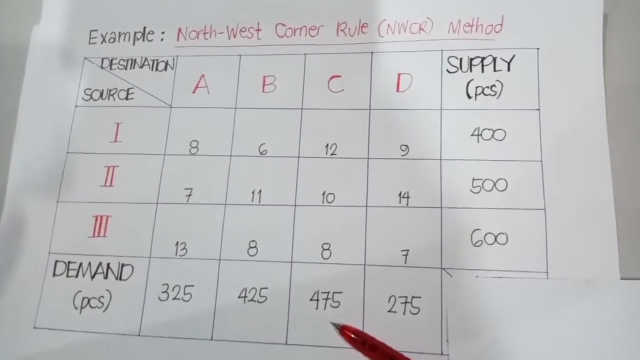 destinations denoted by points A, B, C and D as well. Now, each source has a corresponding supply And for each destination you have a corresponding amount of demand. With respect to destination A, you have a total demand of 325 pieces. For B, you have 425 pieces. For C, you have 475 pieces. 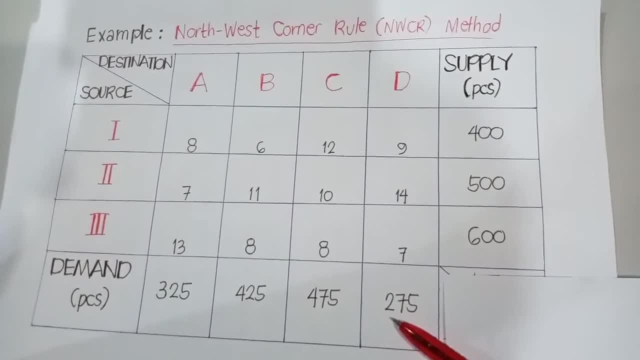 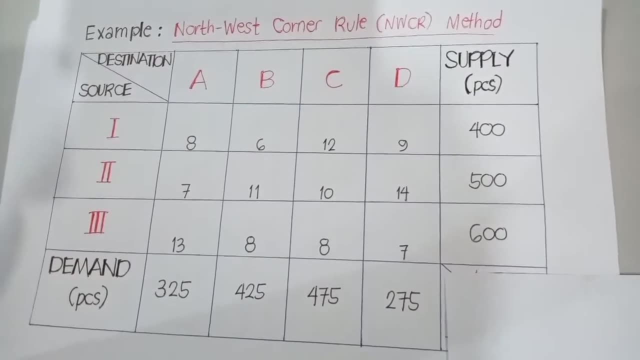 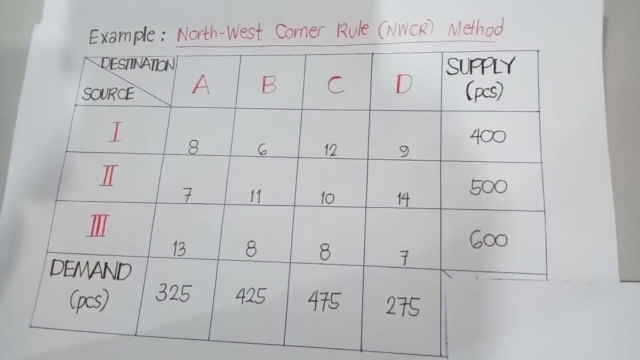 And for destination D you have a total of 275 pieces. Now, before solving the problem, we need to determine first if it is a balanced or an unbalanced type of transportation problem. Now, as discussed earlier, when we say balanced transportation problem, it means that your total supply equals your. 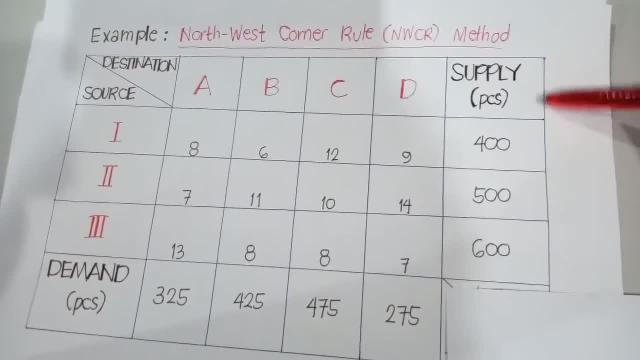 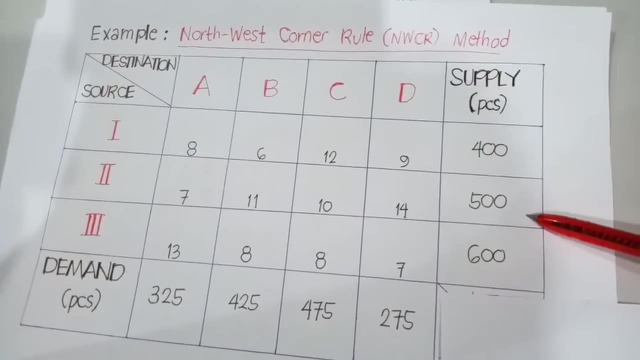 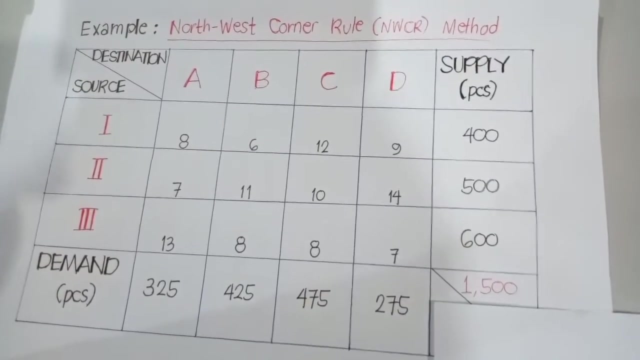 total demand Since, as you can see, your total supply with respect to source 1,, you have 400, 500 for source 2, and 600 for source 3. And the total that would be 1,500 pieces or 1,500.. 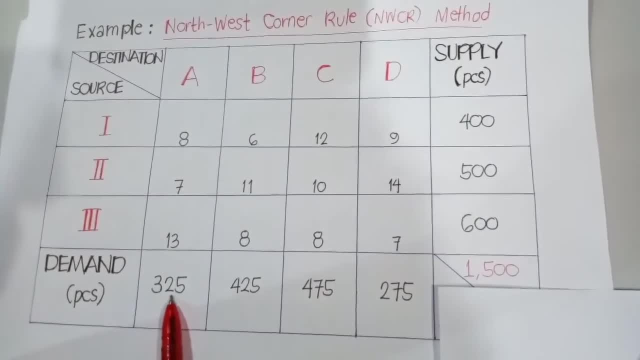 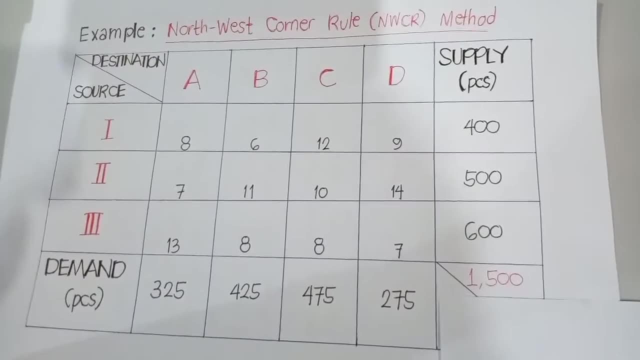 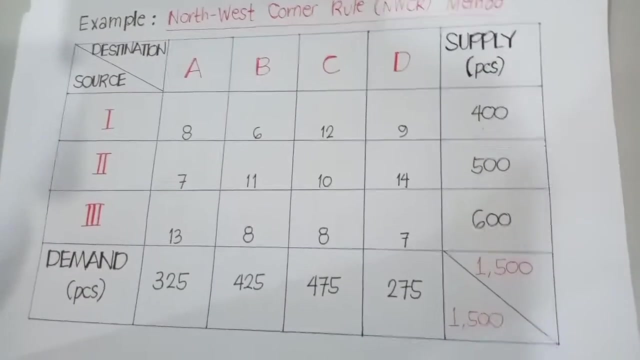 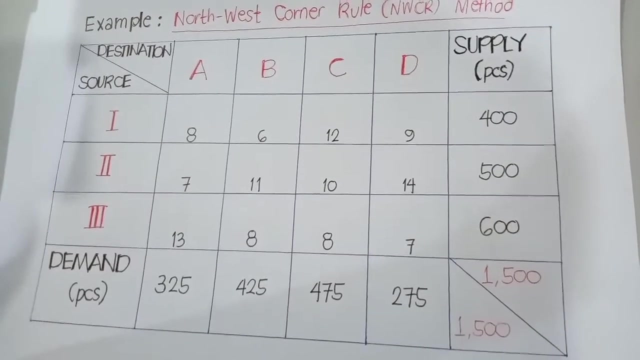 Now, in terms of demand, you have 325,, 425,, 475, and 275.. So a total of 1,500 pieces, or 1,500 pieces. Therefore, for this particular problem, it's an example of balanced transportation problem. 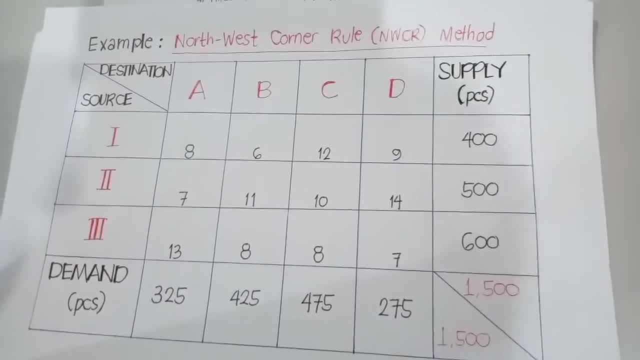 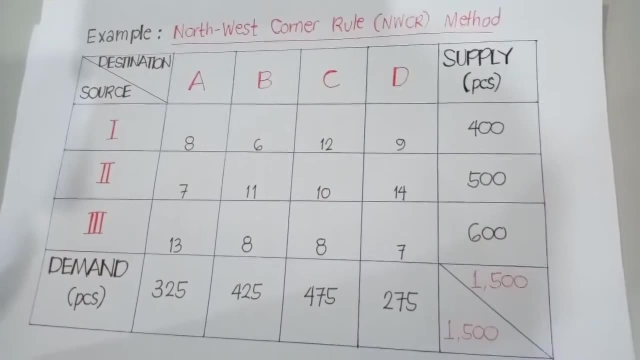 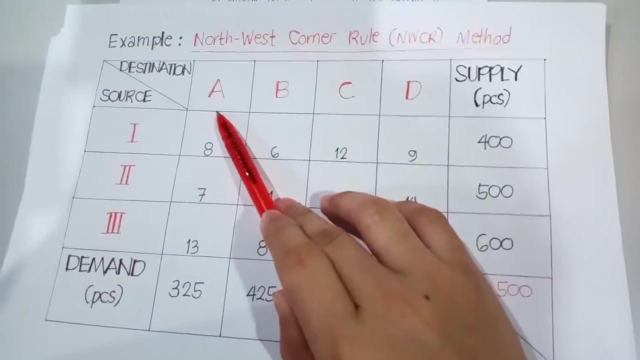 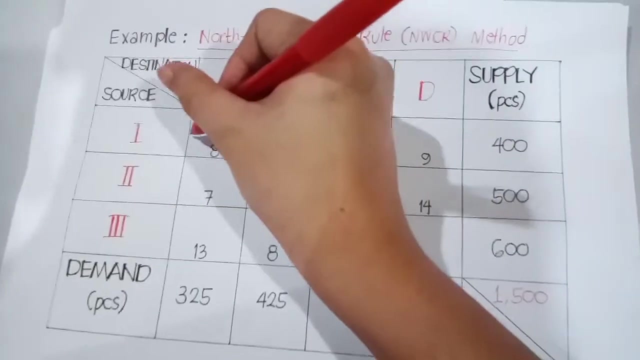 Now, do you recall why it's called the Northwest Corner Rule? Because the basic variables are first of all selected from the extreme left corner, And so we will start right here, at this corner, Because this is north, okay, and this is south, this is east and this is west. So we will start from this corner, right here. 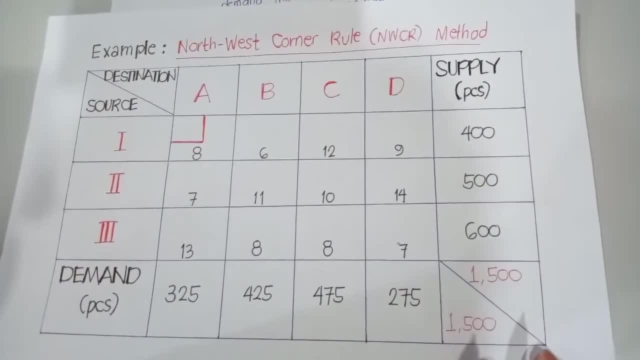 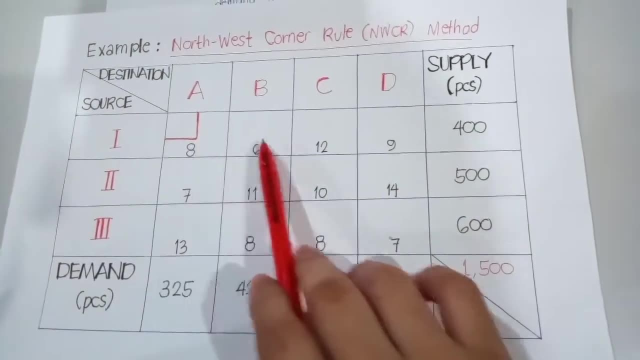 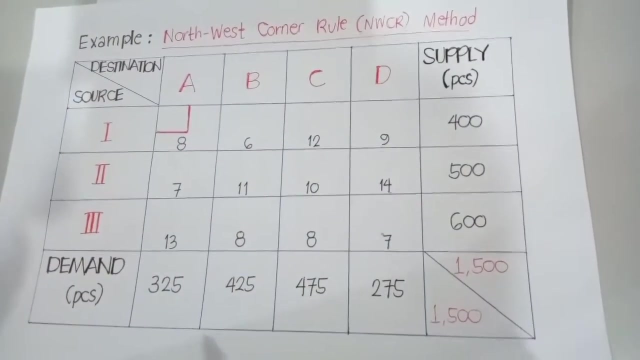 Take note that each element of this cell is considered as the transportation cost. So the elements 8,, 6,, 12,, 9,, 14,, 10,, 11,, 7, and so on and so forth, these are our transportation. 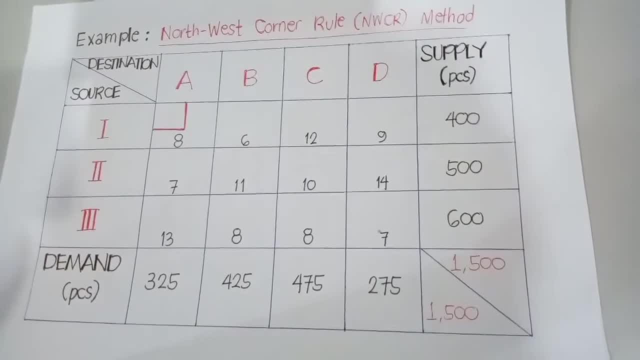 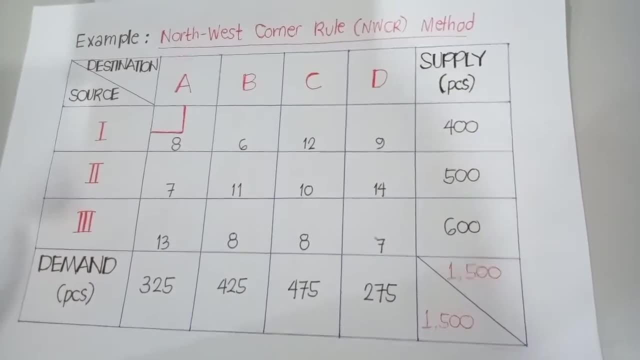 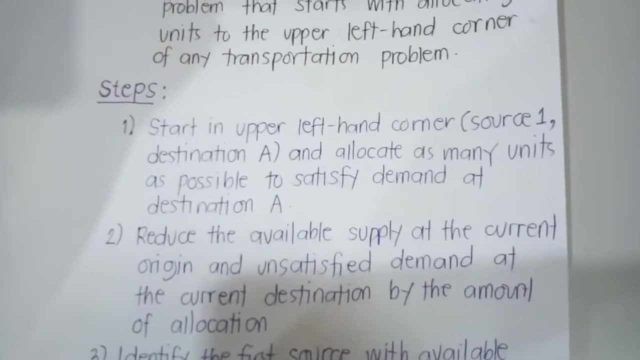 costs. So what do we do next? In order for us to be guided, we need to strictly follow the steps of Northwest Corner Rule. So what do we do next? We need to strictly follow the steps of Northwest Corner Rule. Now, what's step number one? So, as you can see, step number one says: 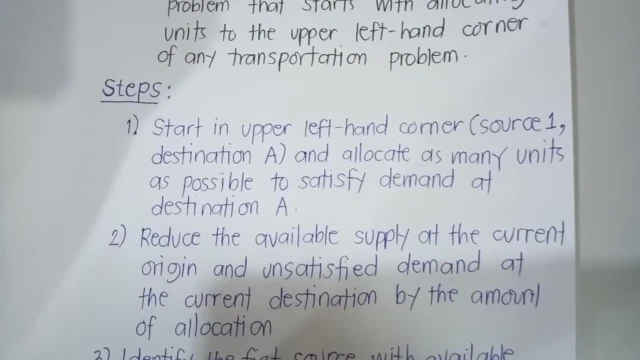 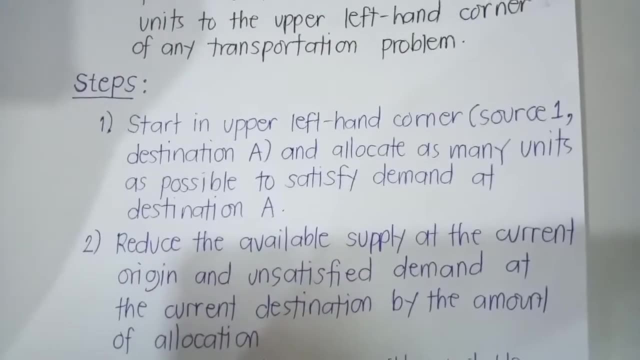 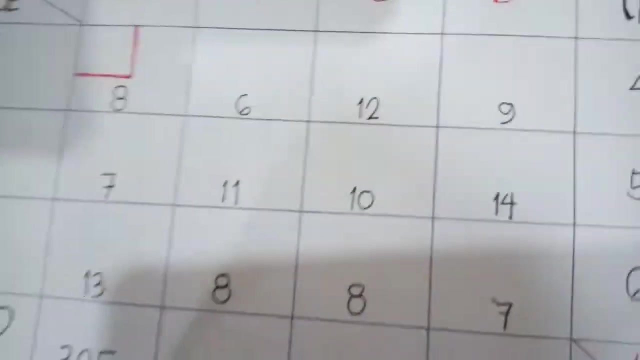 start in the upper left-hand corner. The upper left-hand corner of our cell is source 1, destination A, And we need to allocate as many units as possible to satisfy demand at destination A. So, as you can see, going back to our problem, this is our number one, So we need to allocate. 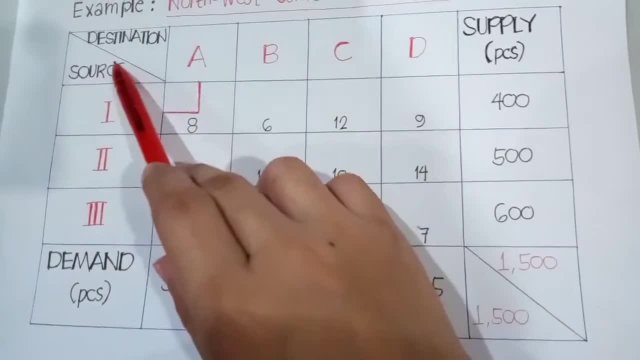 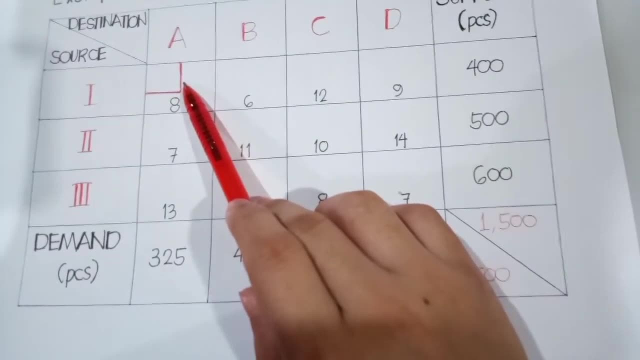 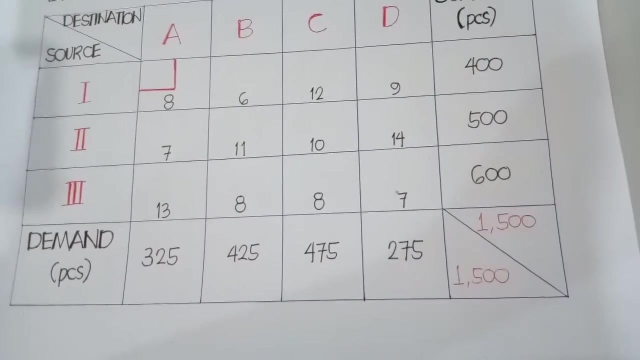 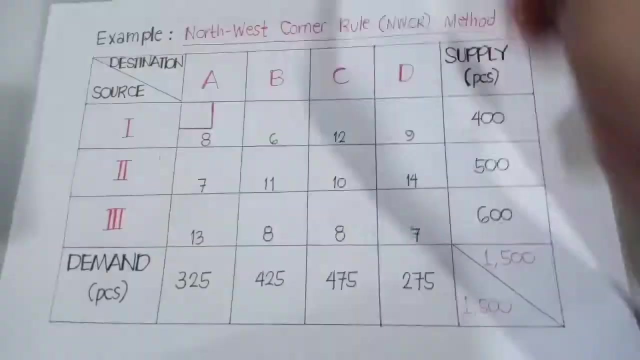 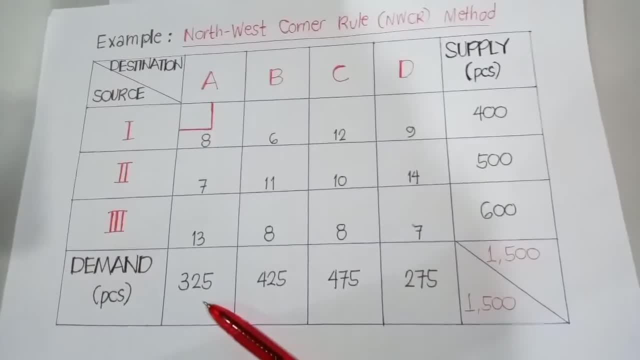 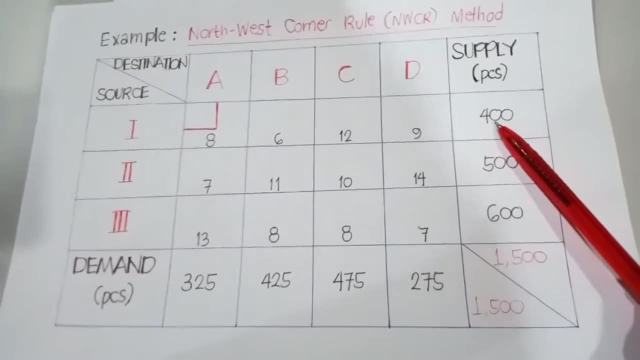 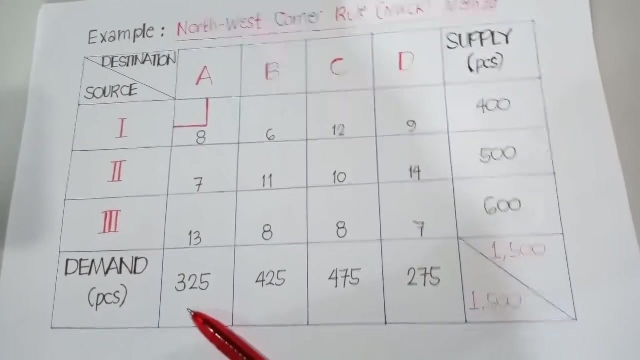 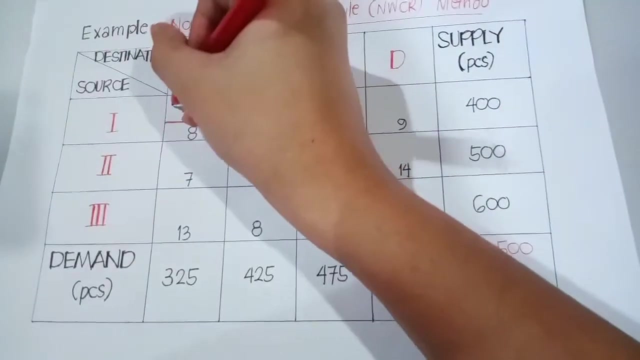 cell. your demand is 325 pieces and your supply is 400 pieces. now which one has the lesser value? so apparently, that will be your demand. it only has 325 pieces and so, for this matter, this will be the amount that we will be allocating in this cell. so we will allocate 325 pieces. so that is step. 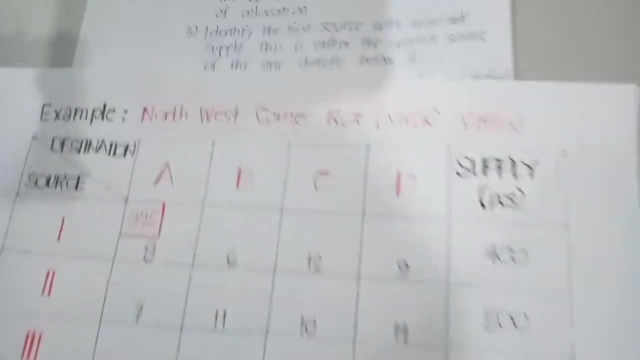 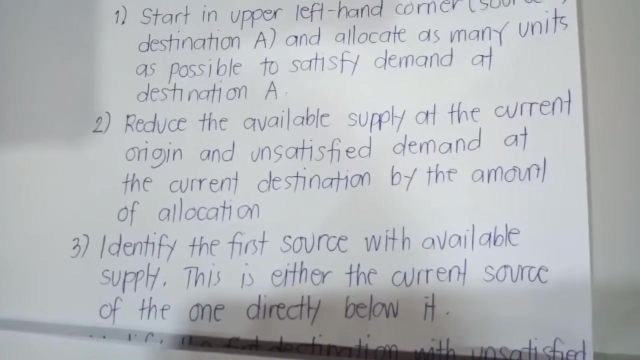 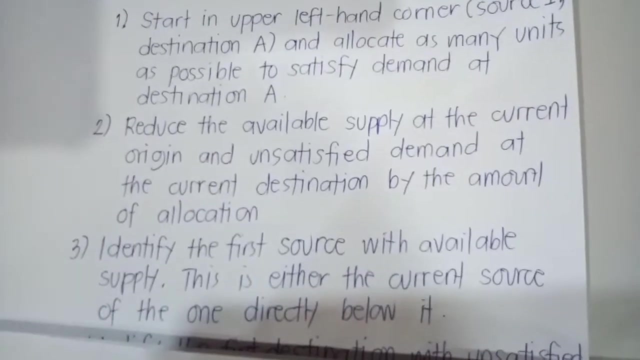 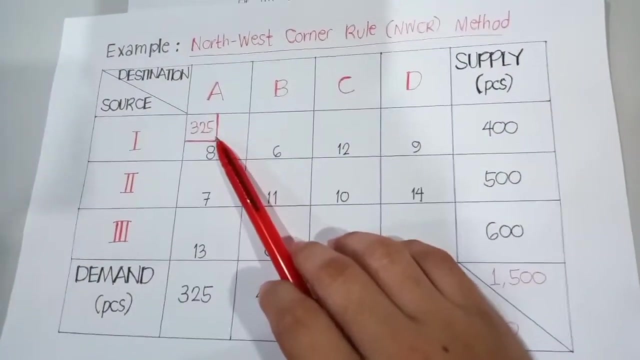 number one. now let's move on to step number two. now. step number two states reduce the available supply at the current origin and unsatisfied demand at the current destination by the amount of allocation. now going back to our problem, as you can see, we have already allocated um a resource here, amounting 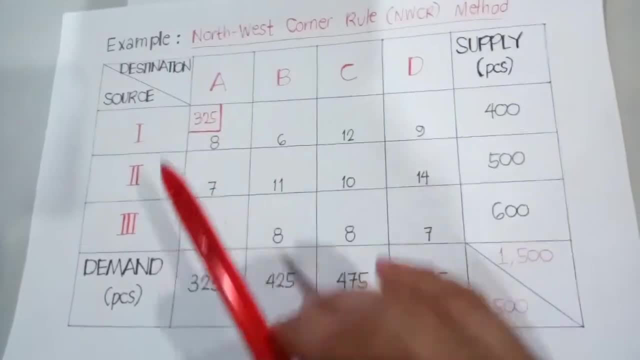 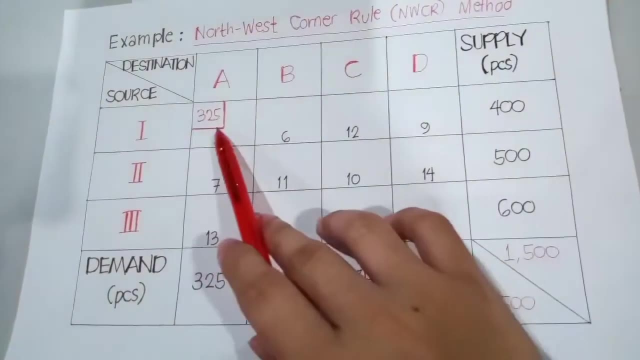 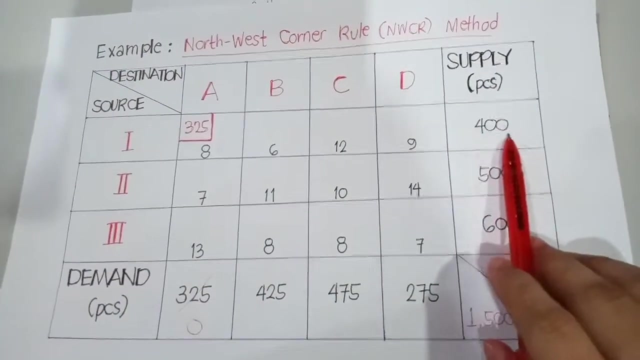 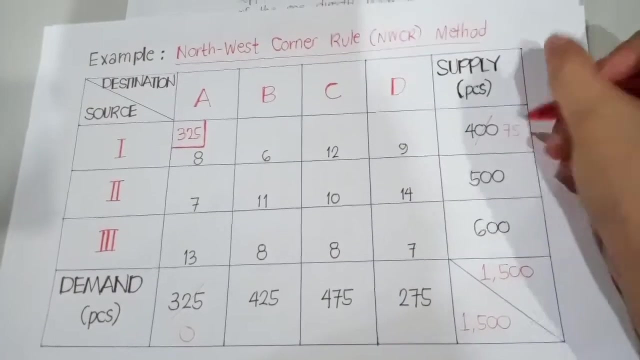 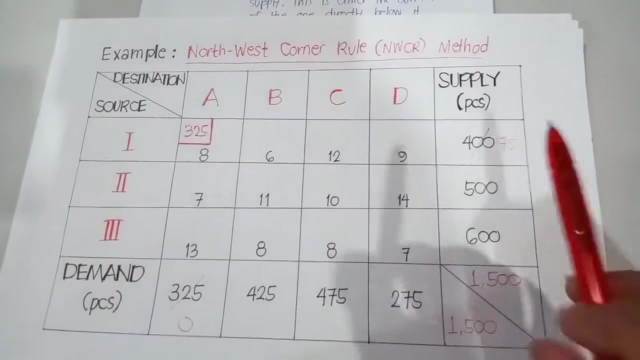 to 325 pieces and therefore our demand, 325, is already satisfied. so 325 minus 325, that becomes zero right, and 400 minus 325, so that becomes 75 pieces. so that's step number two. what we did, we reduced the amount of our remaining supply. 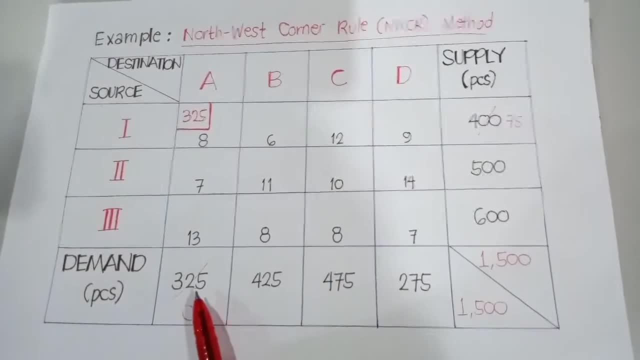 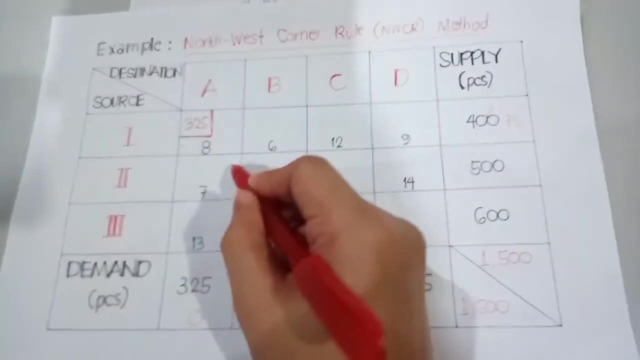 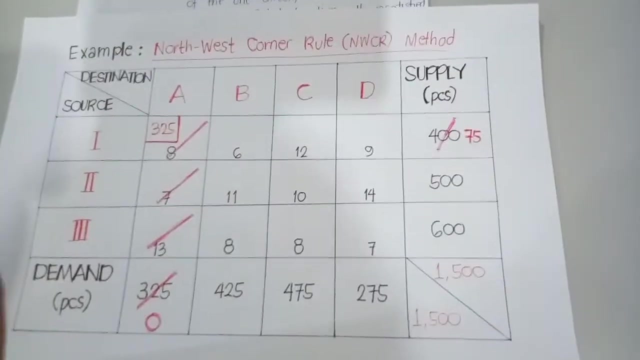 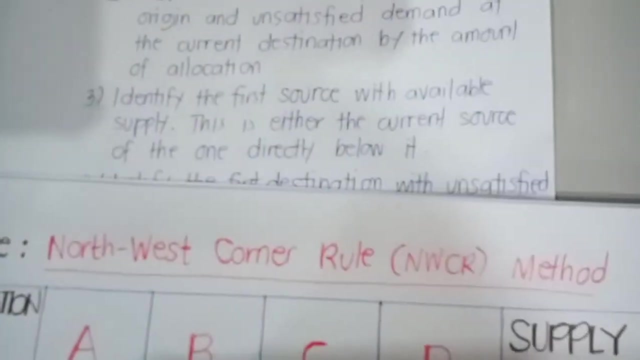 and our demand. now, as you can see, since this is already exhausted, that means to say that we need to cancel out or mark out the entire column a. okay, this will be marked out already. so that is step number two. and moving on to step number three, step number three states: we need to. 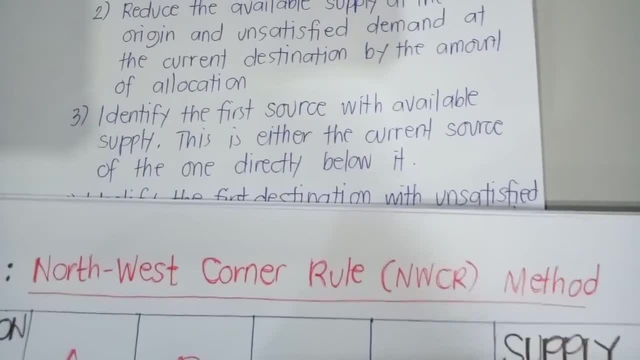 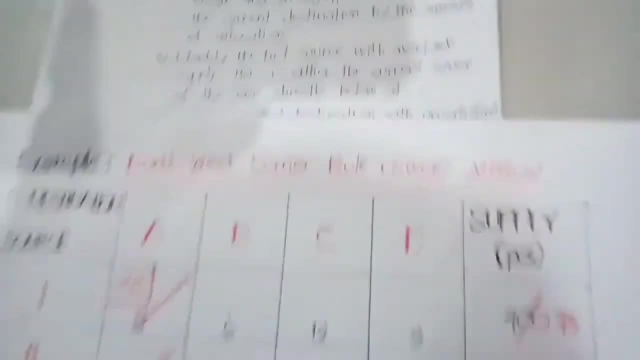 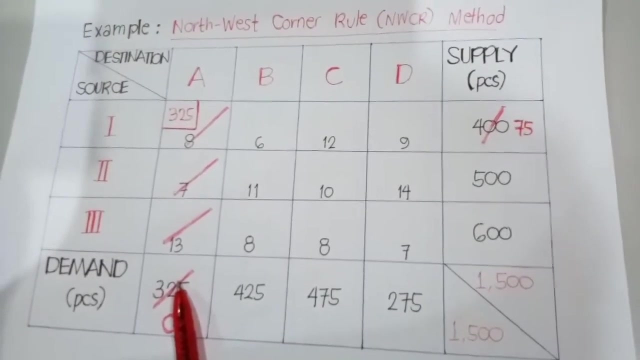 identify the first source with available supply. this is either the current source of the one or the one directly below it. now, going back to our problem: since we already canceled out the entire column a, we are now left with destination columns with points B, C and Z. 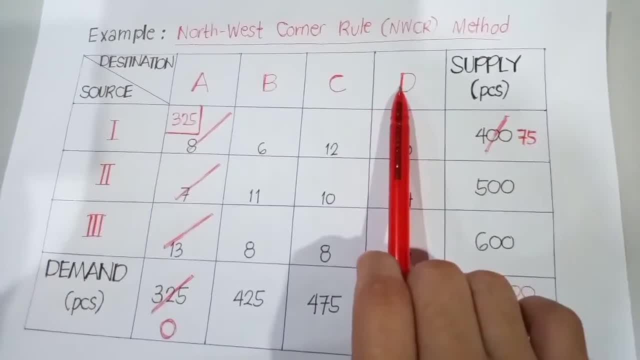 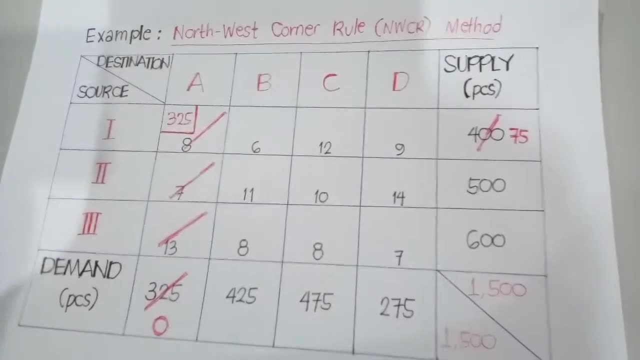 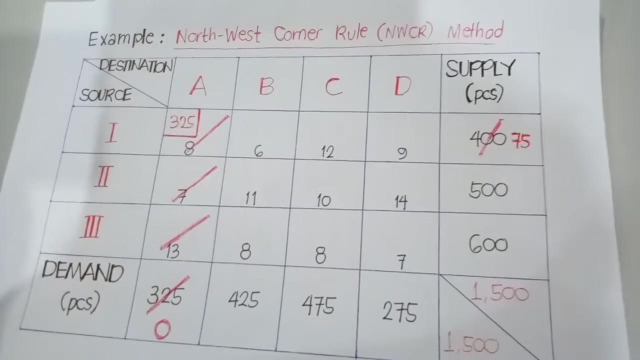 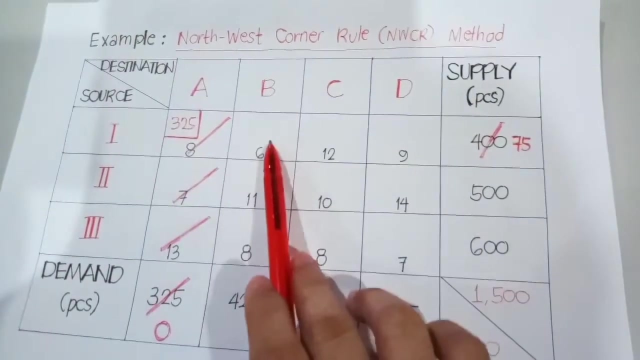 c and d as well, and including the supply column. okay, so we have b, c, d and the supply columns left, and so we need to find out the extreme northwest corner of our remaining columns, and in this case, our northwest corner is the source one and destination b, which is 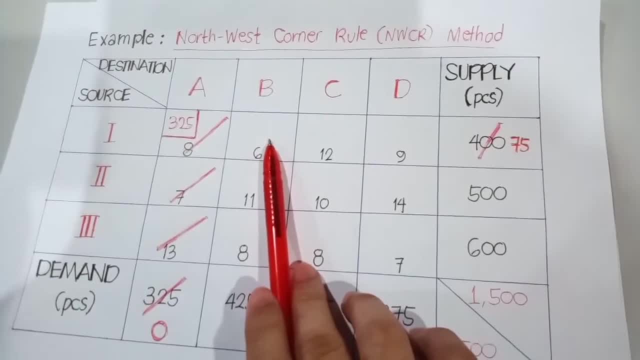 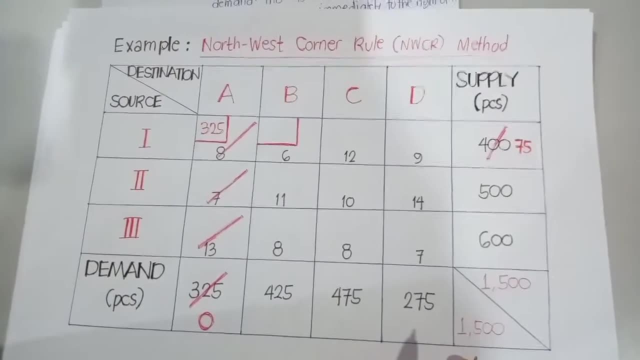 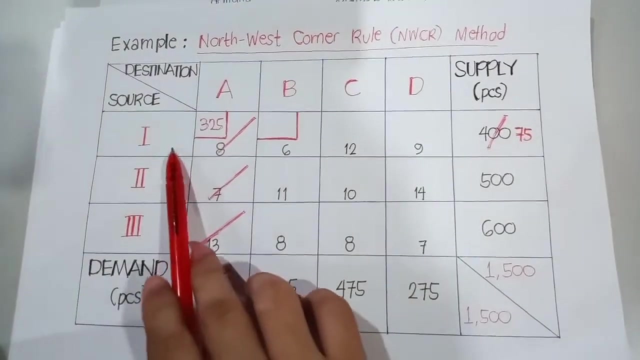 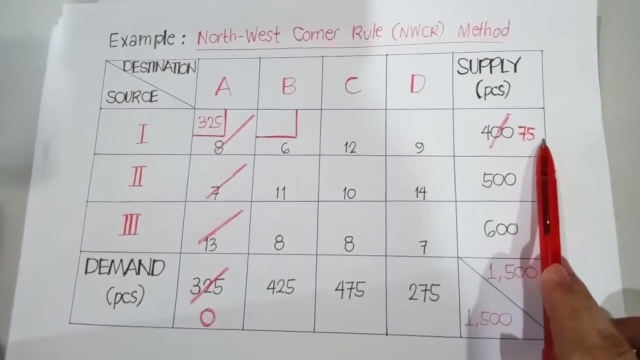 this one. so we will be doing our allocation in this cell, since in step number three we need to identify the first source with available supply. as you can notice, each source still has available supply right. for source one, we still have remaining of 75 pieces. for source two, we have 500 and for source three, we have 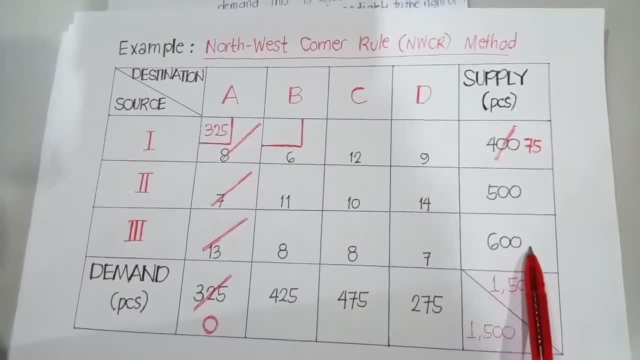 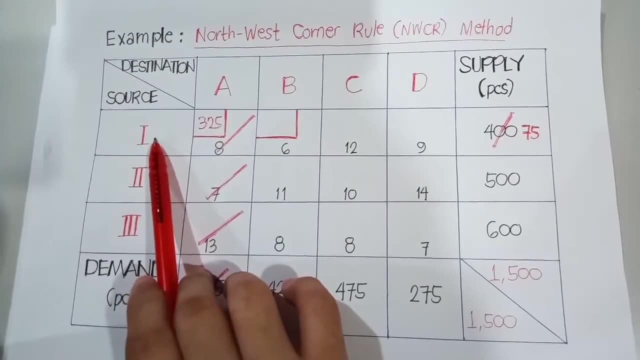 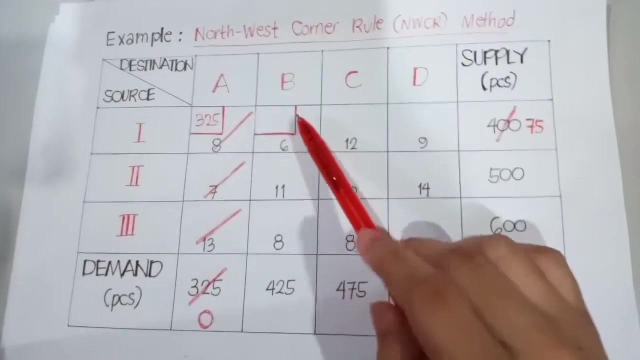 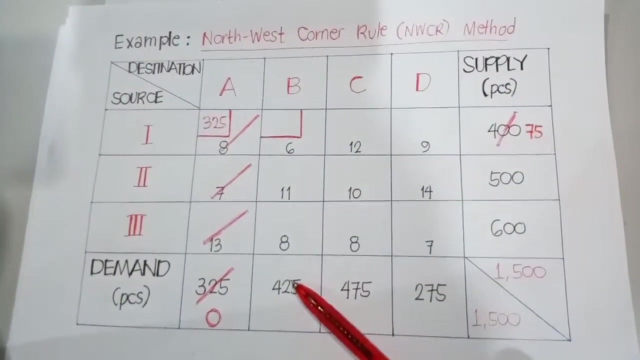 600. but it is very clear that we need to identify the first source with available supply, since our source one is the first source, then the remaining supply is 75 and since we will be doing our allocation in this particular cell, so we need to match the quantity of our demand versus the 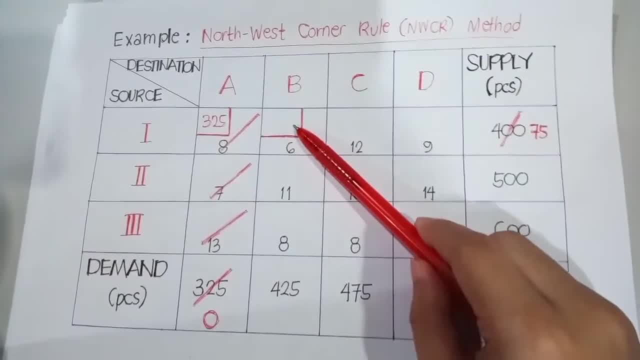 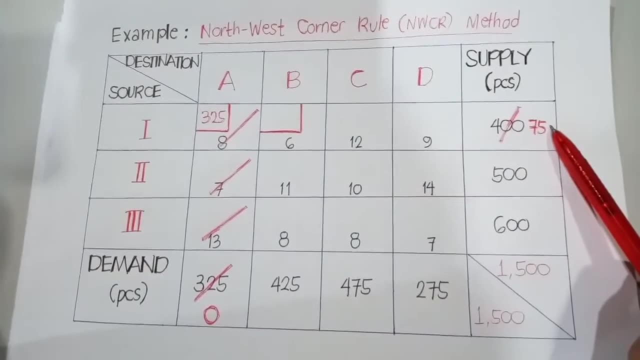 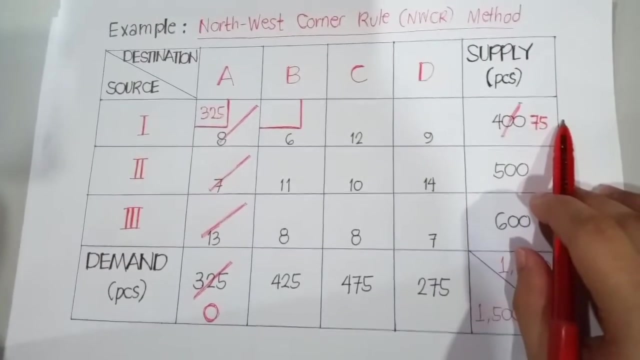 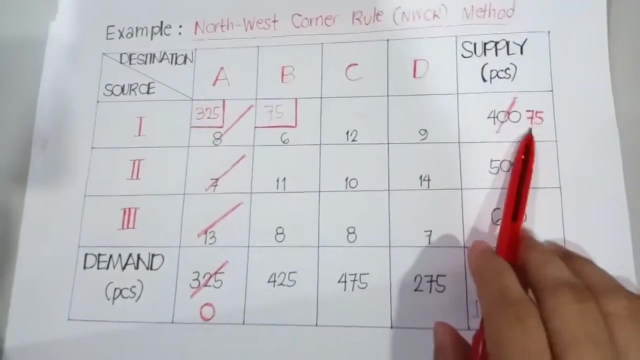 quantity of our supply now with respect to this cell. our total demand is 425 pieces and our total supply is 75 pieces. so which has the lesser value? we have the supply 75 pieces, and so for this matter, we will be allocating 75 pieces right here, so 75. 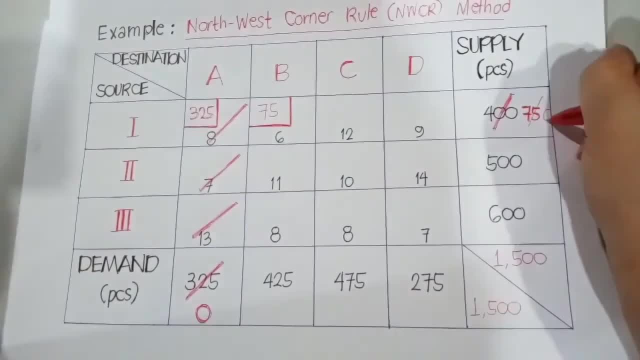 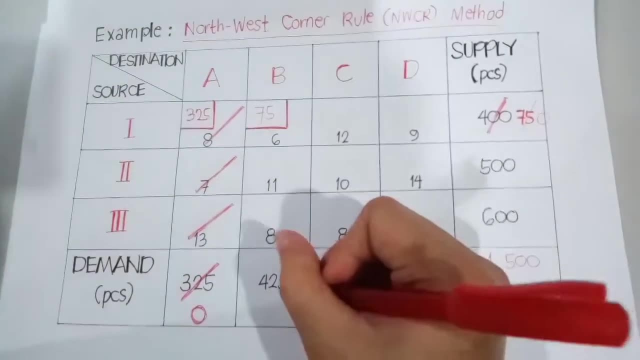 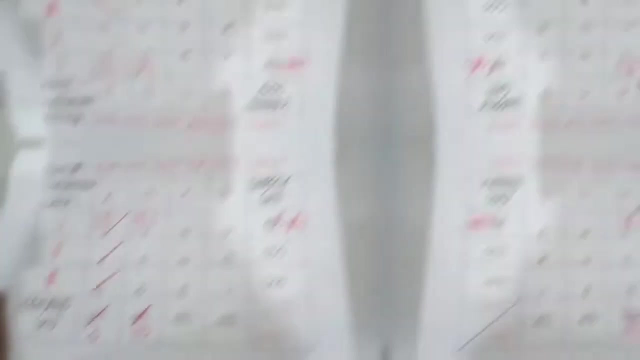 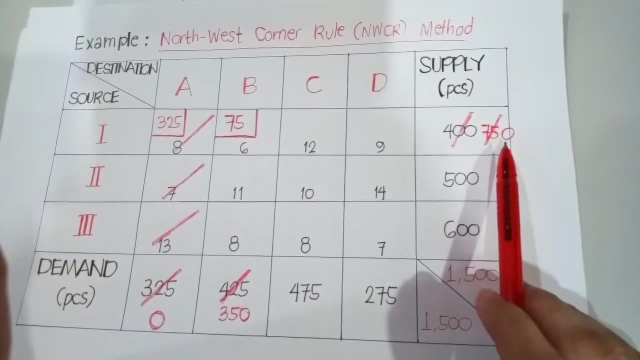 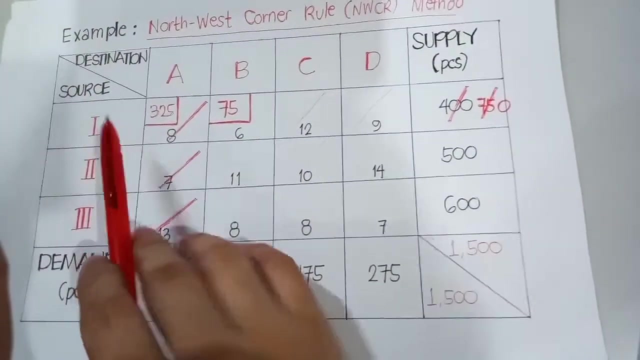 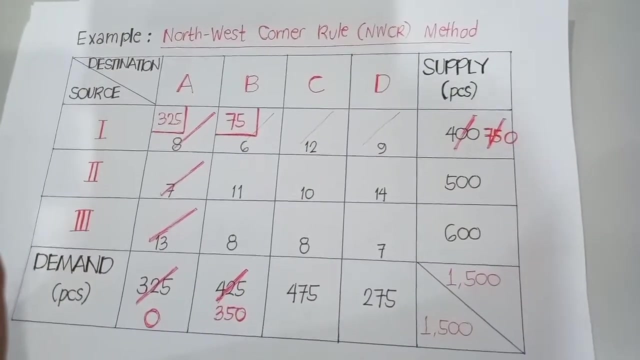 minus 75, this becomes zero, and 425 minus 75, so that becomes 350 pieces. okay, that's step number three. since our supply is already zeroed out and exhausted, that means to say that we are now able to cancel out all the entire row. is the row source one? okay, we will be marking this out. okay, that is step number three. now what about? 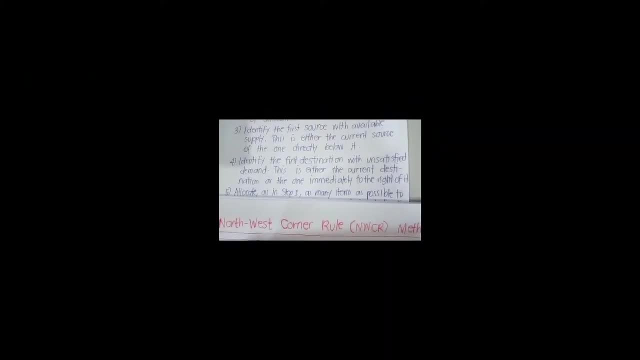 step number four. so, moving on to step number four, step number four is to identify the first destination with unsatisfied demand. this is either the current destination or the one immediately to the right of it. now going back to our problem, and so, for this matter, these are now our remaining. 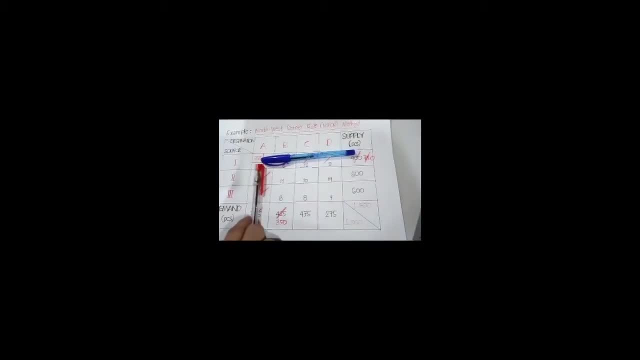 cells, since these are already cancelled out or marked out. these are now our remaining cells. with this, where is our northwest corner? so our northwest corner that would be located here. okay, with an 11 transportation if you go a step up and eliminating them all, this means that it is the time when it is best. 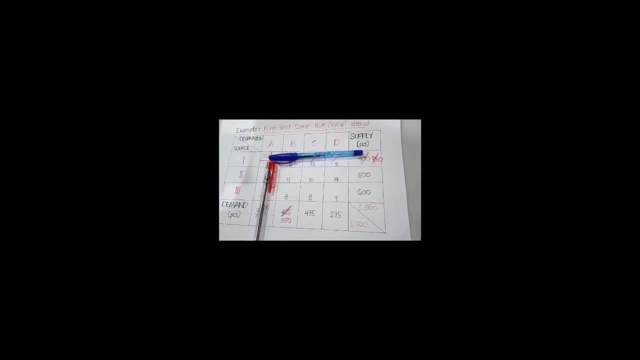 to identify station that does not SURGE fish property protection right. so this gives you the right to call this destination, that is a destination, a total of three hundred and fifty pieces remaining. and with respect to source two, which is this one: okay, it has a total supply. 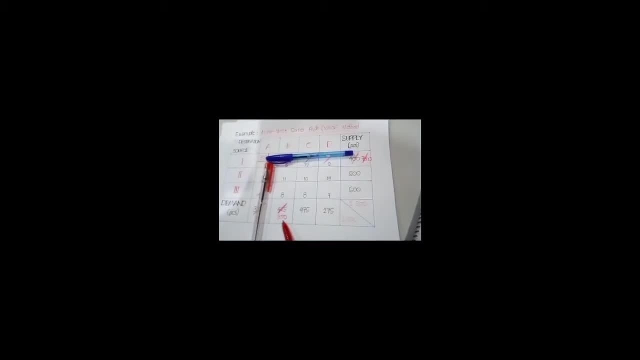 of costs for the five sets. each and five is already- 우리는 자체만 nonsense- a totalimana 500 pieces. now, since 350 is lesser than 500, then we will be allocating 300 pieces here. okay, so that would be 350 pieces. okay, we just plugged in our value right here, so therefore, 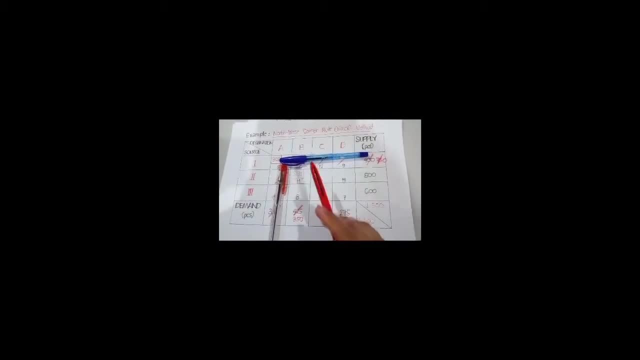 350 minus 350, this becomes zero, and 500 minus 350, so that becomes 150. okay, so this is 150. so moving on to step number five. step number five is where we need to allocate, as in step number one, as many items as possible to the route associated with the origin or source destination combination. 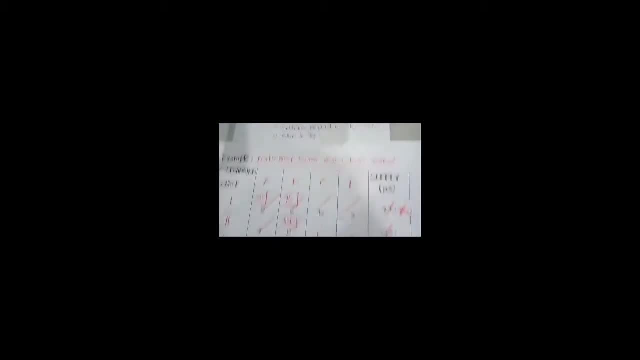 identified in steps numbers three and four. now, going back to our problem right here now. in this case, these are now the only remaining cells that we have. okay, as you can notice, we have one, two columns and one, two rows remaining. okay, these are what we call three. 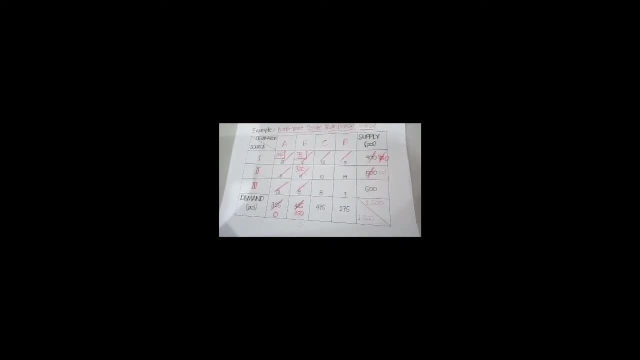 our unlocated cells. now, based on step number five, we need to allocate as many items as possible to the route associated with our source destination combination and, as you can notice, that route is the route source to, okay, this one and destination c, so source to destination c. 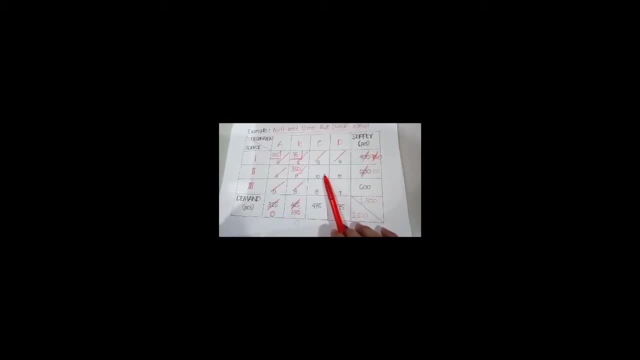 this is where we need to do our allocation. in this case, we need to allocate as many items as possible. so we need first to give us our value demand, the current value of our value. here we need to use 10 dollars and we will plot this value, value, value. this is right here. 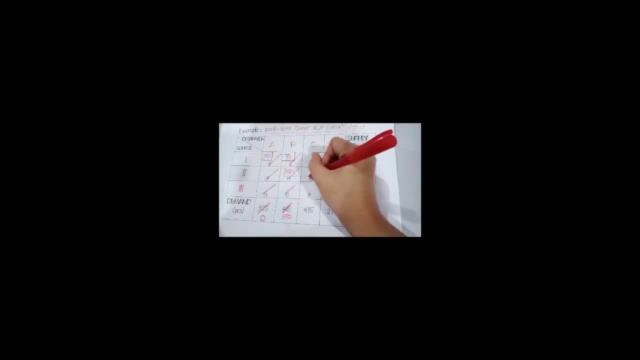 this is also our northwest corner of our cell, so we will select this cell and allocate the value. okay, so we will select this and this is where we will allocate the value. so before doing the allocation, remember that we have to match first the value of our demand. 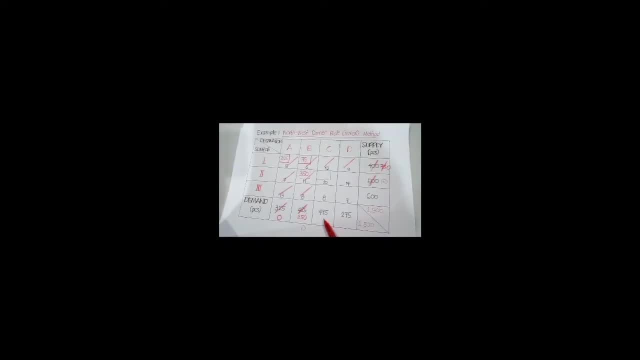 versus the value of the price. ok, we have selected that to be 10 units. okay, so I found property is the value of our supply. now, in this case, as you can see, we have a total of 475 pieces for our demand and for our supply we have a total of 150, and clearly 150 pieces is lesser compared to 475. 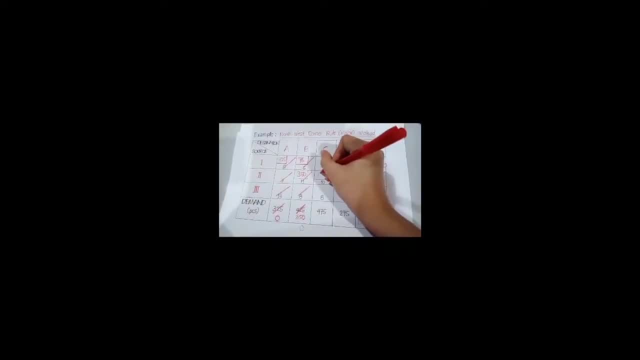 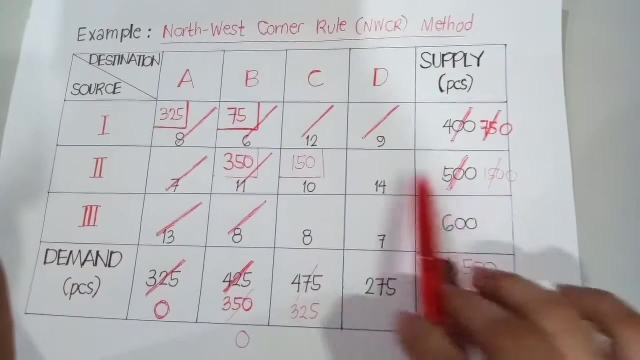 pieces, and so, because of this, we will allocate 150 pieces right here, and 150 minus 150- this becomes zero. and 475 minus 150- now that becomes 325. since this row is zeroed out, that means to say that we are now able to mark. 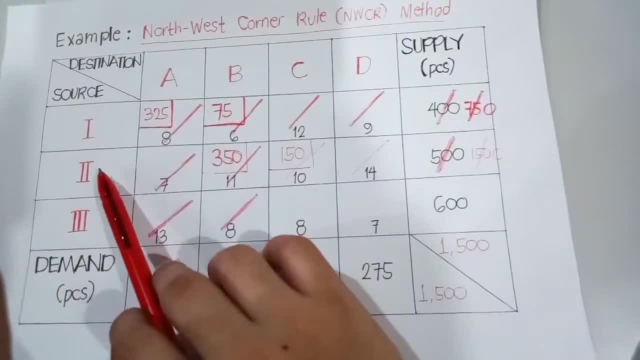 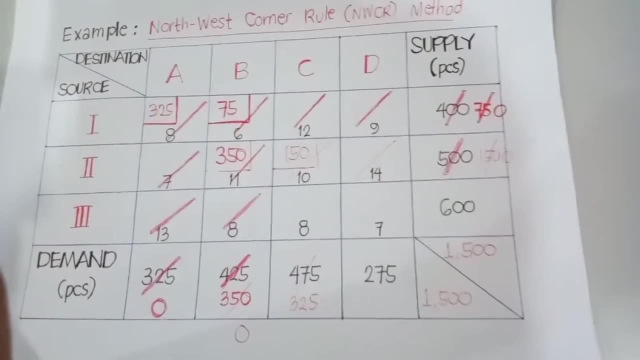 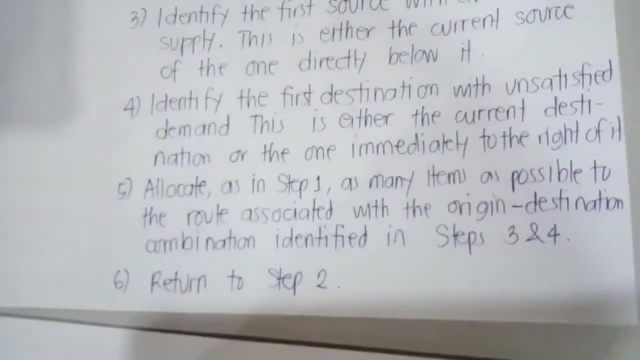 the the out or cancel the entire row. source 2.. Okay, so that is rule, or step number 5.. Now moving on to step number 6.. For step number 6, it says return to step number 2.. So what we did on step number 2,. 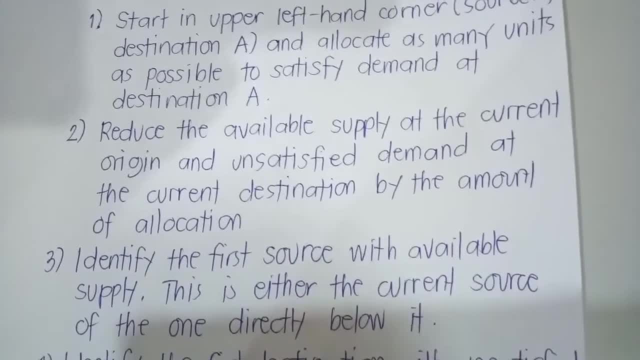 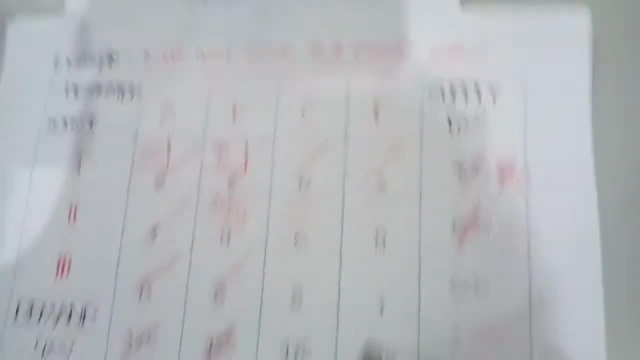 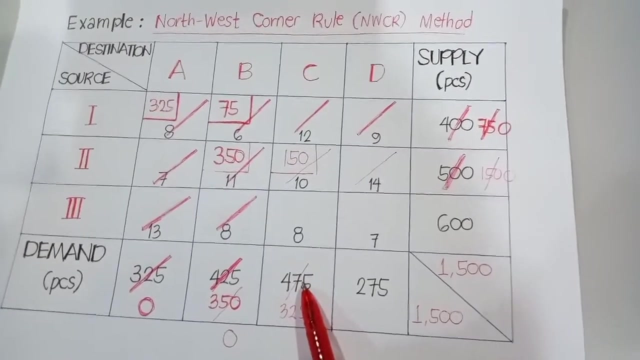 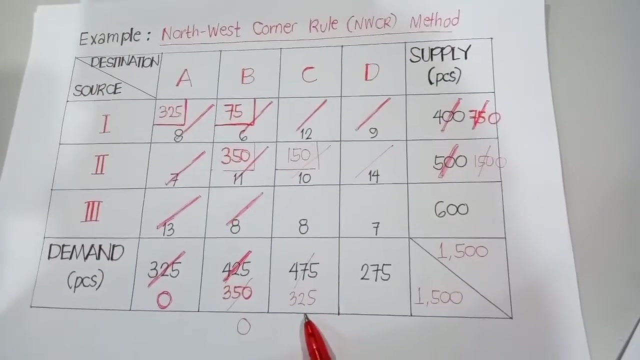 we reduce the available supply at the current origin and unsatisfied demand at the current destination by the amount of the allocation. Okay, as you can notice, we have already do the reduction. So 475 was already deducted by 150 and this now becomes 325.. Okay, so right now. 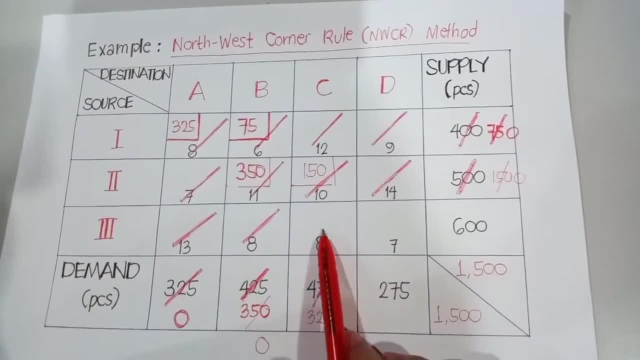 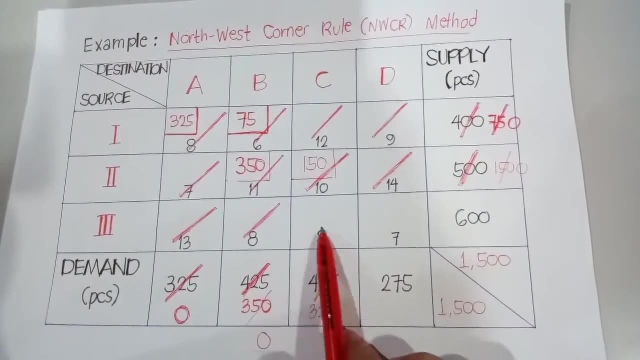 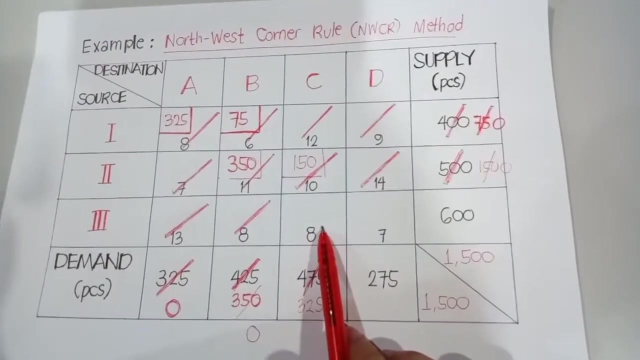 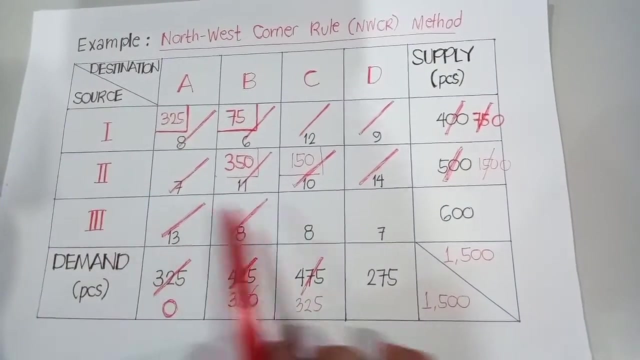 now with our remaining unallocated cells, which are these two cells? as you can notice, this is our northwest corner, So this is where we will allocate next. So, as you can notice, matching the quantity of our demand versus the quantity of our supply. with respect to source 3, destination. 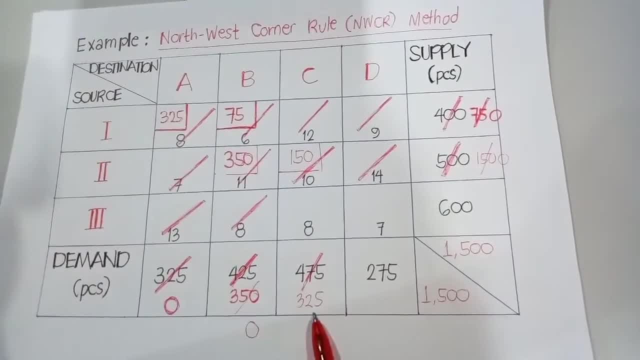 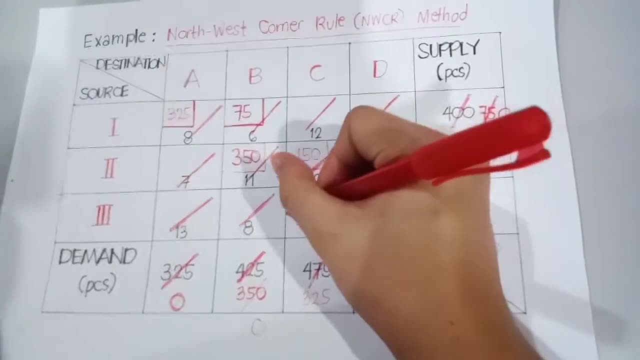 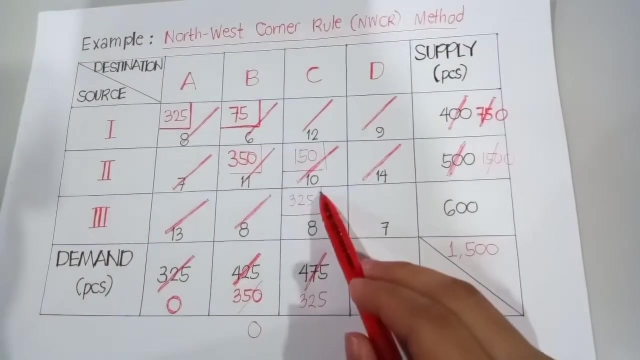 C, So our total demand is 325 pieces and our total supply is 600 pieces, And so, for this matter, we will allocate 325.. We will allocate 325 pieces in this cell And 325 minus 325, this becomes 0.. And 600 minus 325,. 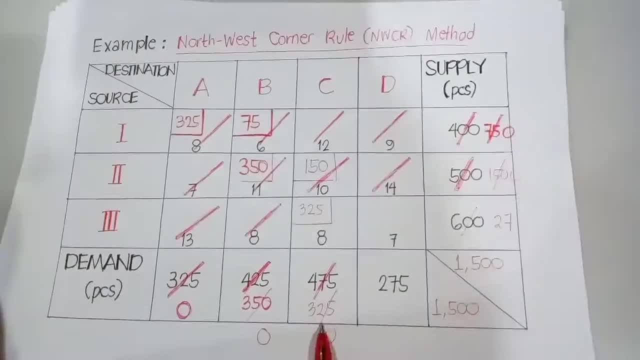 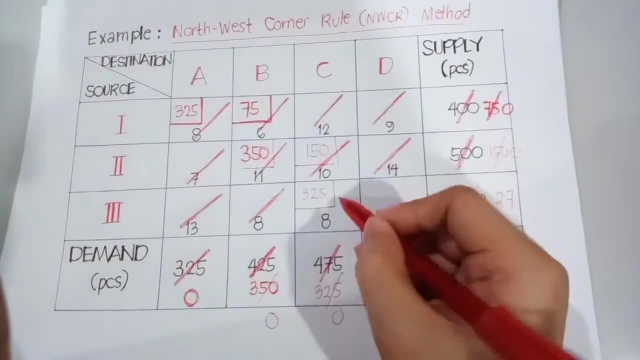 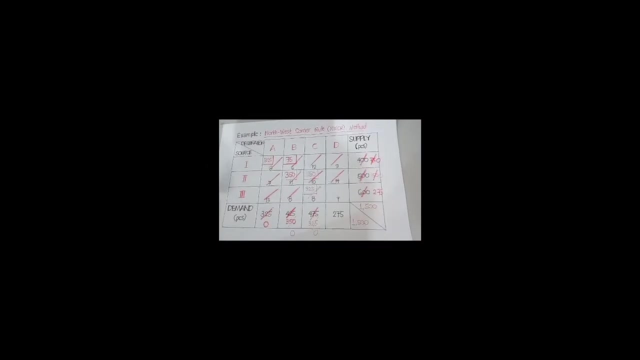 this becomes 275.. Now, since this amount is already zeroed out or exhausted, that means to say that we are now able to mark this out or cancel out the entire column C And, finally, we only have one unallocated cell remaining, which is this one. So, as you can, 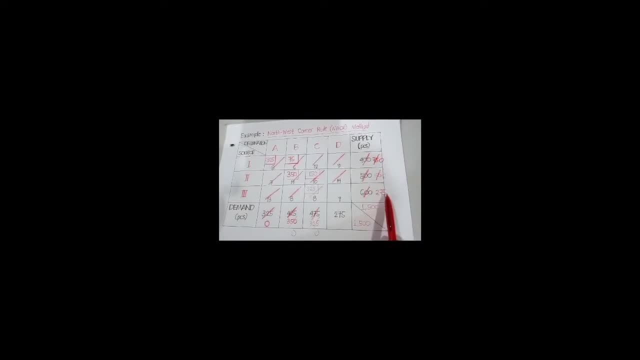 see, both demand and the supply value are the same. You have 275 pieces for your remaining demand and 275 pieces for your remaining supply, And so, for this matter, we will be allocating this one right here: 275.. 275.. 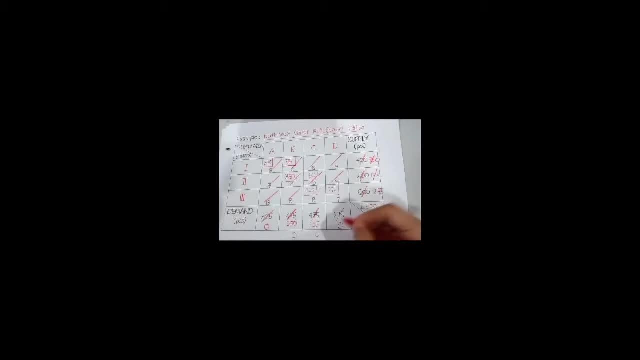 275.. 275. 275.. this becomes 0.. 275 minus 275, this also becomes 0.. Since all of our cells have been exhausted already, the next thing that we need to compute is to calculate our transportation cost. So this: 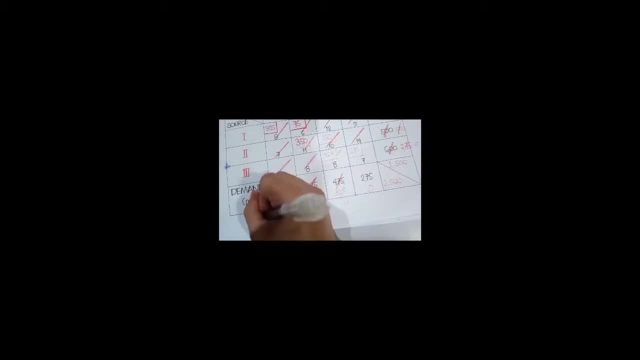 is how we will calculate our transportation cost. Okay transportation cost: you have 325 times 8.. Okay, 325 times 8 plus, you have 75 times 6.. So 75 times 6 plus, you have 250 times 11.. 350 times 11 plus you. 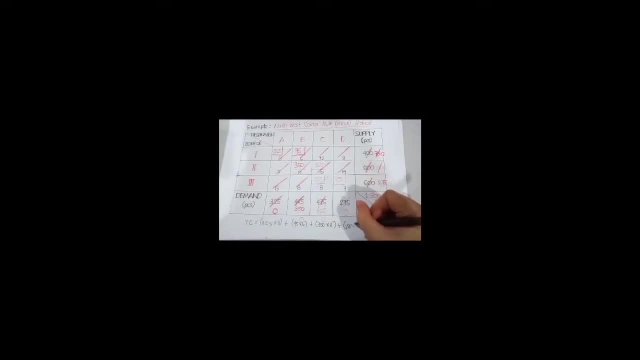 have 150 times 10.. 150 times 10 plus 325 times 8., 325 times 8 plus 275 times 7. Plus 275 times 7.. row transportation cost for this particular problem, that will be $12,925.. 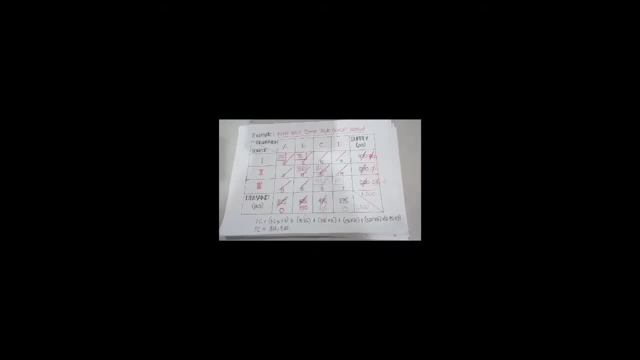 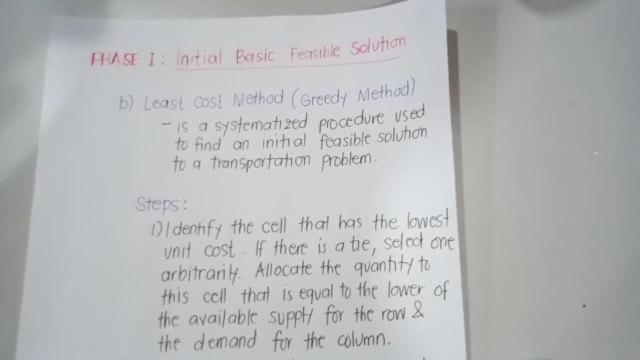 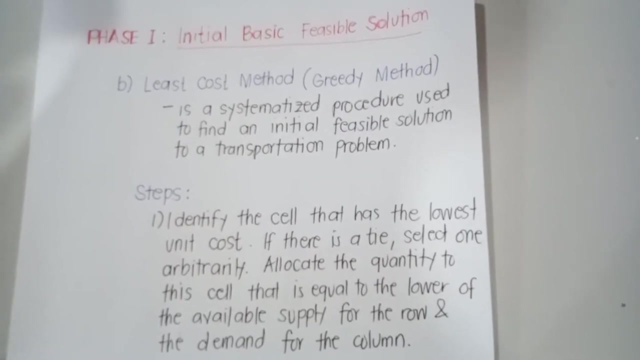 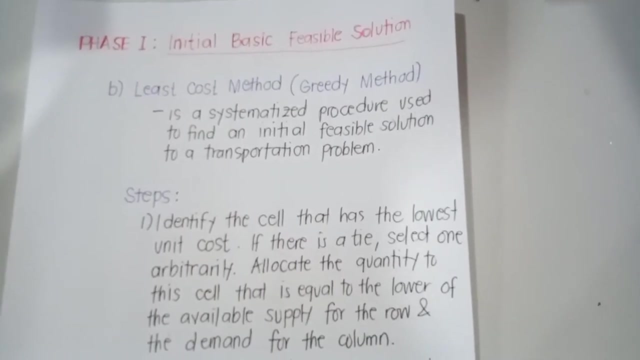 Okay, that is Northwest Corner Rule Method. Now, the second method used to establish the initial basic feasible solution is what we call the least common method, or also known as the greedy method. The greedy method is a systematized procedure used to find an initial feasible solution. 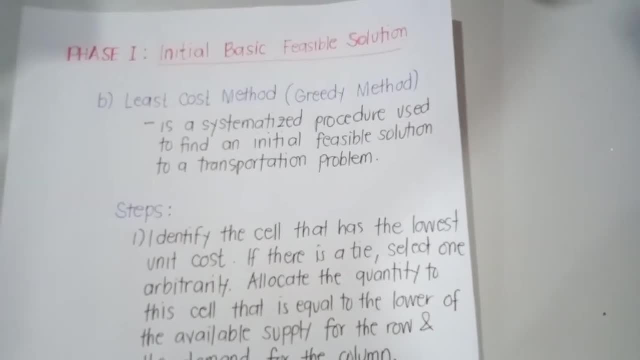 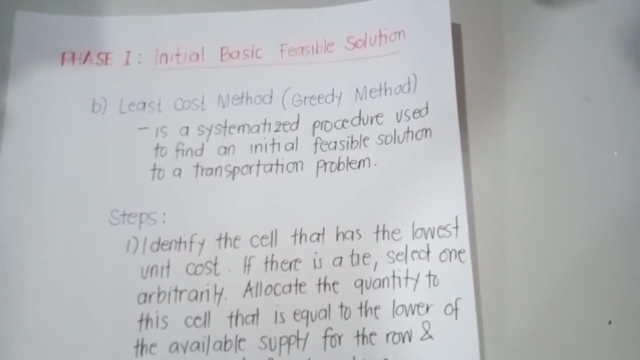 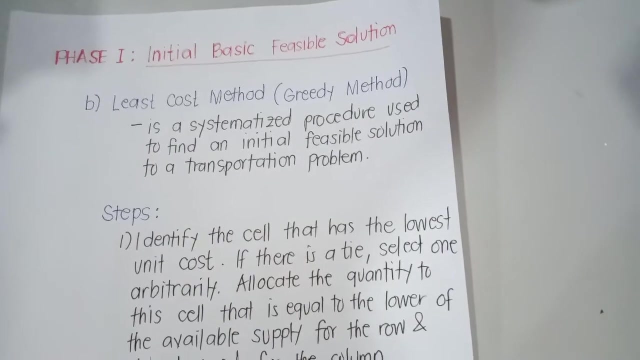 to a transportation problem. Now, in this method, the allocation begins with the cell which has the minimum cost, and the lower cost cells are chosen over the higher cost cells, with the objective to have the least cost of the transportation. Now, in order for us to better understand, 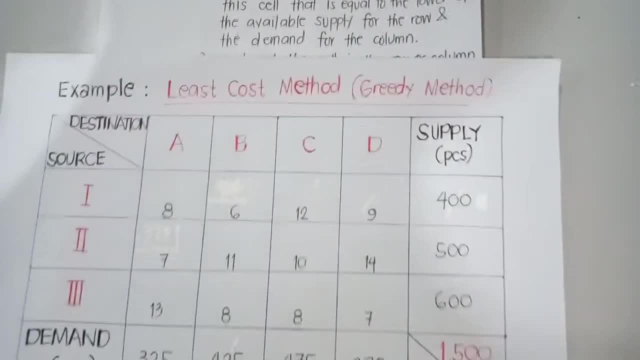 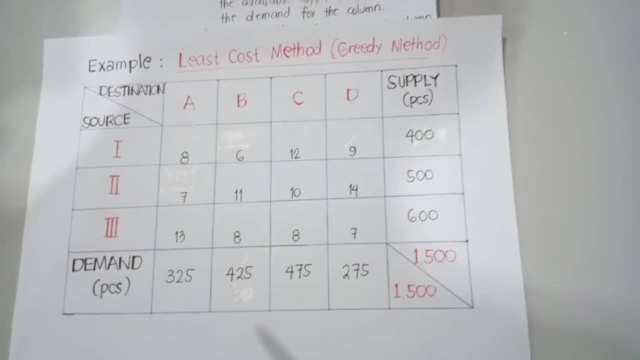 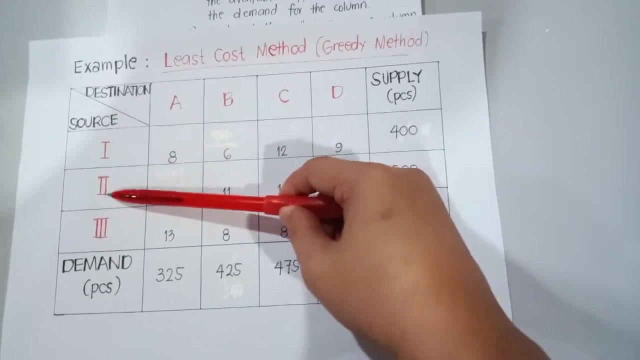 the least cost method. let us have our example. So this is how our example looks like. Okay, as you can notice, we have source column. So, with respect to source column, you have three sources: source one, two and three- And also you have your destination. 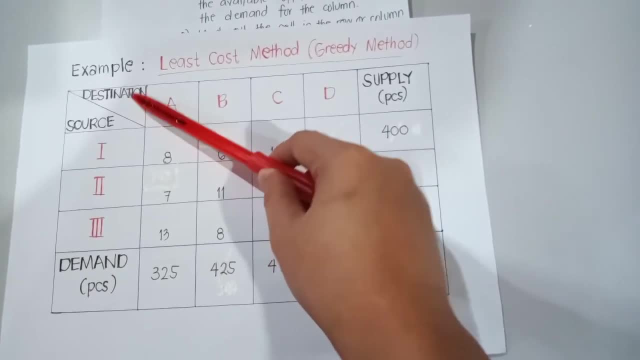 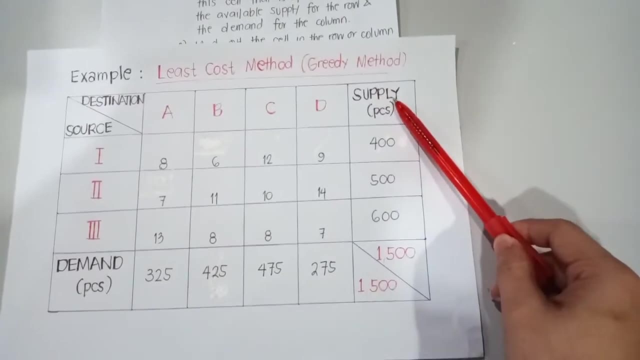 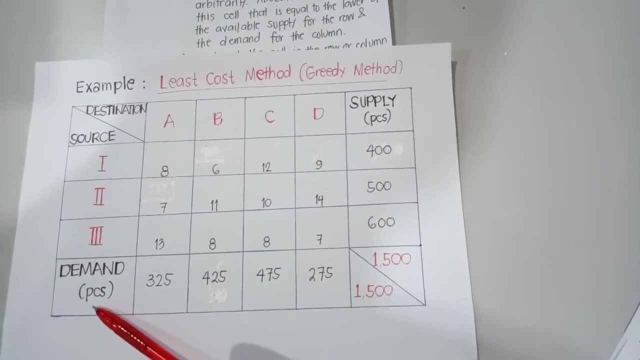 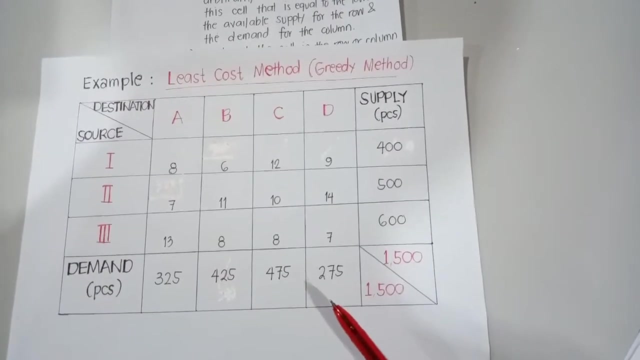 columns And your destination is denoted by points A, B, C and D respectively, And for the last column, you have your supply column in terms of pieces And your last row is your demand row, which is in pieces, And, as you can notice, this is an example of a balanced transportation problem. 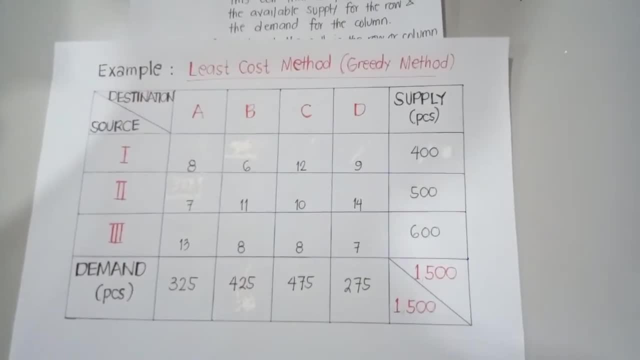 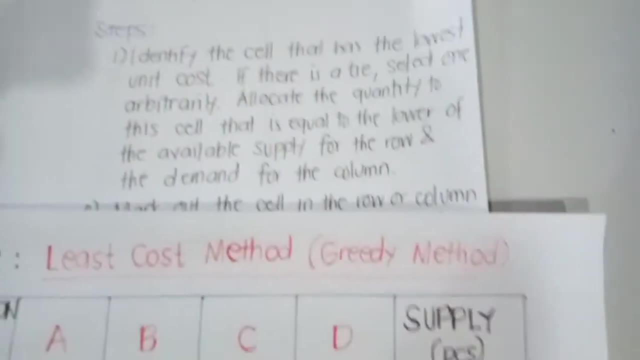 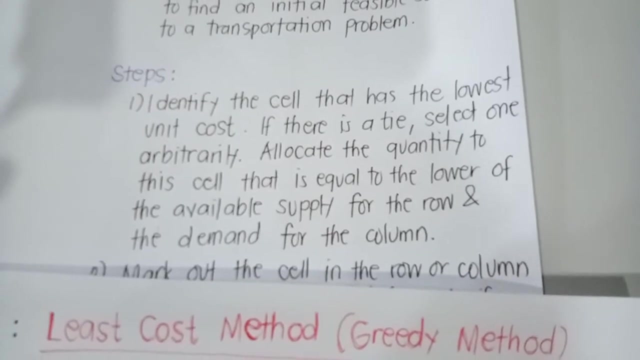 Now, in order for us to be guided in doing the least cost method, then we need to strictly follow the steps. Now, first one in least cost method. that would be, identify the cell that has the lowest unit cost. If there is a tie, select one arbitrarily. 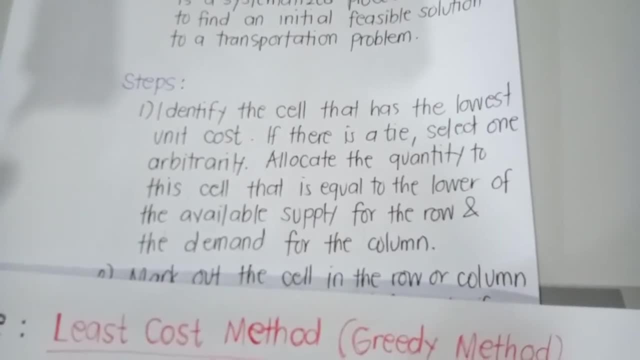 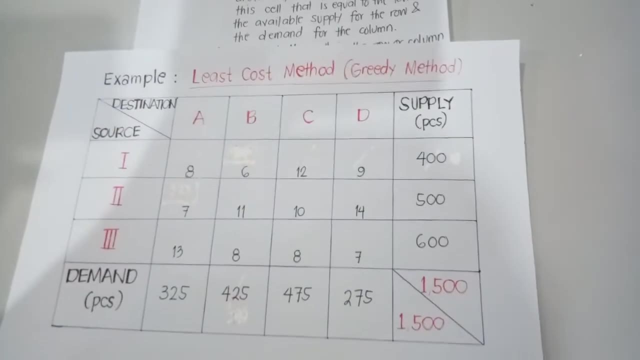 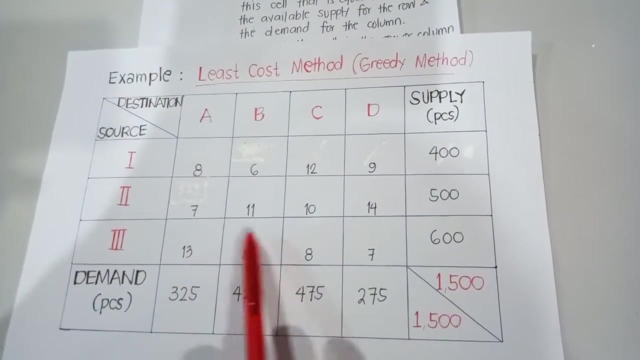 Allocate the quantity to this cell, that is equal to the lower of the available supply for the row and the demand for the column. Now, going back to our problem, we have 12 different costs. right, We have 1,, 2,, 3,, 4,, 5,, 6,, 7,, 8,, 9,, 10,, 11, 12.. These are 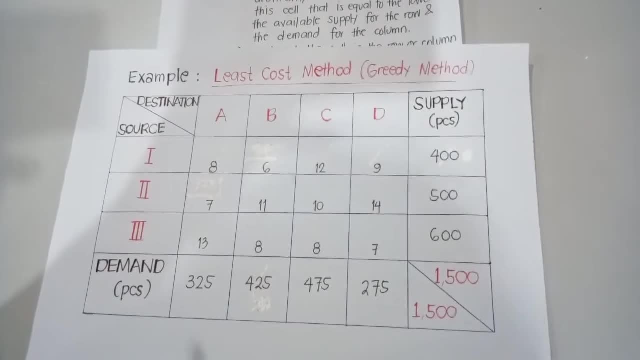 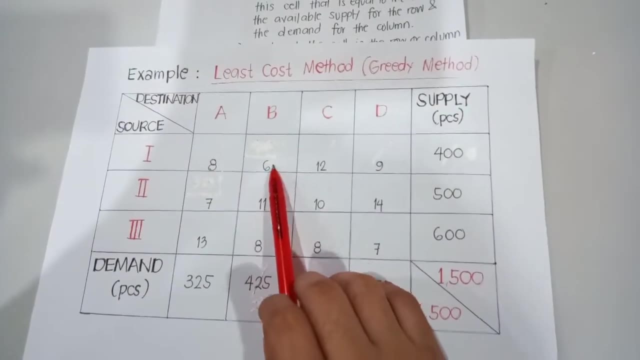 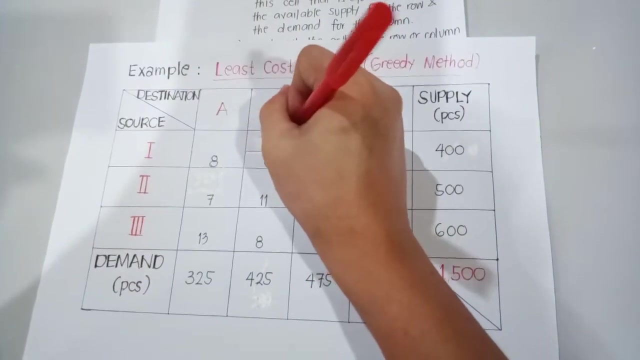 our transportation costs. Now, with respect to this cost that we have, the least cost is we have six And therefore this is the cell in which we will do our first allocation. okay, So this is where we will allocate the least cost And this is the cell in which we will do our first allocation. 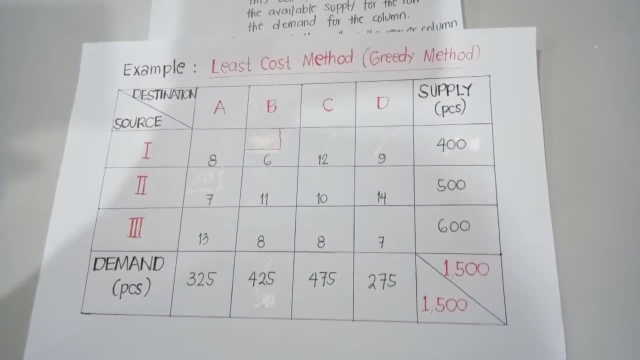 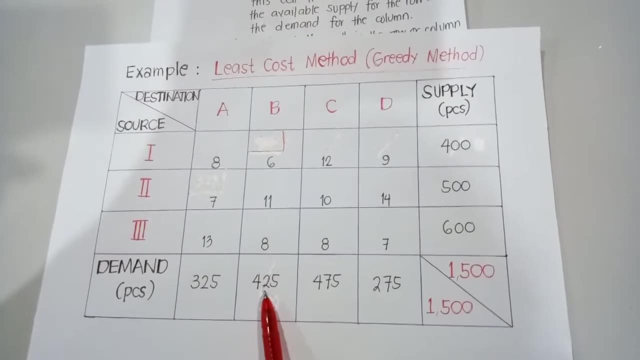 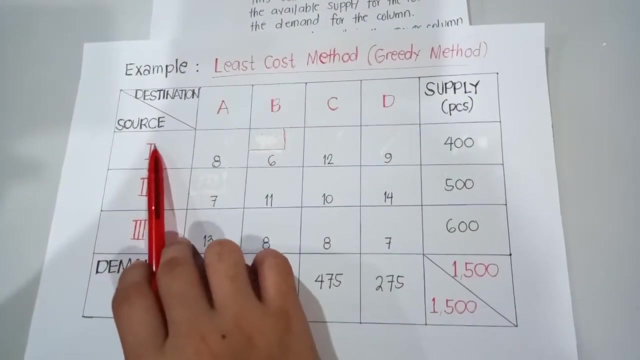 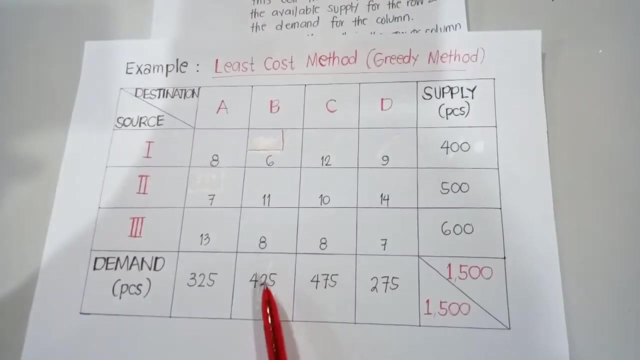 first. So how do we do that? How do we allocate? Now, in allocating, we need to match the quantity of our demand and the quantity of our supply. As you can notice, the quantity of our supply with respect to source 1, destination B, which is this cell, is 400 pieces, And for the demand, 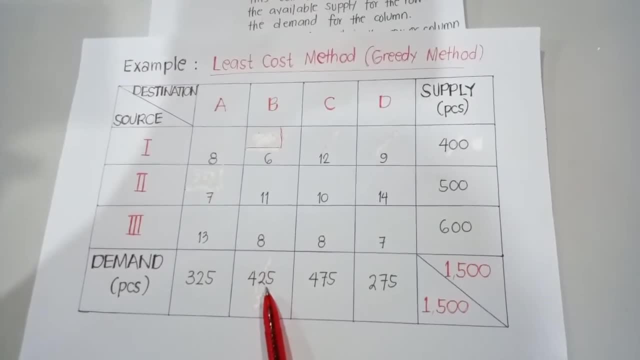 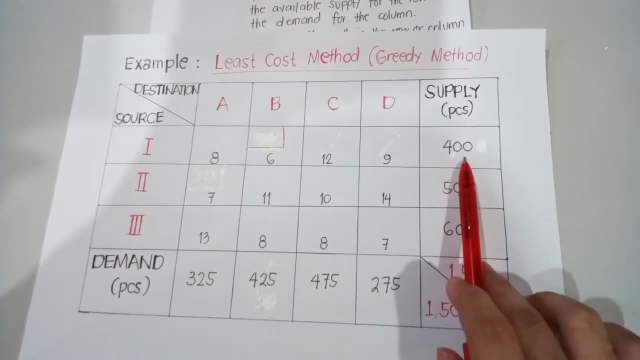 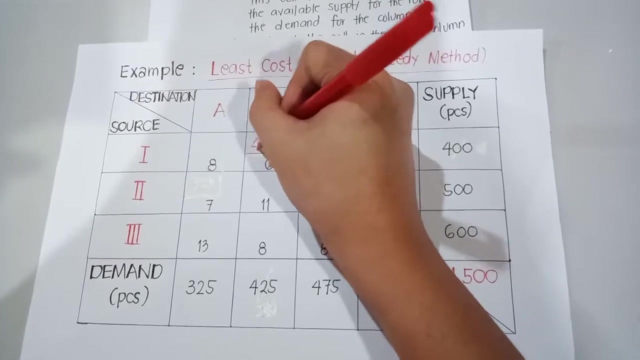 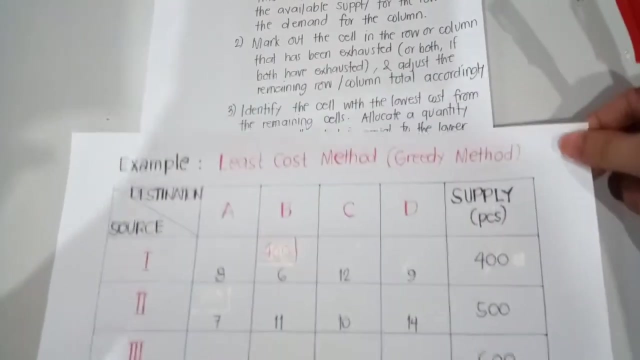 you have 425.. Now what we need to allocate is the one which has the least value, And apparently your supply has the least value: 400.. So, therefore, I will be allocating 400 pieces right here. Okay, that will be step number one And step number two. Step number two says: 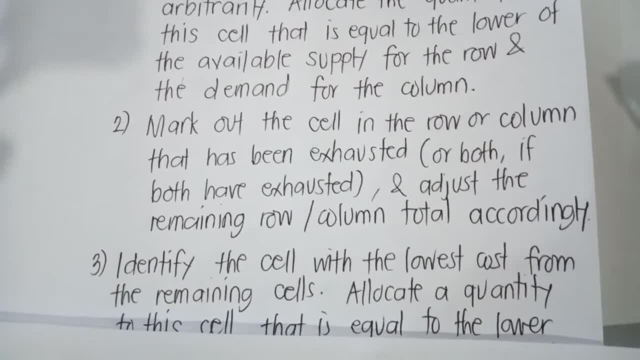 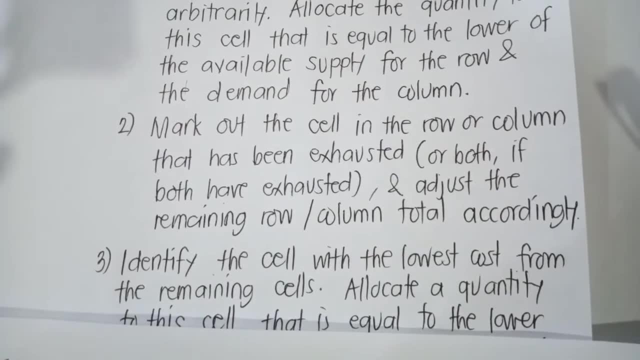 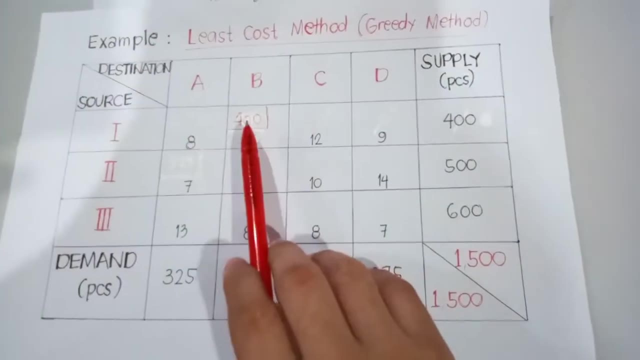 mark out the cell in the row or column that has been exhausted, or both have exhausted, And adjust the remaining row or column total accordingly. Now, in doing step number two, as you can notice, we have already allocated 400 of our supply And therefore 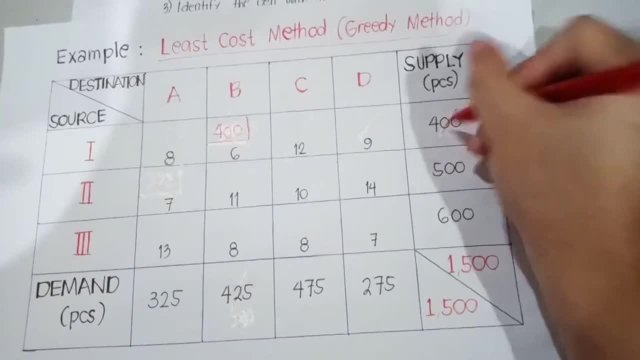 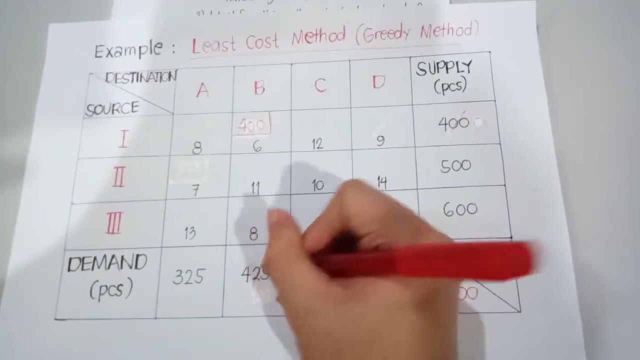 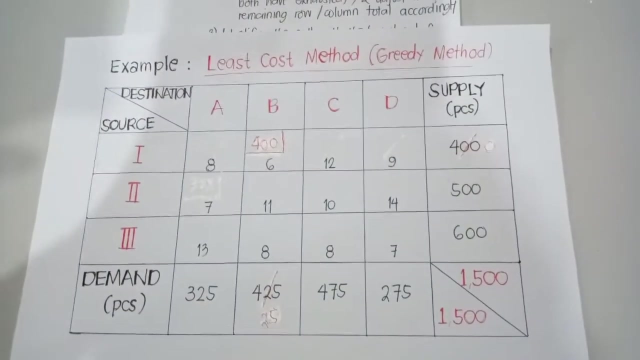 400 minus 400, this becomes zero right. And 425 minus 400, this becomes 425 minus 400, this becomes 25 pcs. Okay, that's step number two. And for step number three it says: 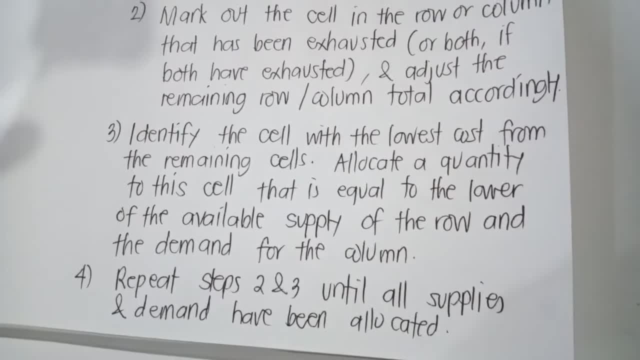 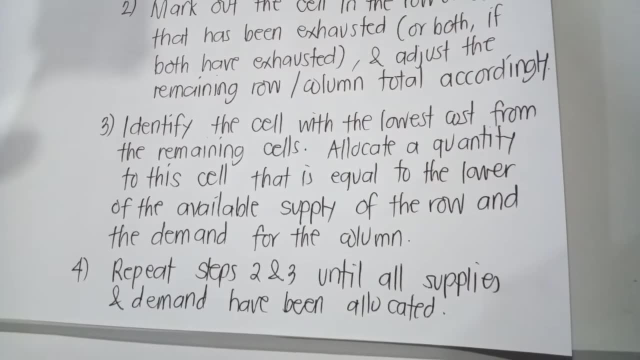 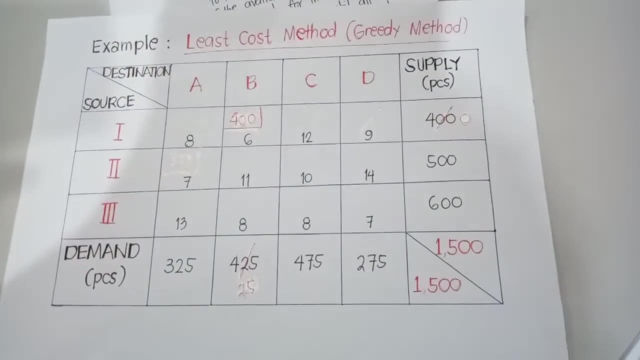 identify the cell with the lowest costs from the remaining cells, Allocate a quantity to this cell that is equal to the lower of the available supply of the row and the demand for the column. Now, before moving on to step number three, since we have already satisfied this one, 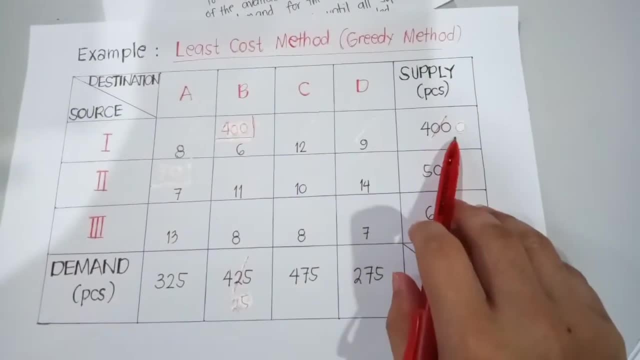 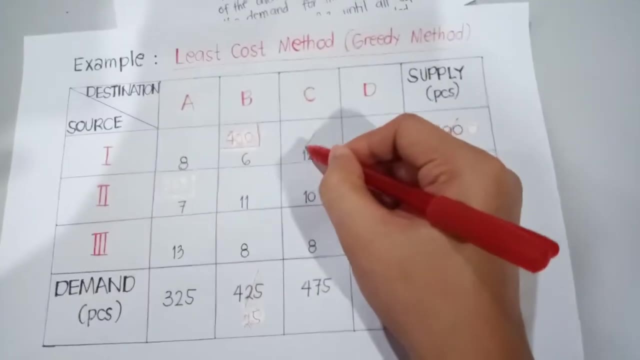 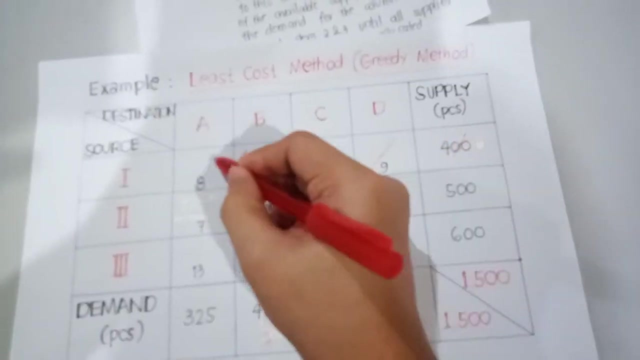 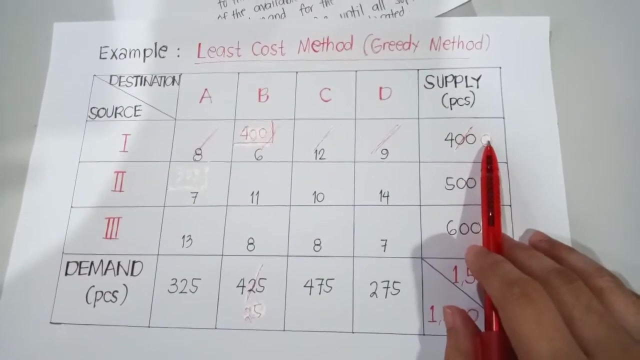 we have already cancelled out this one, right? so what we need to do next is to mark this out, mark the entire row, which is the row source one. we will no longer be needing this row, since this has been exhausted already. okay, and since this has been exhausted already, then we are having the remaining columns, or the. 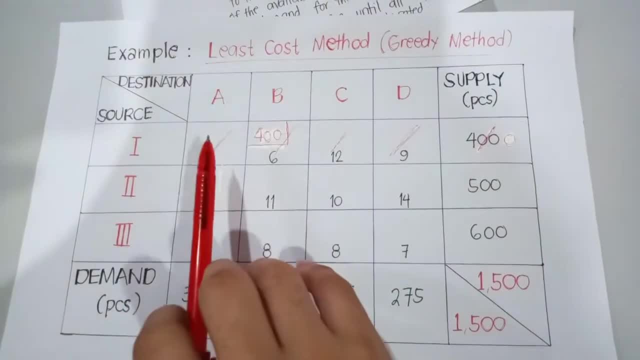 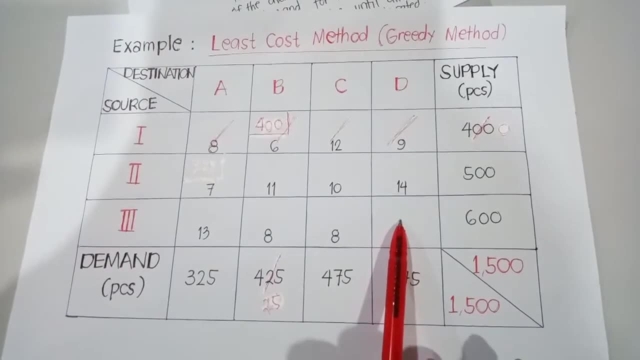 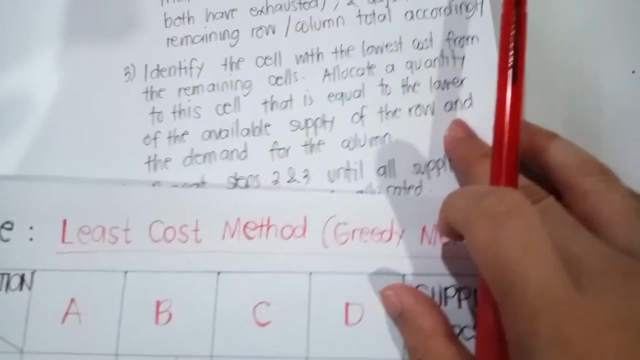 remaining cells and our remaining cells. that would be this one right here: one, two, three, four columns and two rows. these are our remaining cells and, like I said earlier, for a step number three, we need to identify the cell with the lowest cost from the row that has been exhausted already, and that is, of course. 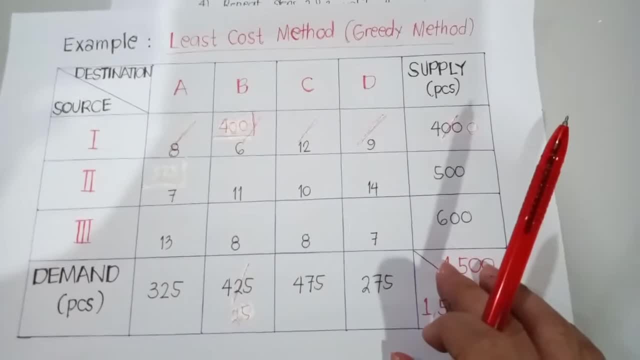 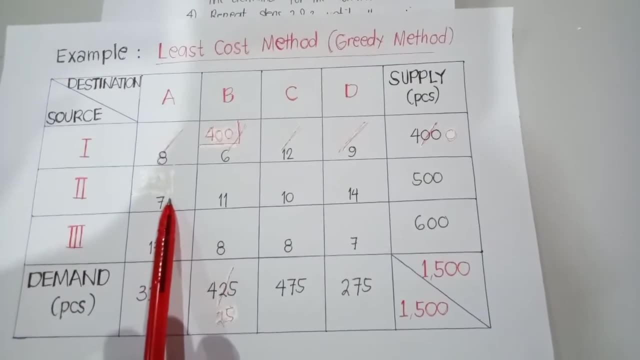 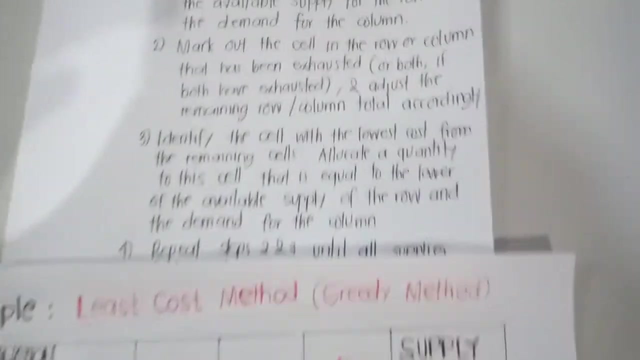 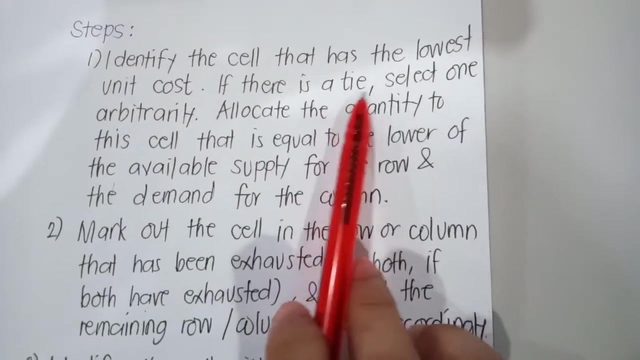 remaining cells. now, as you can notice, for our remaining cells the lowest cause that would be seven, right, but remember there are duplications. we have two sevens right here, seven here and seven here now. as you can recall, in step number one, it is stated here that if there is a tie, we need to. 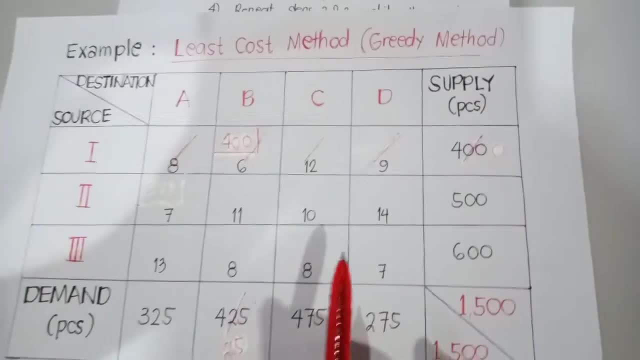 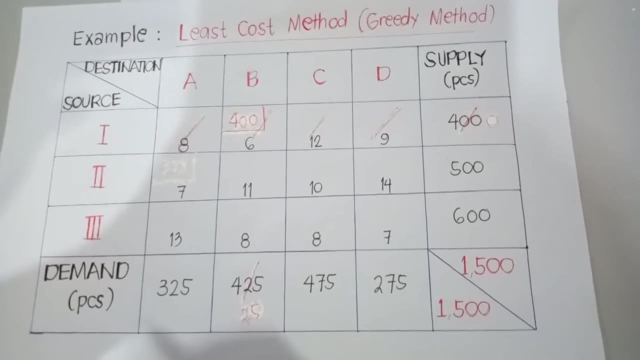 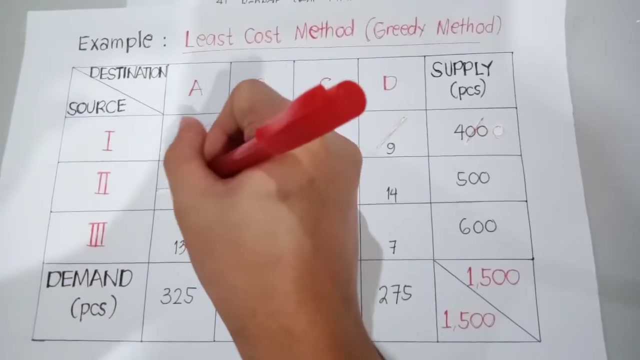 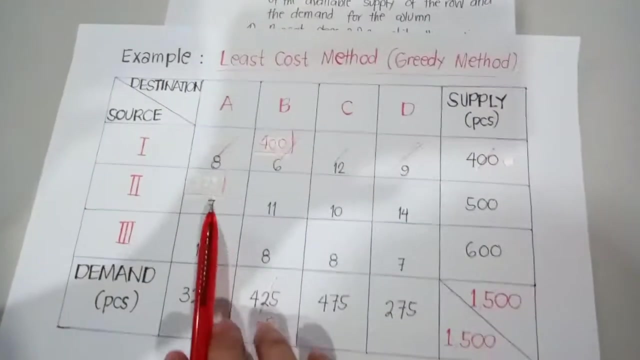 select one arbitrarily, which means to say that we have the right, we have the prerogative to select based on our preferences. okay, based on our personal whim. so in this case, I will be selecting this column right here, or this cell, cell source two and destination a. okay. so with respect to this, 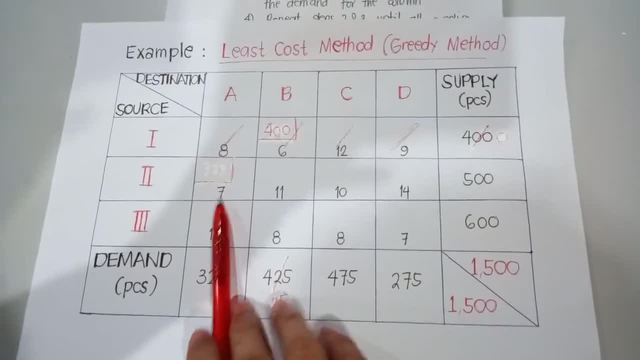 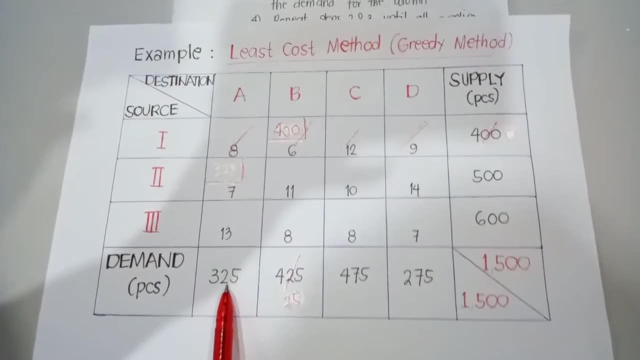 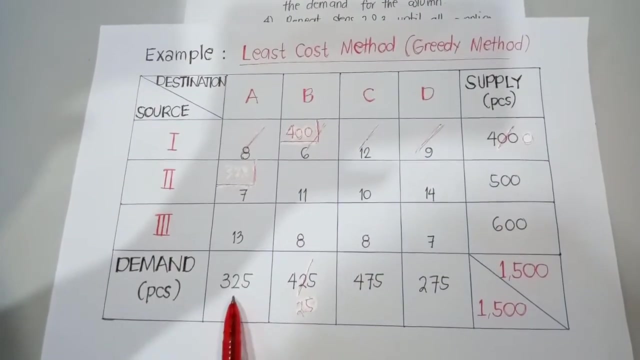 one. I will be matching the quantity of my demand demand versus the quantity of my supply. As you can notice, the quantity of my demand is 325 pieces and the quantity of my supply is 500 pieces. Now, since your demand has the least, 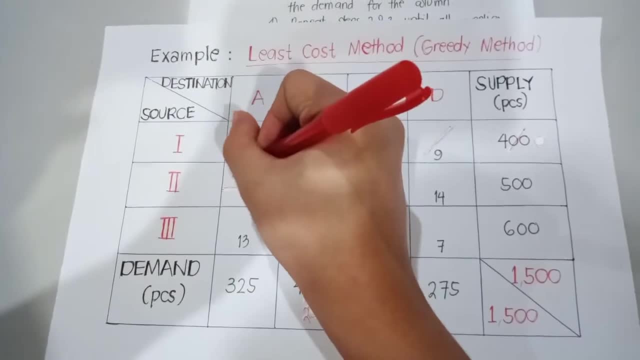 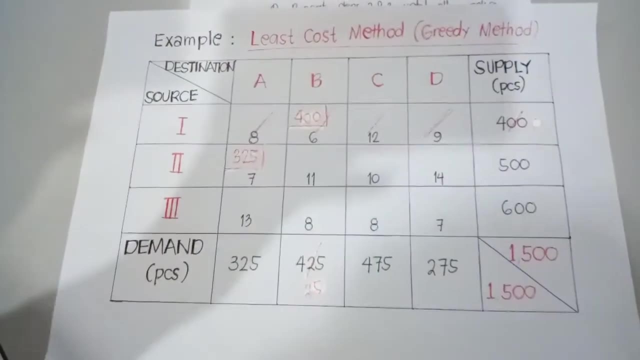 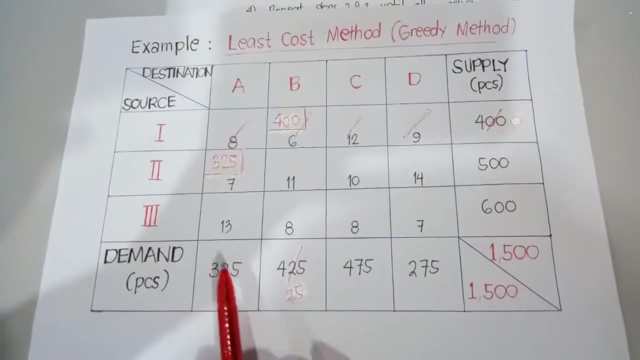 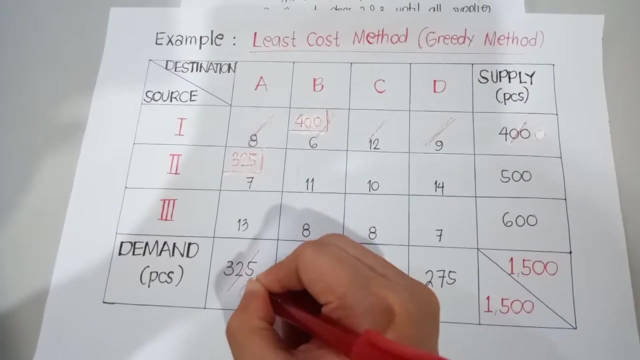 value, then this will be the one that I will be using to allocate here. So I will be plugging in 325 pieces, okay. And next, since I have already allocated 325, therefore 325 minus 325, this becomes zero. okay, This will be satisfied, this will be exhausted. and since this will be, 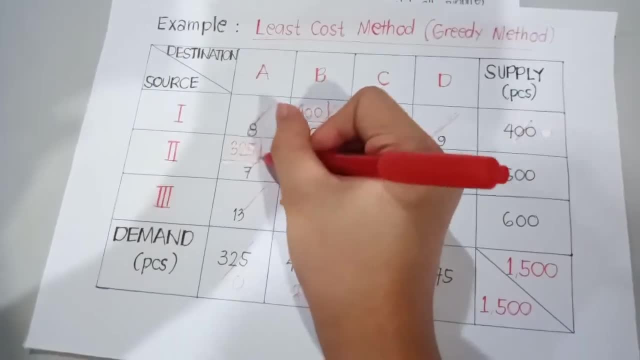 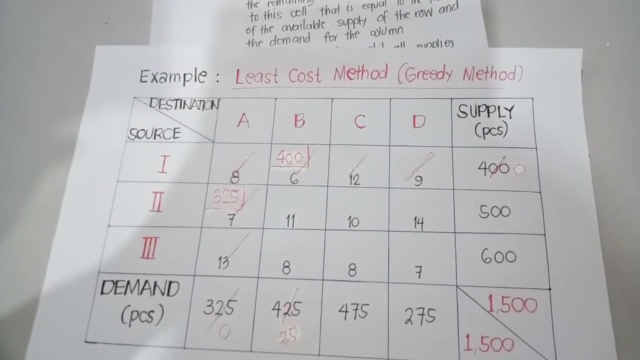 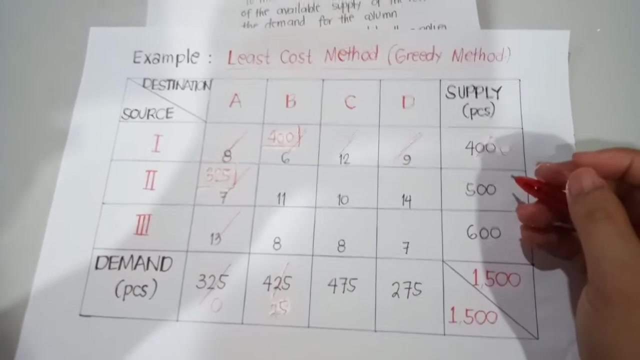 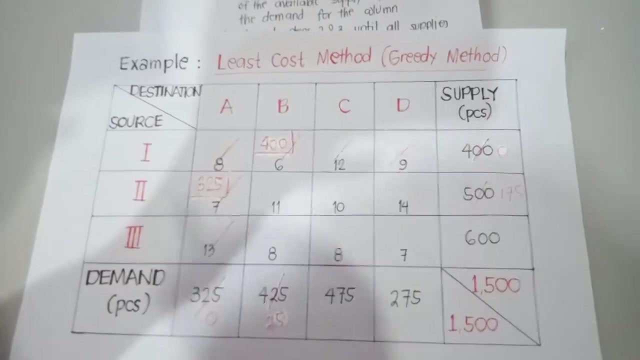 exhausted. we will be marking this out. We will be no longer using this entire column, which is column A, And we will be doing the reduction, as well, of the quantity of our supply. So 500 minus 325, so that becomes 175,- okay, 175.. And next thing that we need to do is to look at our remaining. 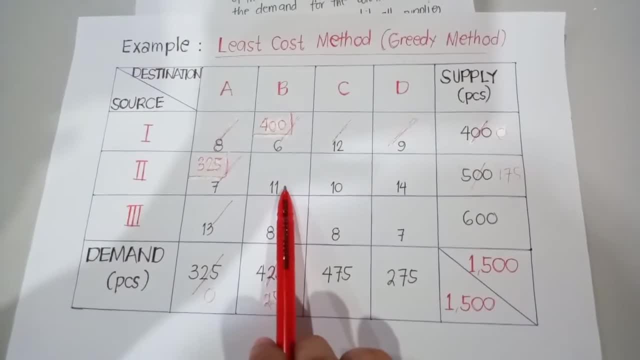 cells. So our remaining cells. we have cells 11,, 8,, 8,, 10,, 14,, 7.. And, based on our remaining cells, that will be 175.. So this will be 175.. And next thing that we need to do is to look at our 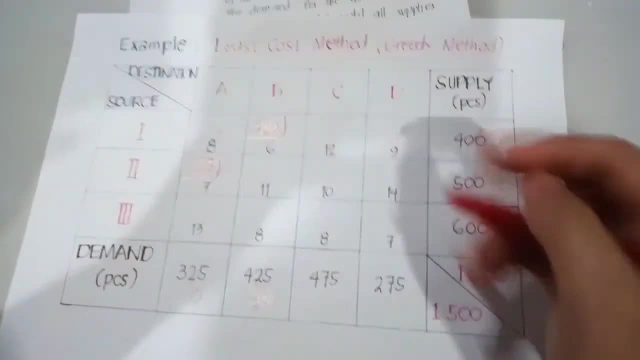 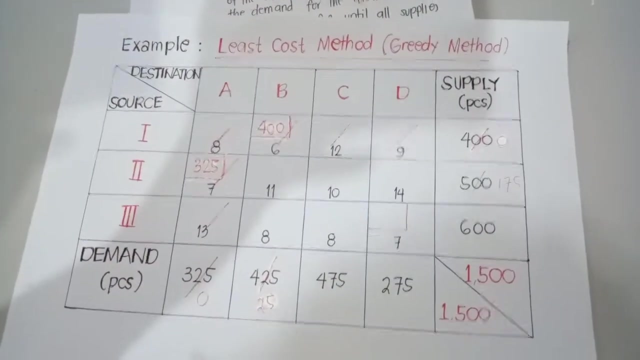 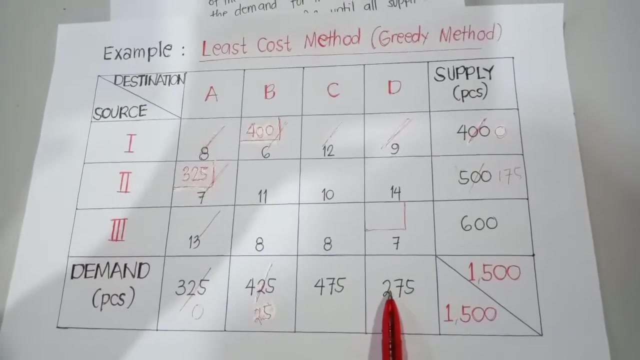 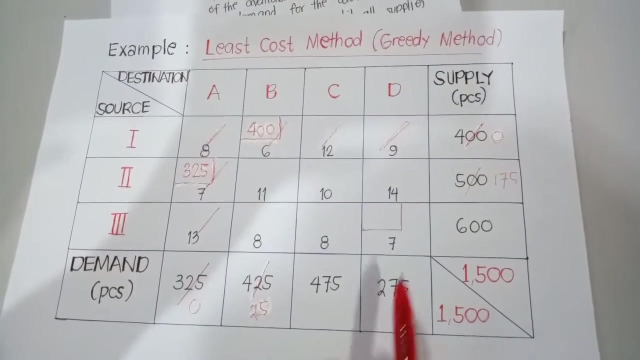 The least cost value is you have 7.. Therefore, I will be doing my next allocation right here There. And remember that in doing the allocation, we need to match the values of your demand versus your supply. Now, with respect to this cell, my demand is 275 and my supply is 600.. 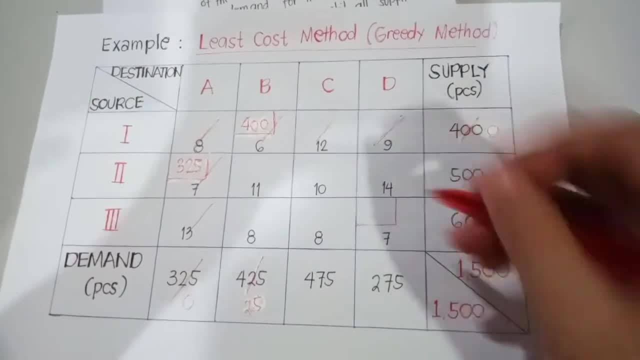 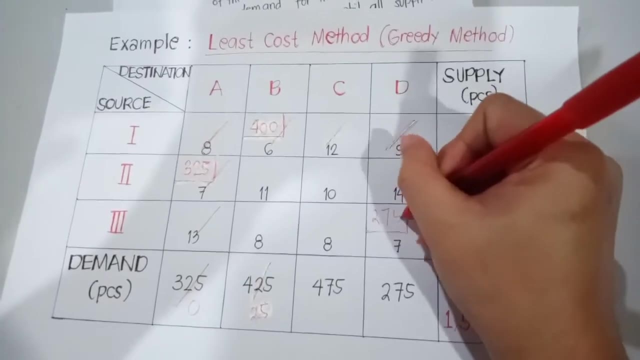 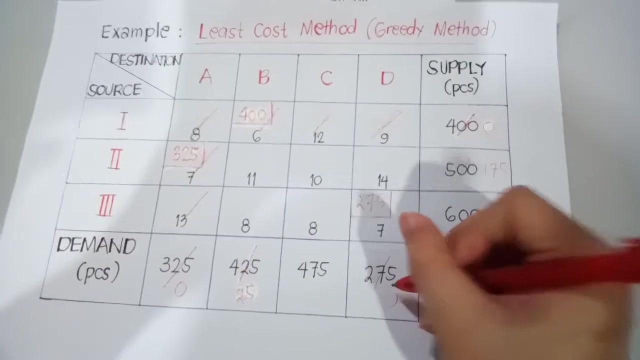 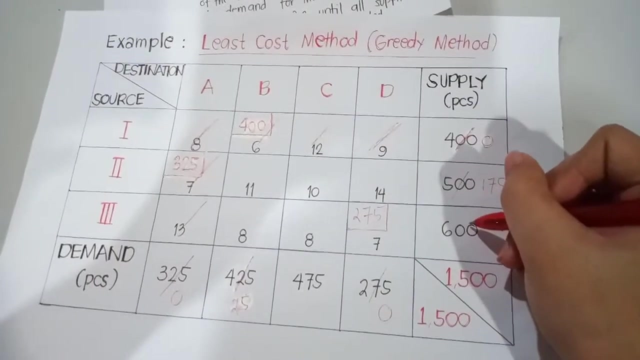 Clearly 275 has the least value and therefore I will be plugging in this value right here: 275 pieces. So 275 minus 275, this becomes 0. And 600 minus 275, that becomes 300 and 25.. 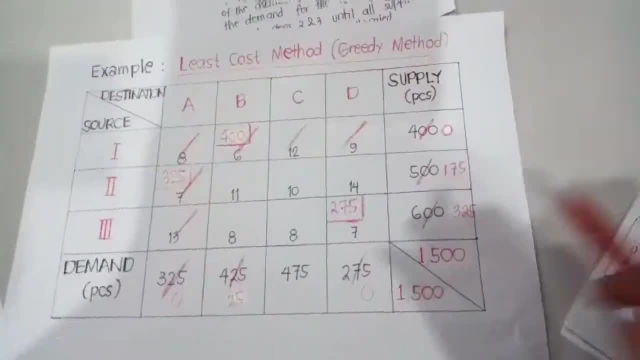 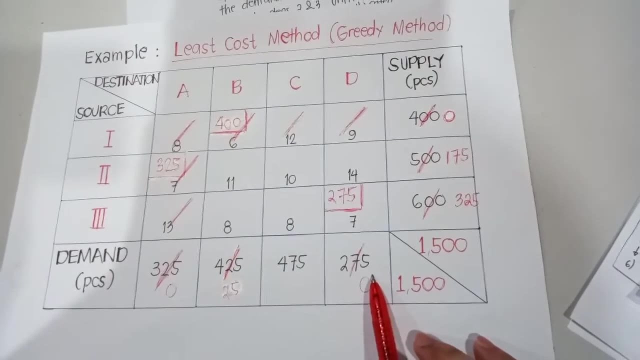 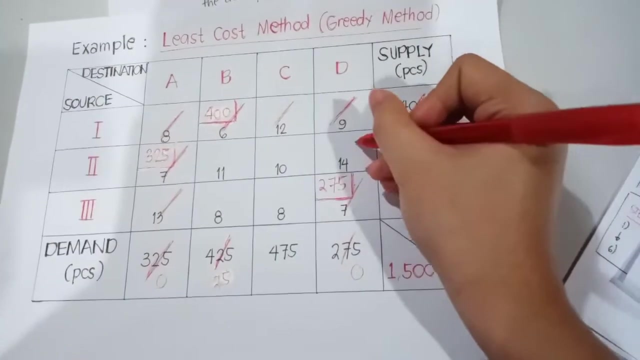 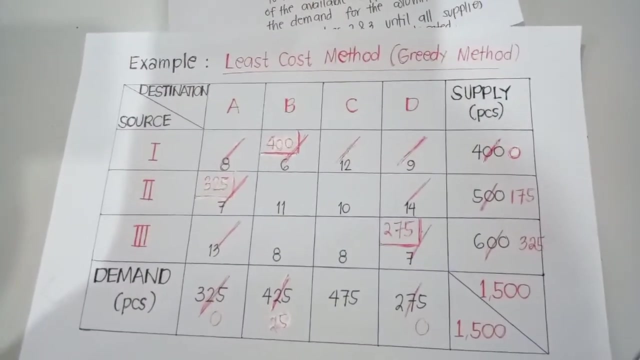 Okay, 3,, 2,, 5.. Since we already have satisfied this amount, we have already exhausted this one, which means that we are now able to mark this entire column, because we will no longer be needing this column. Okay, So, after marking out that column, we are now left with how many cells? 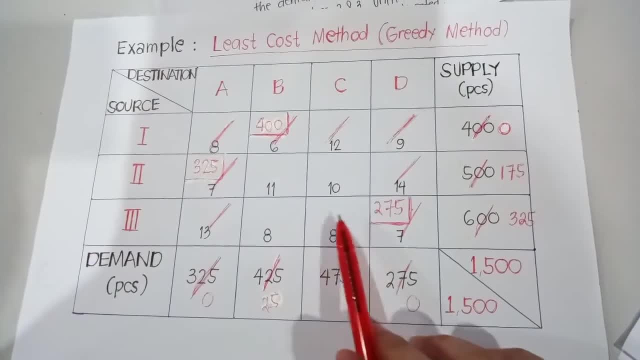 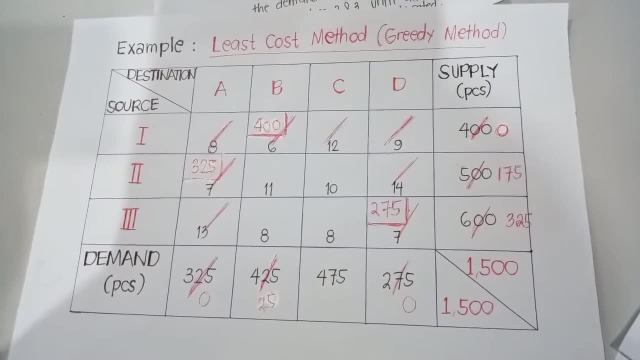 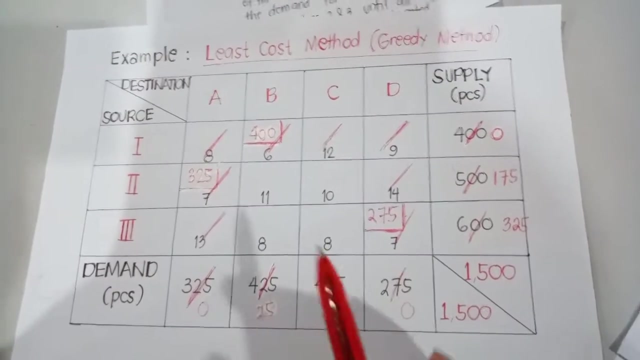 We have 4 cells, We have 11.. 10,, 8,, 8, and 10.. Now remember that in choosing the next allocation, we need to do the allocation in the one which has the least cost. Now, as you can see, there are two duplications here. 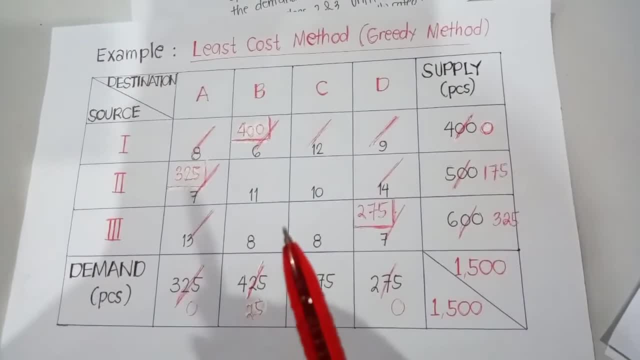 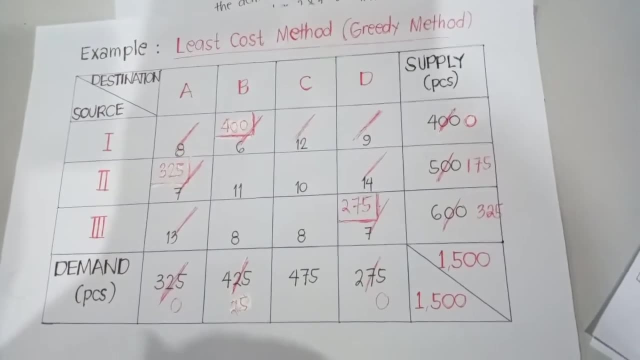 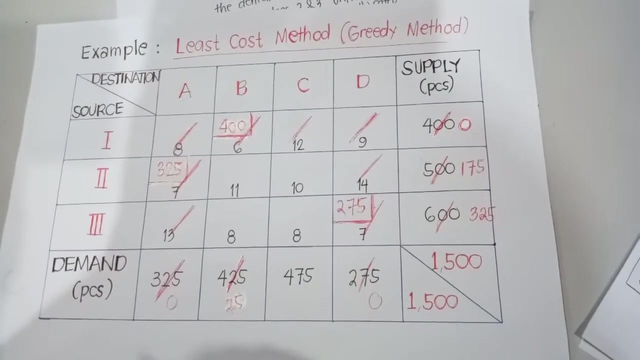 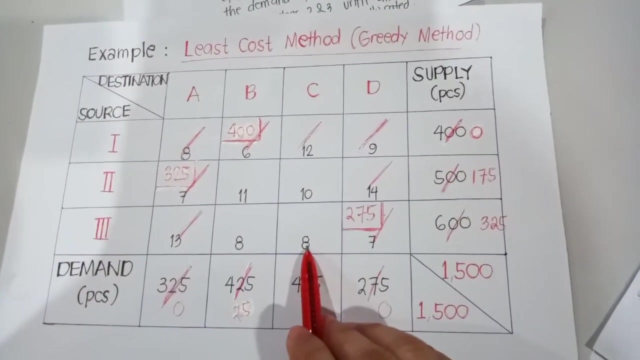 We have two 8s. So, as mentioned earlier, if you have two duplications or if there is a tie, then you have the chance to choose arbitrary, Based on your own preference, based on your personal whim. So in this case, as for this matter, I will be choosing to select this cell right here. 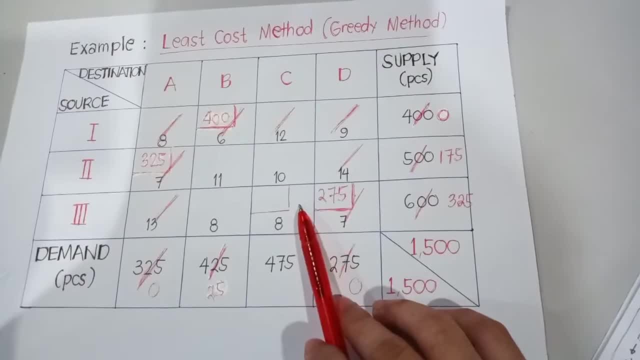 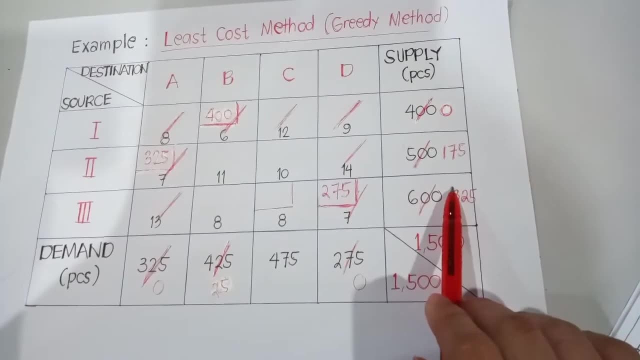 So I will do my allocation here. Now, in doing my allocation, I need to match again the quantity of my demand versus the quantity of my supply. Now, in this case, with respect to this cell, the quantity of my supply is 320.. 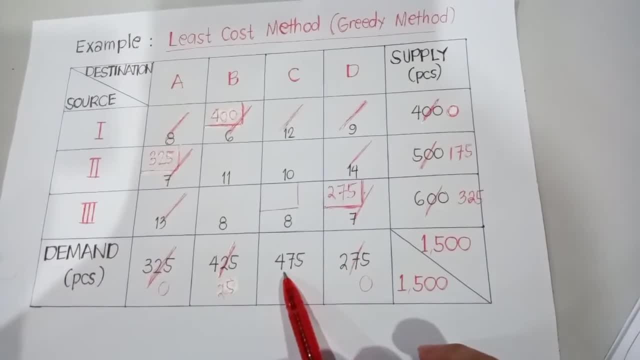 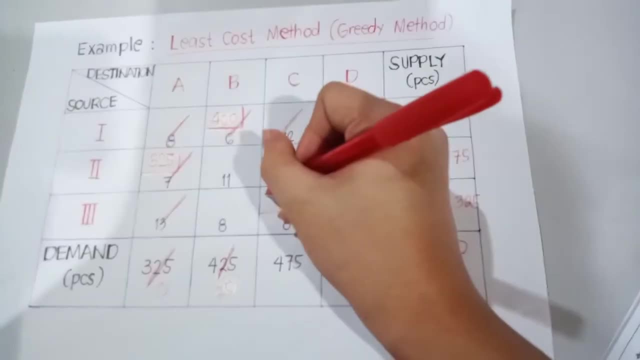 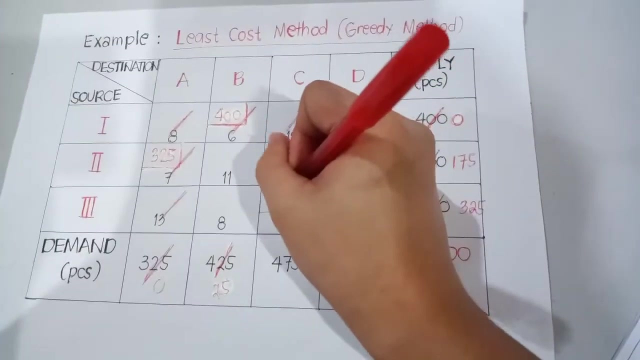 And the quantity of my demand is 475.. And therefore, since 325 has the least value, this will be the amount that I will be plugging in here. Okay, I will be allocating 325 pieces. Okay, Here you go. 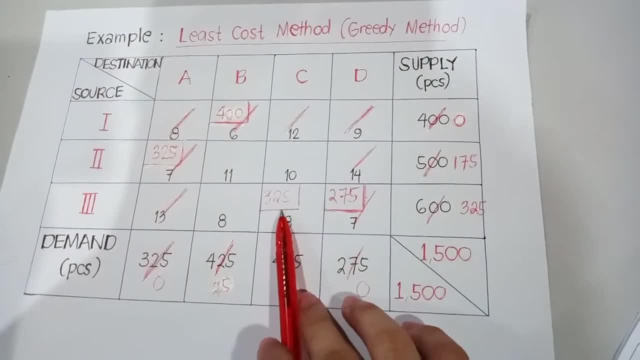 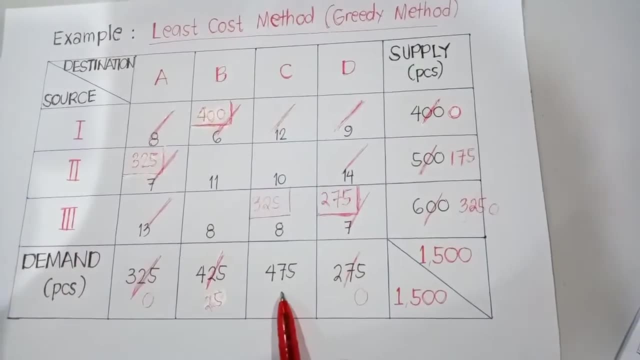 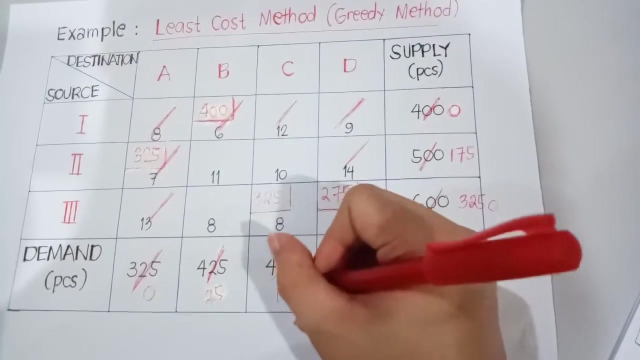 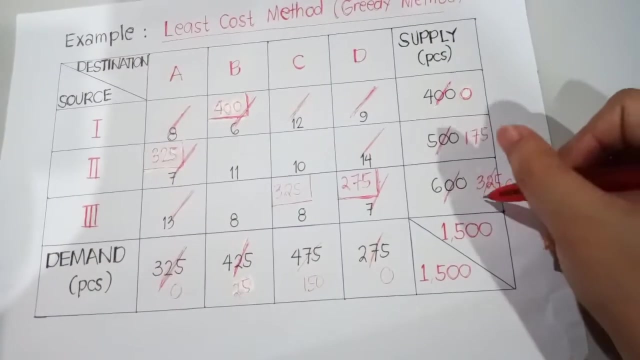 Now, 325 minus 325.. This now becomes 0.. This will be zeroed out, Okay. And 475 minus 325.. Now, this becomes 150.. Now, since this has been zeroed out or exhausted already, that means to say that we can now cancel out this entire row. 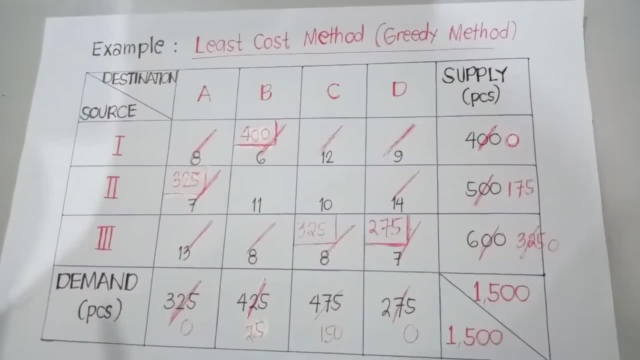 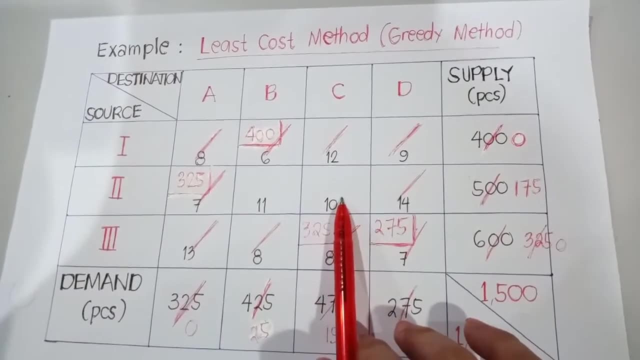 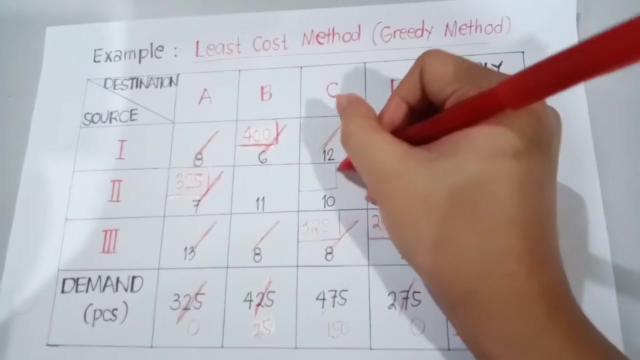 We will no longer be using this one. By canceling that out, we are now left with two cells. We have cell 11. And cell 10.. Now, since 10 has the least value, this will be the point in which we will be doing our next allocation. 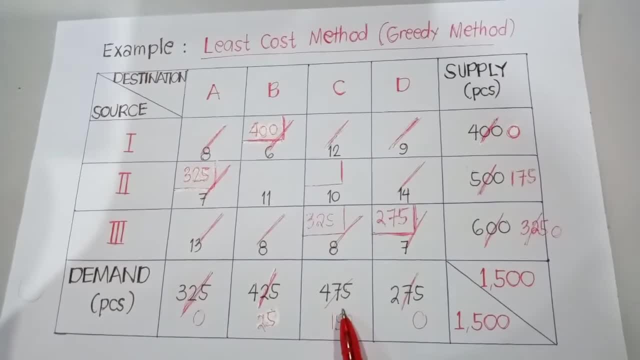 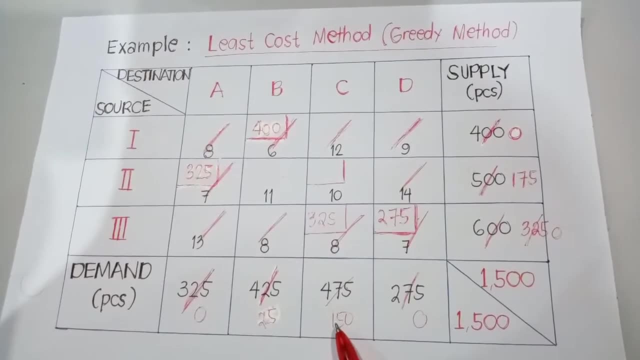 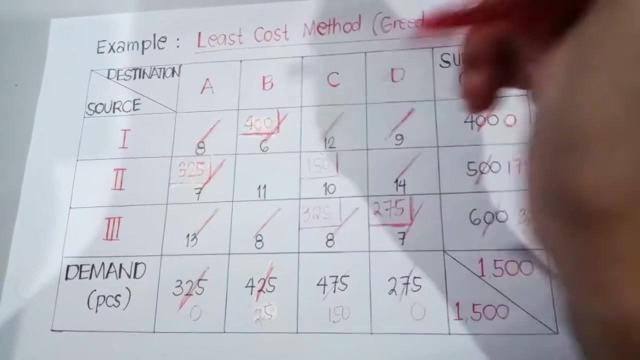 Now we will be matching again the quantity of our demand versus our supply. For our supply, we have 175.. And we have 150 for our demand. Now I will be using 150, since this has the least value. Okay. 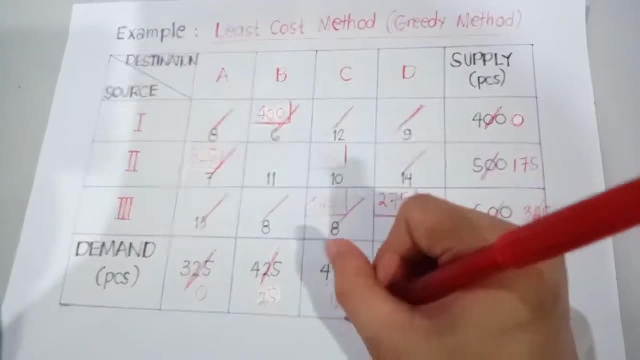 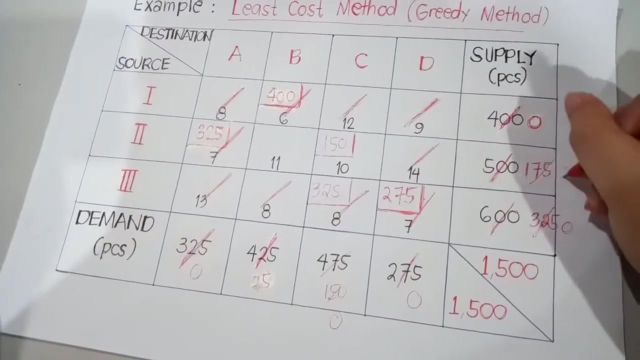 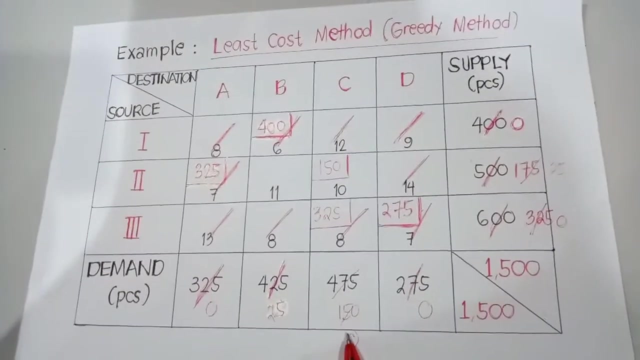 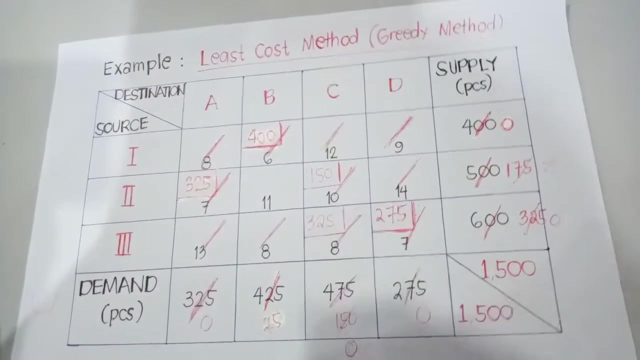 Now 150 minus 150, this becomes 0 now, And 175 minus 150, this becomes 25.. Okay, That's 25.. And therefore, since this has been exhausted already, we can now cancel out this entire row, because we will no longer be using this one. 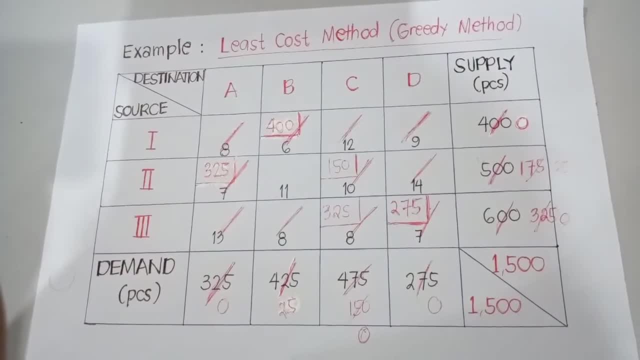 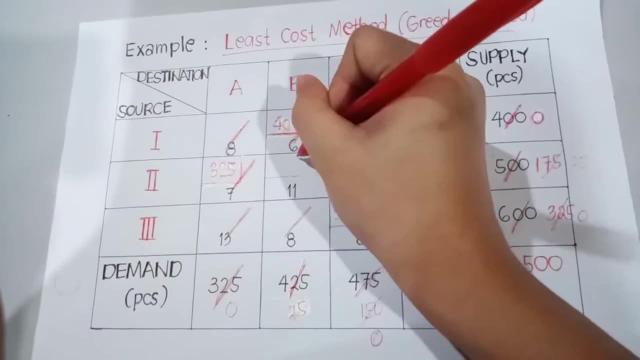 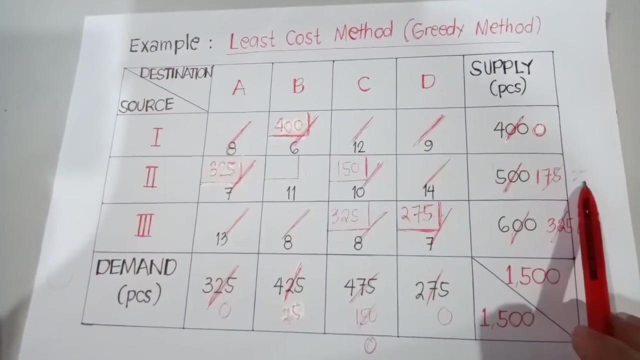 Okay, And now, finally, we are left with one cell, That would be cell number 11.. So we will be doing our last allocation here. Okay, Right there. And, as you can notice, each value of your demand and your supply is both 25 pieces. 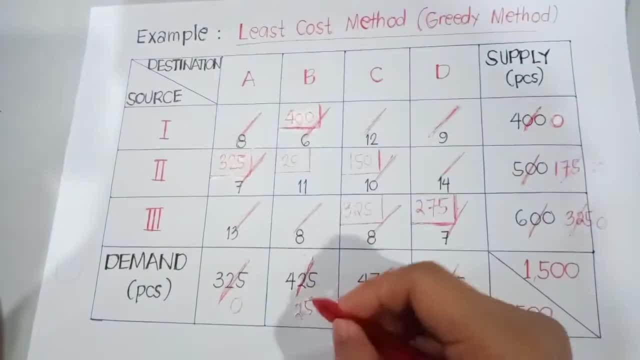 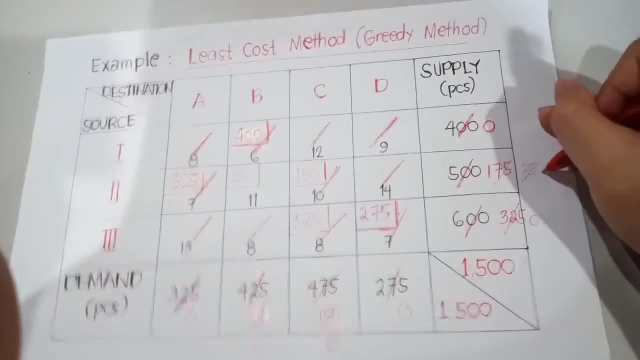 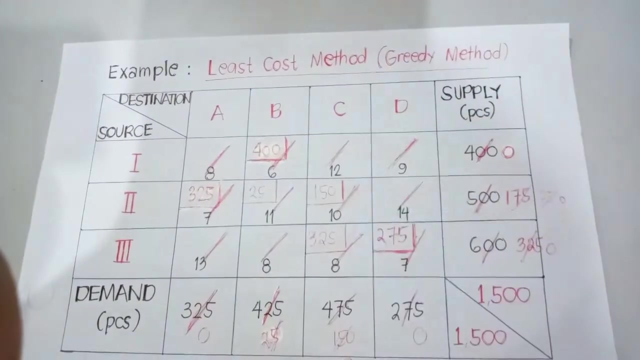 So you plug in 25 pieces here and both will be zeroed out. Okay, This will become 0. And this will be zeroed out as well. Okay, And since it has been zeroed out, all the cells now will be marked out. 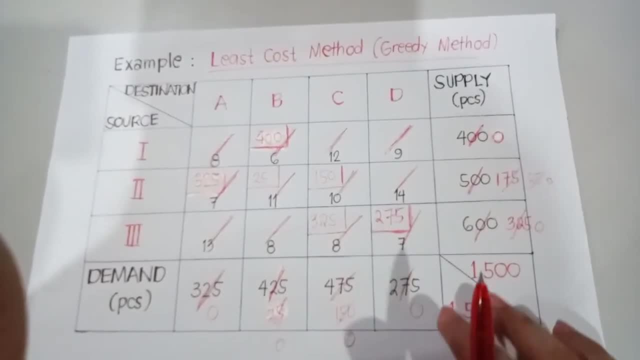 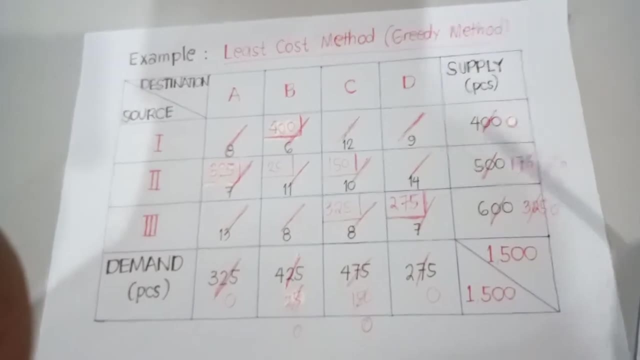 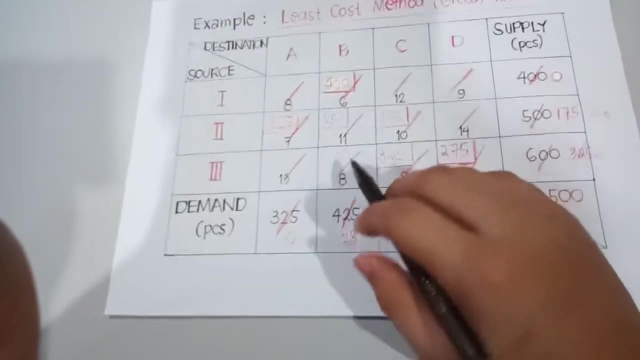 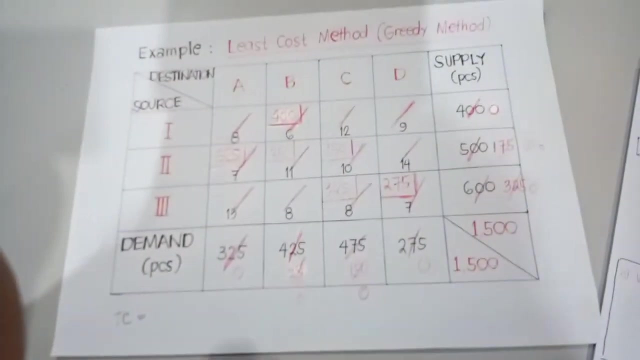 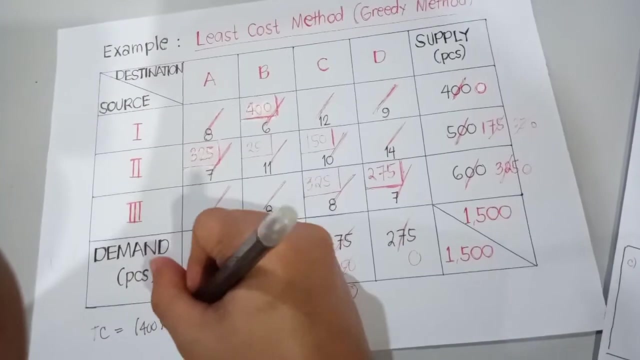 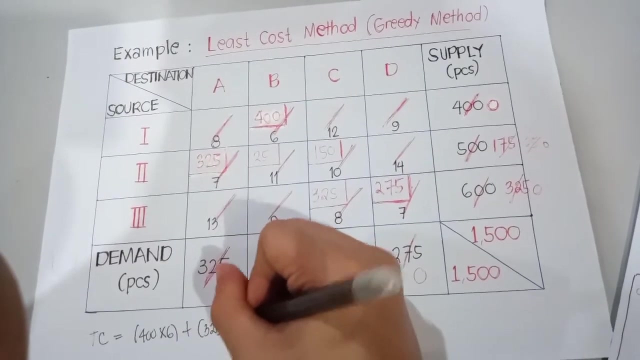 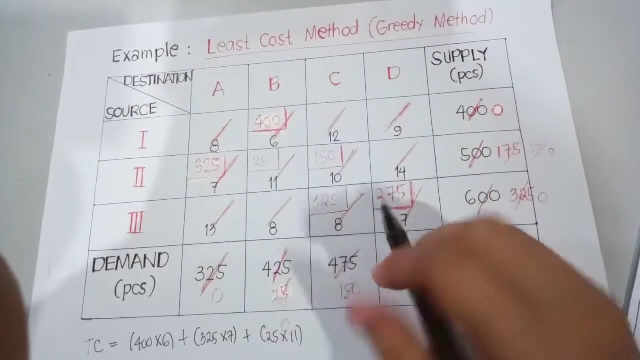 Okay, so that is how you do least cost method. Now, how do we compute, then, our total transportation cost for this one? Now, in doing so, we need to multiply the amount that we have allocated to each transportation cost. Now, in this manner, transportation cost would be equal to 400 times 6, so we have 400 times 6, plus you have 325 times 7,, 325 times 7, plus 25 times 11,, that's 25 times 11.. 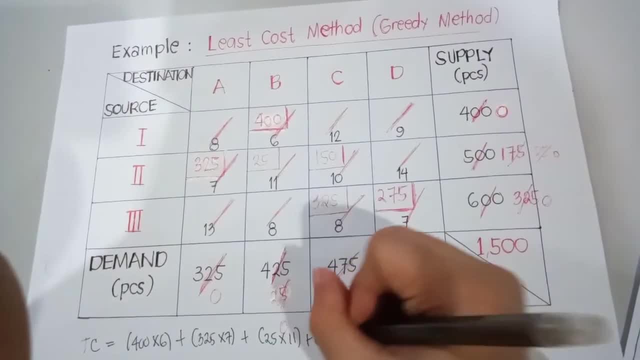 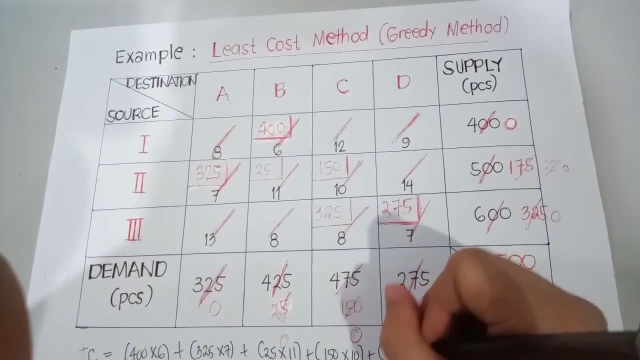 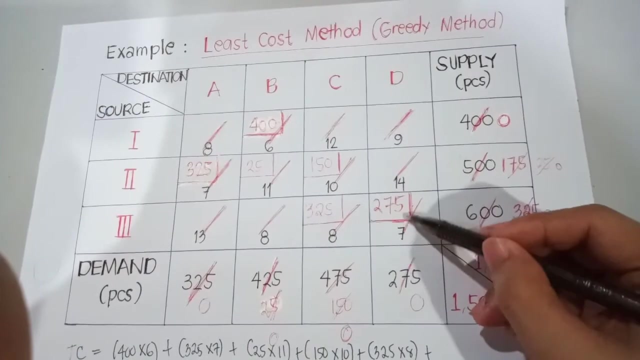 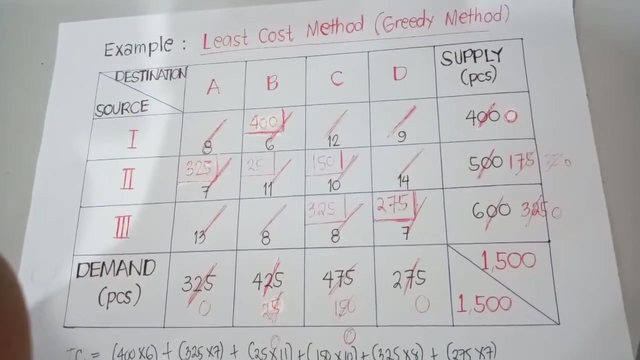 You have 152.. 150 times 10,, plus 150 times 10,, plus 325 times 8,, you have 325 times 8, and finally, you have 275 times 7,, so 275 times 7.. Now, in this case, our total transportation cost for our least cost method problem is: 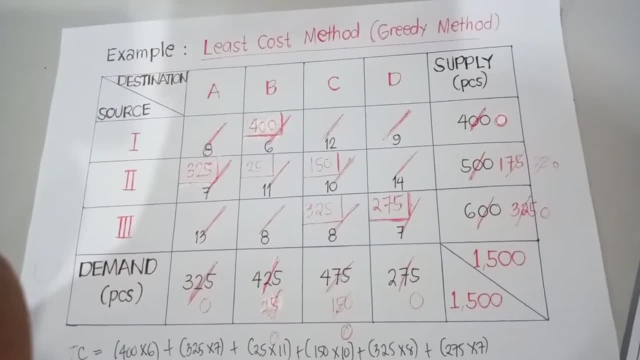 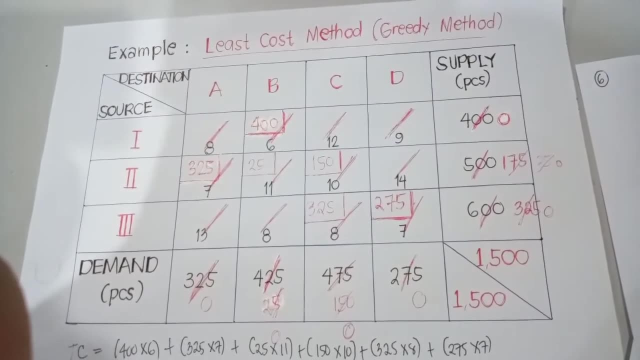 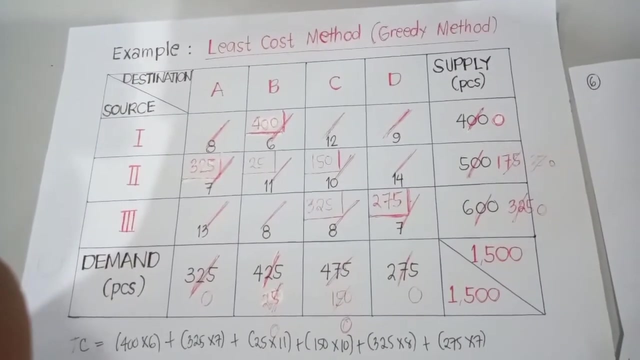 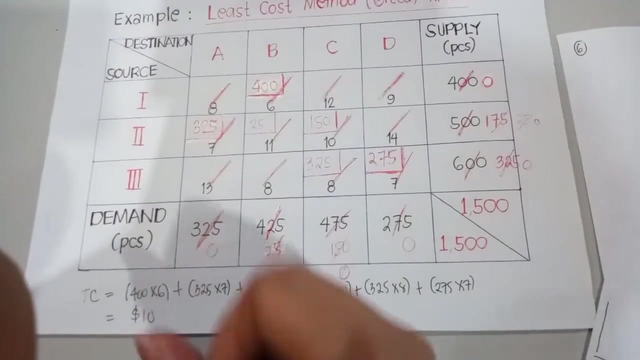 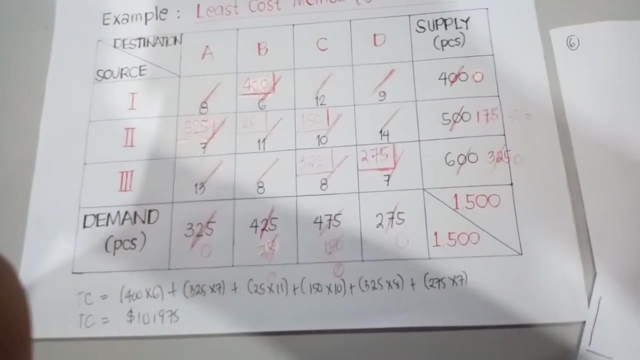 That would be amounting to how much? Okay, if you will try to calculate, that would be amounting to $10,975.. Okay, One more time, that's $10,975.. Okay, that will be our total cost. 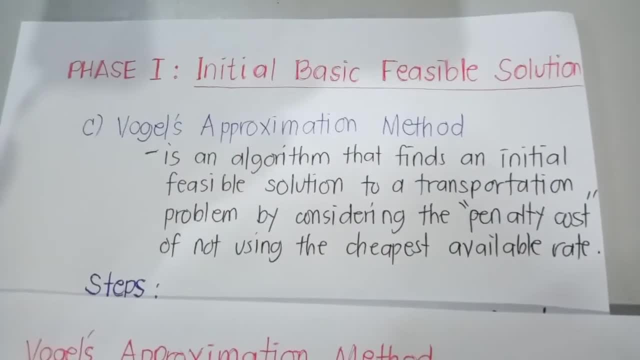 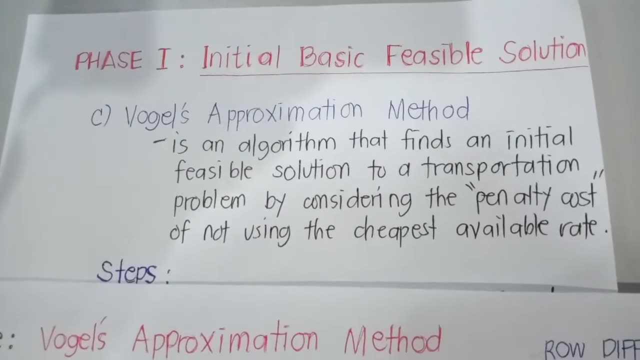 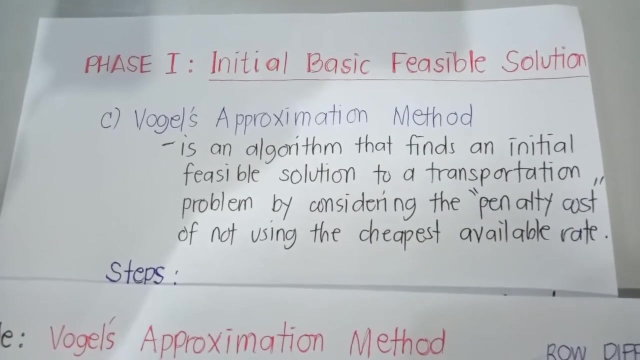 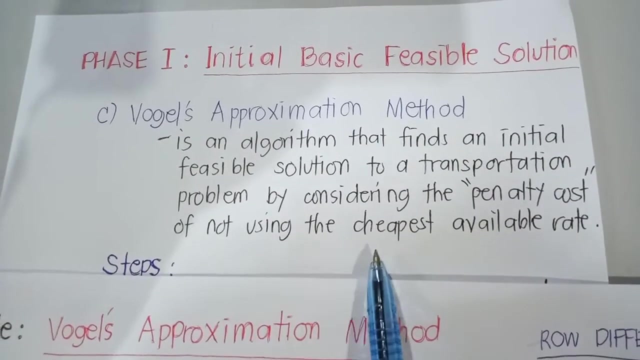 And finally, the last method that is used in establishing the initial basic feasible solution, that would be the Vogel's approximation method, or VAM. It is an algorithm that finds an initial feasible solution to a transportation problem by considering the penalty cost of not using the cheapest available. 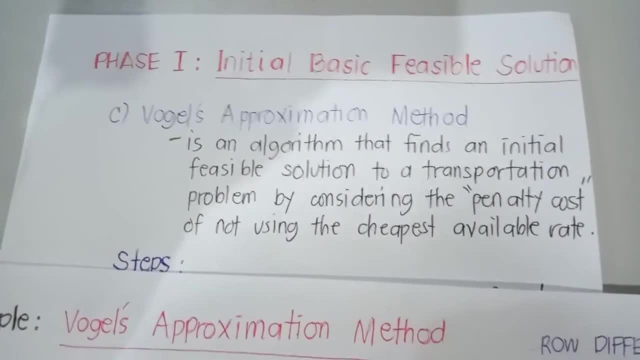 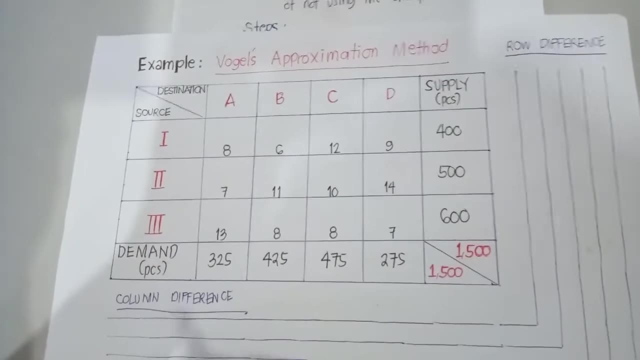 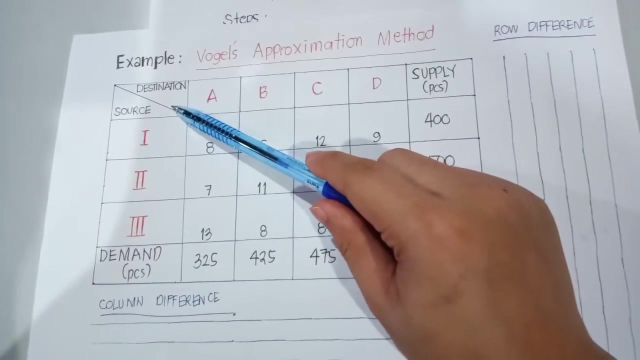 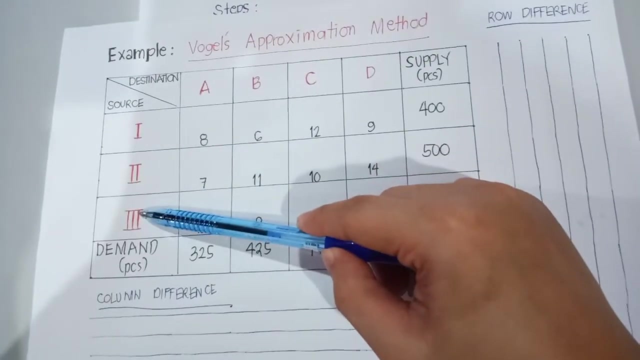 Rates. Now, in order for us to better understand this, let me show you an example Now. this example is quite similar to our previous methods, So we also have 3 different sources With respect to this source column. we have 1st source, 2nd and 3rd source, and we also have 4 destination sources. 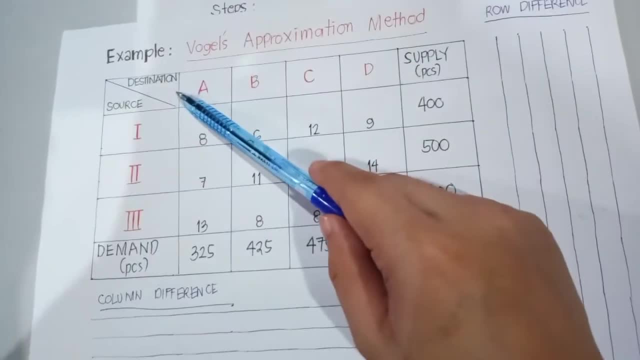 So at this point we already have 4 destinations. So what is the怎樣 condition of destination? The same as saying, when we create another variable, we have, We already have one destination and one destination. So to achieve this one destination, we will need to design one destination first. 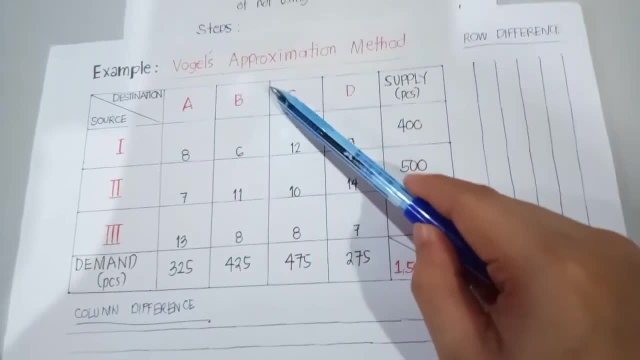 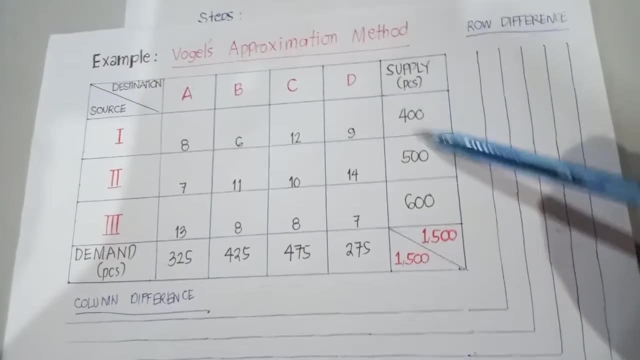 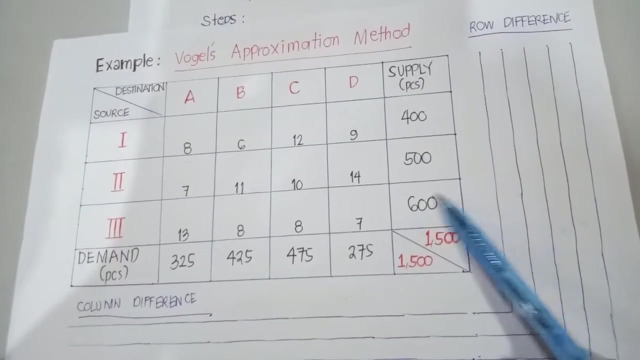 denoted with point A, point B, point C and point D respectively. We also have our column for our supply in terms of pieces and we also have row for our demand in terms of pieces And, as you can notice, this is also an example of a balanced transportation problem, because your total supply 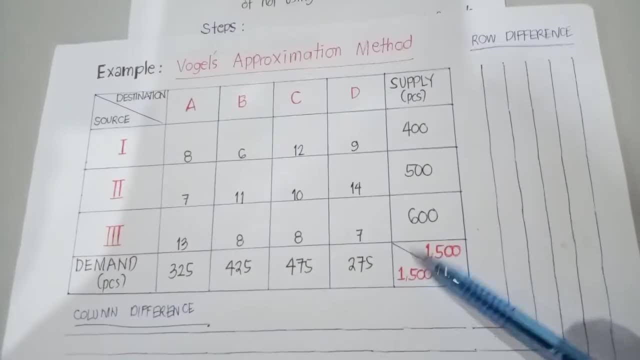 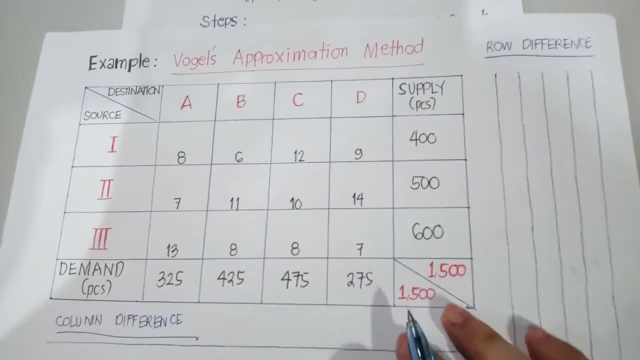 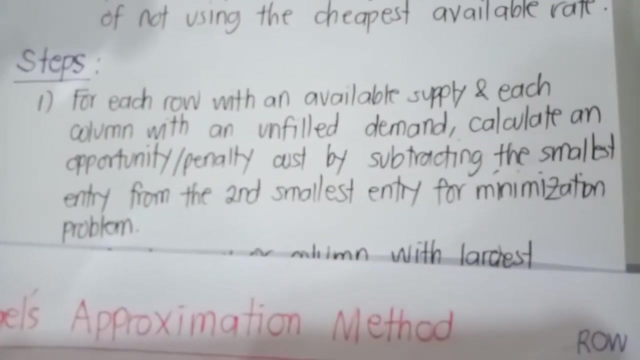 equals your total demand. Now for Vogel's approximation method. in order to do this, we need to strictly follow the different steps. Now let's discuss first step number one. Now, in step number one, it says: for each row with an available supply, each column with an unfilled. 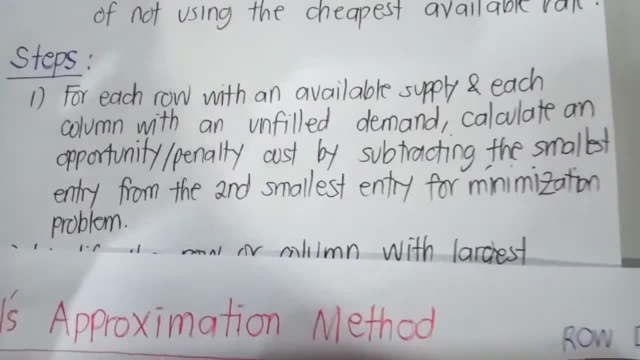 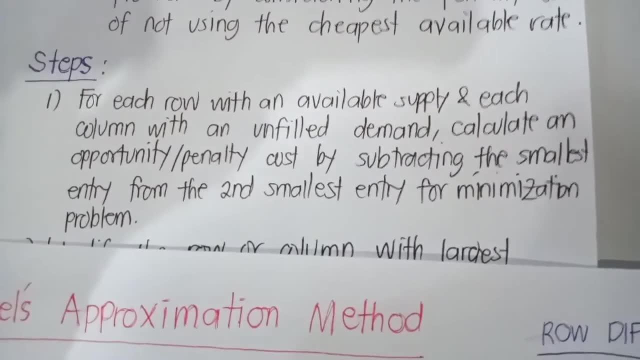 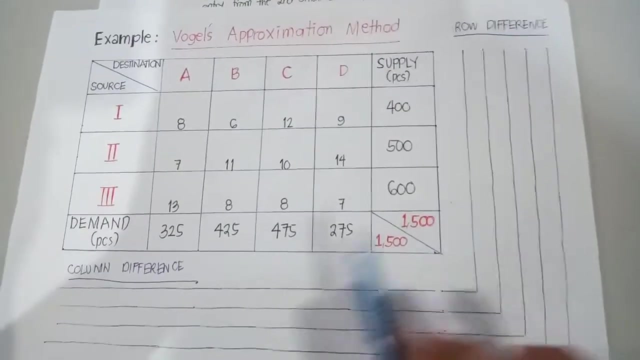 demand. calculate an opportunity or penalty cost by subjecting the supply to the supply, The smallest entry from the second smallest entry for minimization problem. Now, as you can notice, we have what we call row difference and we also have what we call column difference. 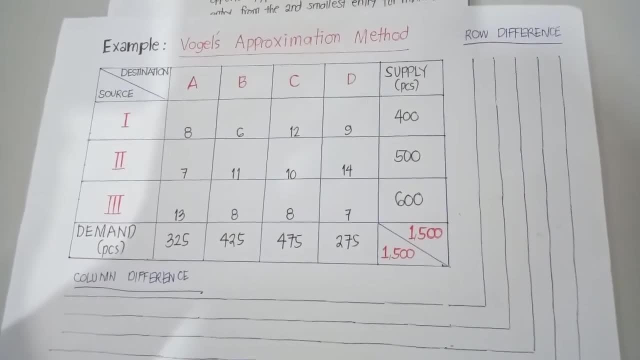 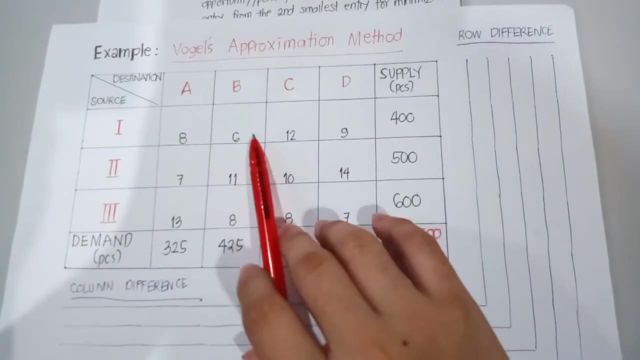 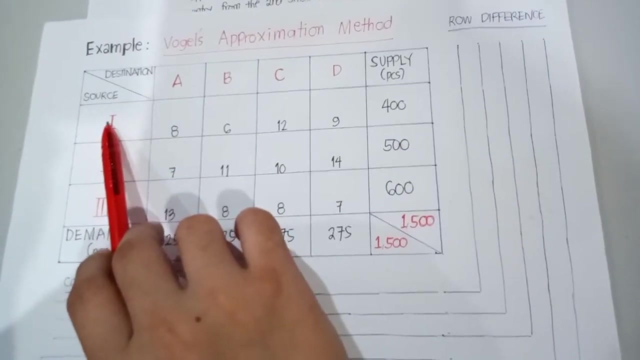 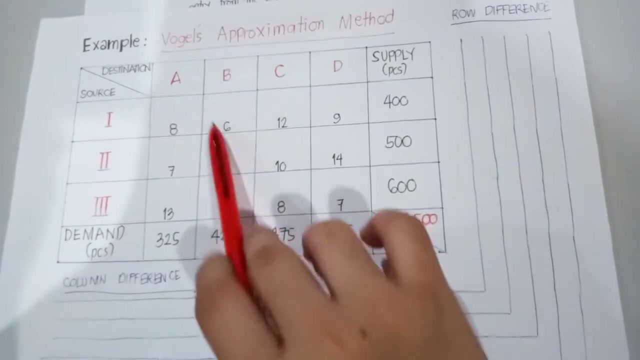 Now, in this case for step number one, we will do the row difference first. So in doing the difference, we need to identify the amount with the least cost. So in terms of row one or source one rather. so the least cost is six. and once we had already identified our least cost, 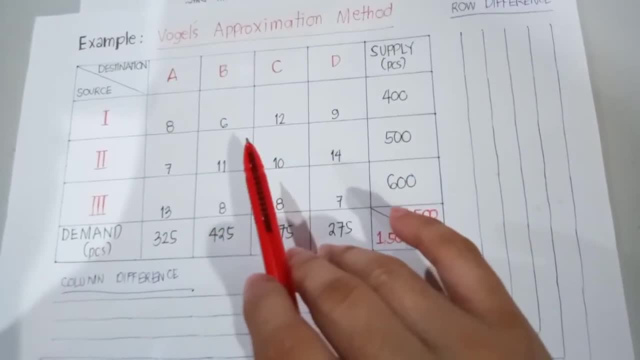 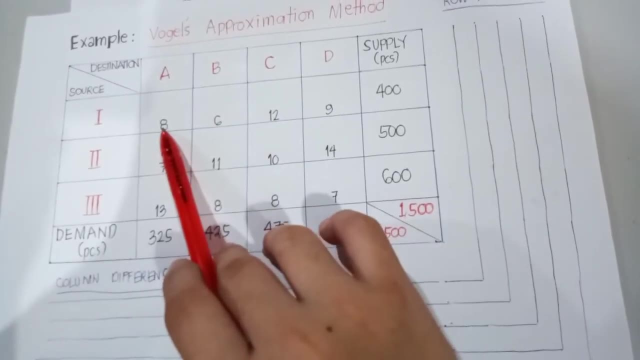 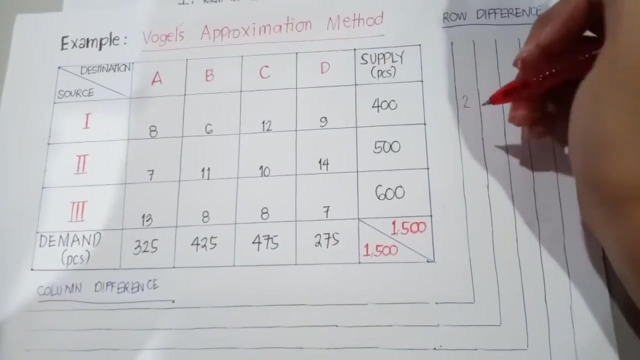 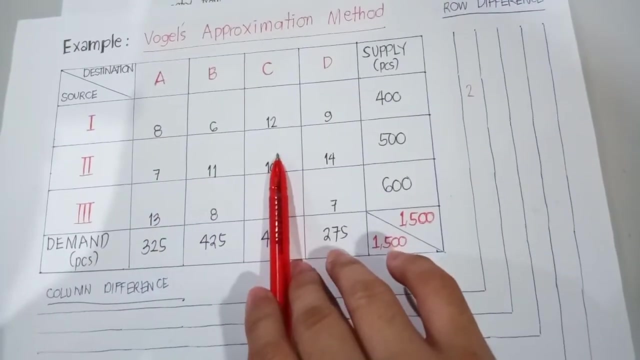 we need also to identify the second least cost. now, in this instance, we have six as the least cost and the second least cost is eight. so therefore, eight minus six, that will be two. okay, that's two. and for the second row, our least cost is seven and our second least cost is ten. so ten minus seven. 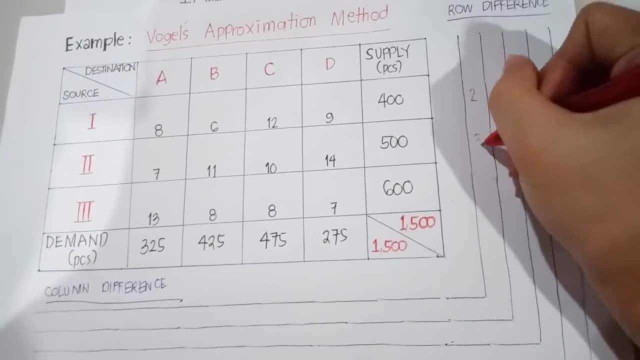 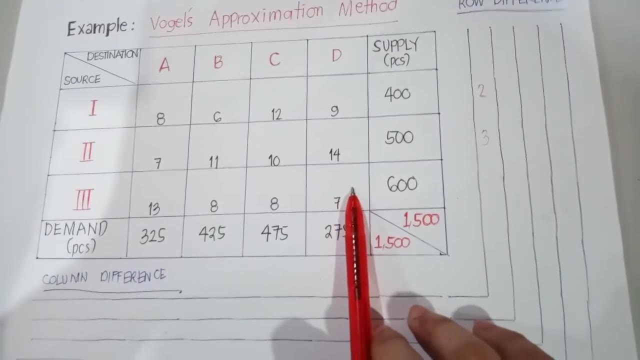 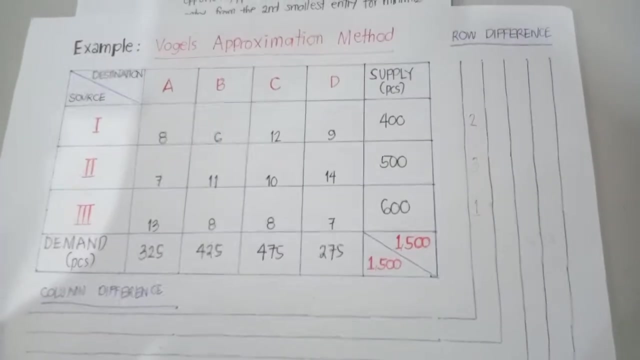 we got a difference of three for the third row. our least cost is seven and our second least cost is eight. so therefore, our difference is one and finally, we are done with row difference and right now we will go to the second row and we will go to the third row and we will schedule a list of 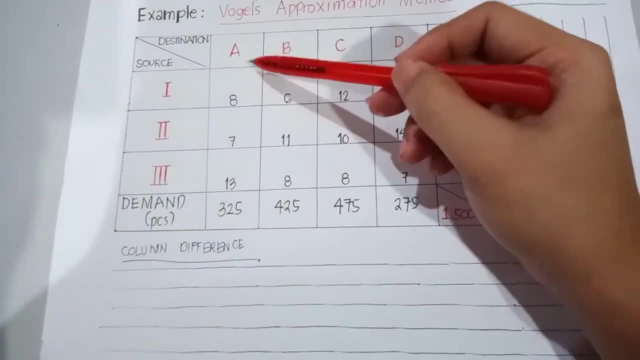 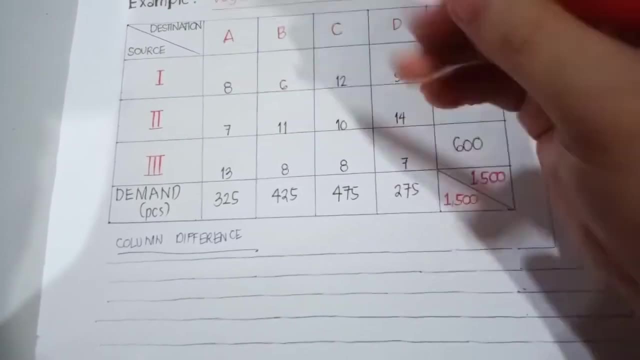 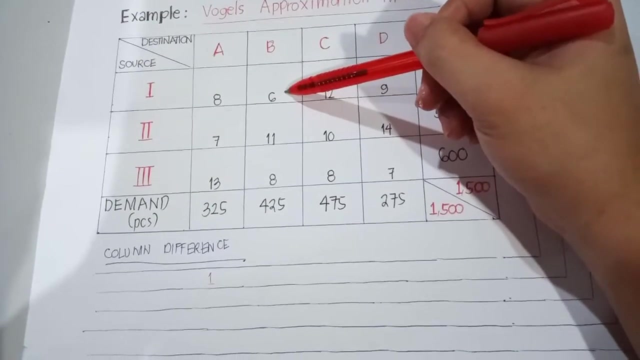 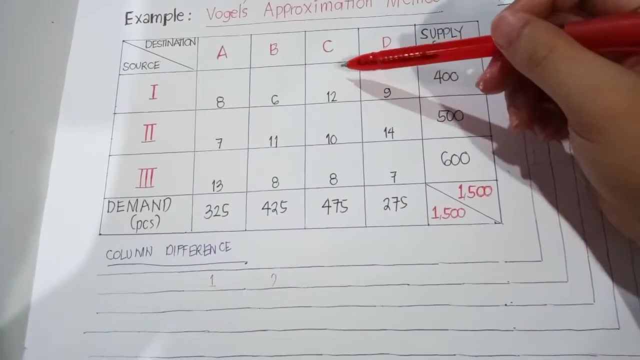 to our column difference. so, in terms of column a, our least cost is seven and our second least cost is eight. so eight minus seven, we have a difference of one. in terms of column b, we have least cost of six, followed by eight. so eight minus six, that would be two. for column c, we have eight as the 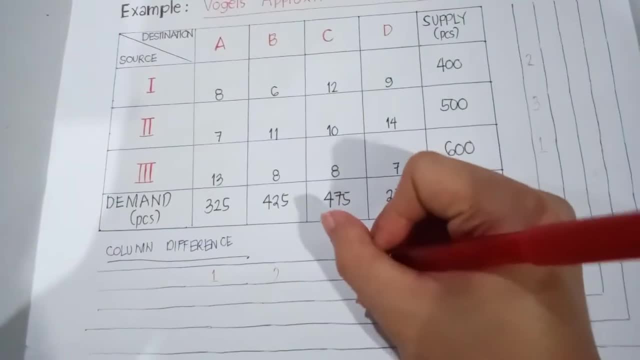 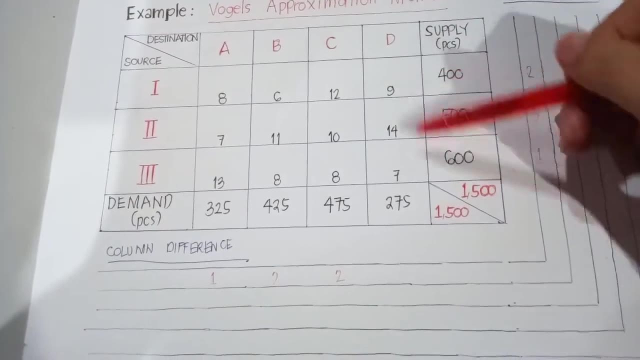 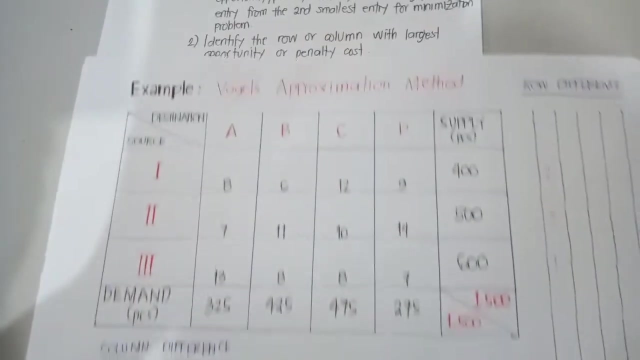 least cost, followed by ten. so ten minus eight, we have two. and for the last column, the least cost is seven, followed by nine. so nine minus seven is two. okay, that's step number one. now what's step number two? so for step number two, we need to identify the row or column with the largest. 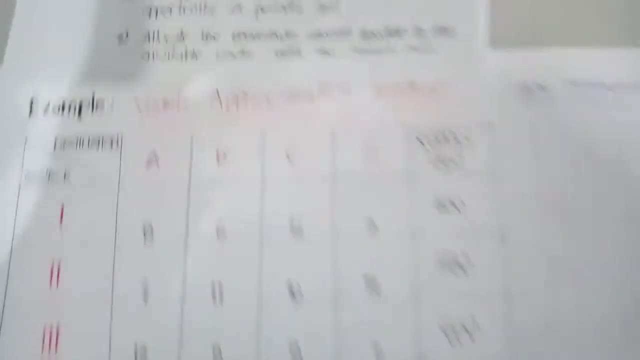 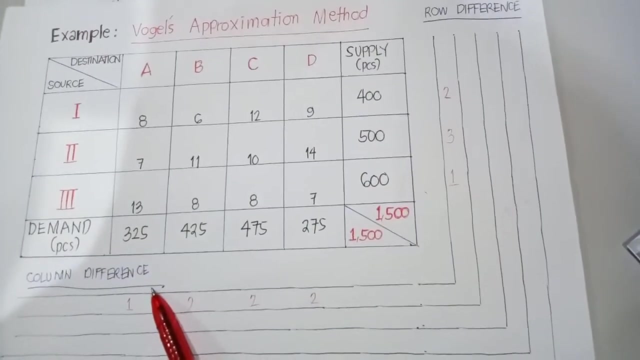 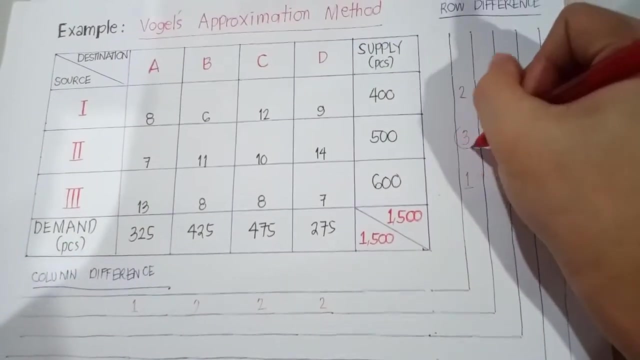 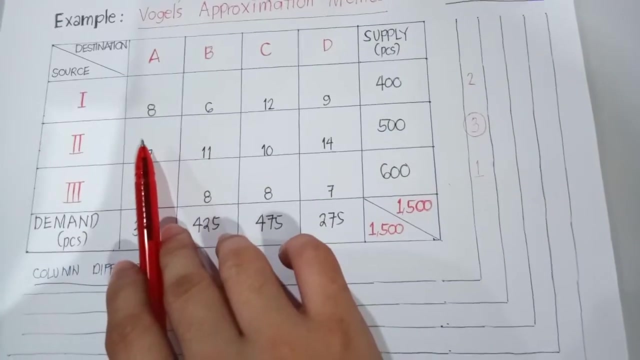 opportunity or penalty cost. now, as you can notice here, based on our row difference and column difference, we need to select the one with the largest value. so the largest value is three and therefore, this three right here is under our row two. right, this is under row two. now, since this is under row two, we need to find: okay, let's read first: 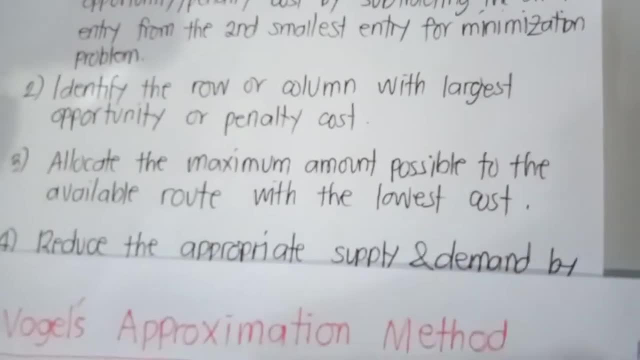 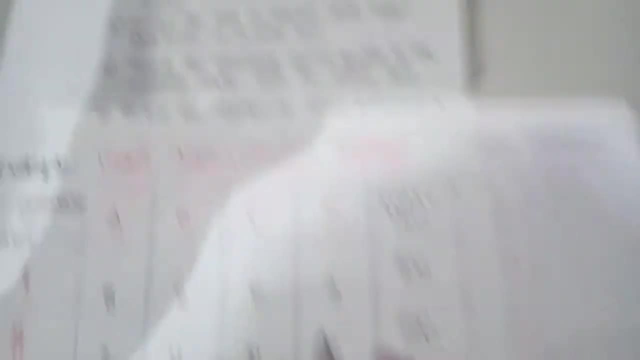 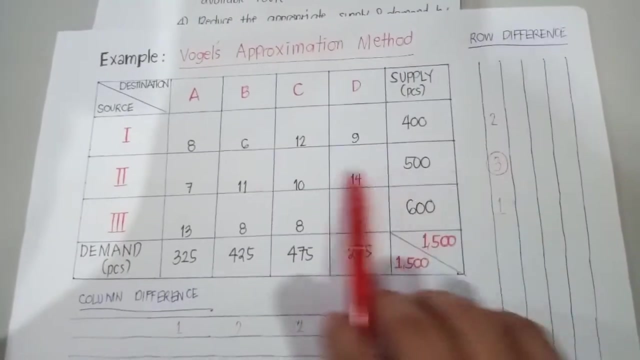 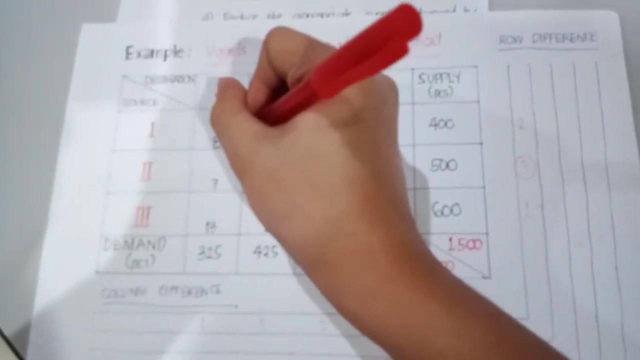 step number three. for step number three, we need to allocate the maximum amount possible to the available route with the lowest cost. so therefore, in step number three, we need to identify the lowest cost under row two. so the lowest cost is seven, right? so therefore, this is where i will be doing my first allocation and in doing so, 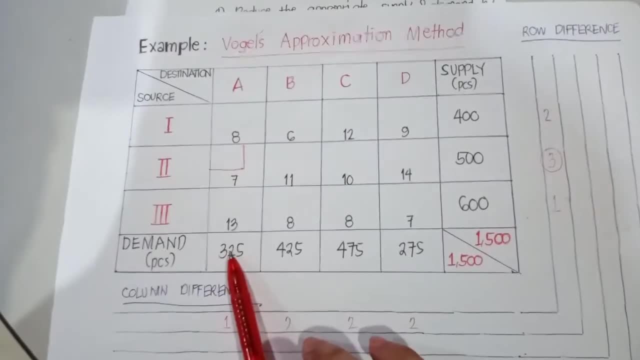 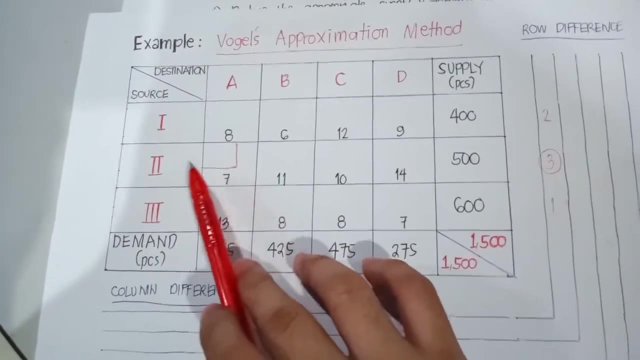 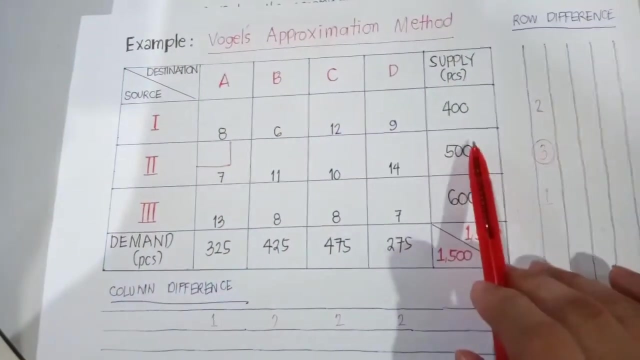 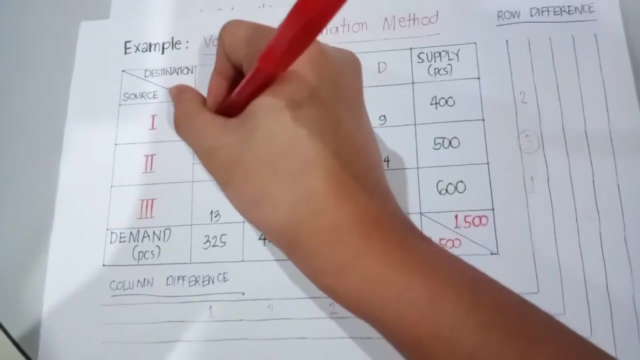 i need to match the quantity of my demand versus the quantity of my supply now, with respect to my cell source to destination a. so the quantity of my demand is 325 and the quantity of my supply is 500, and therefore, since 325 is the least value, then i will be. 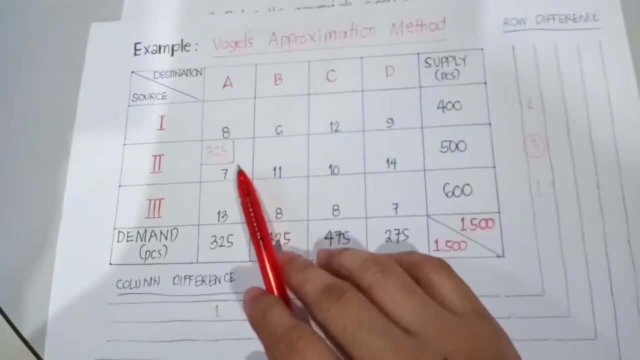 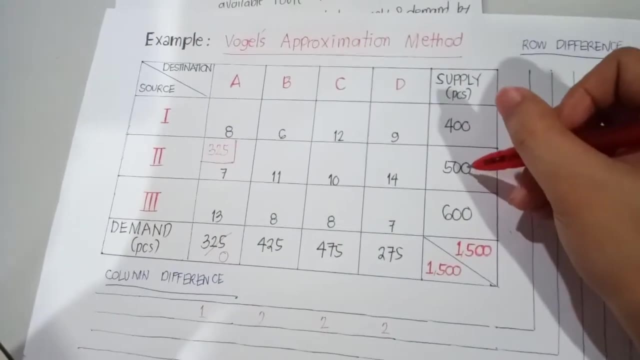 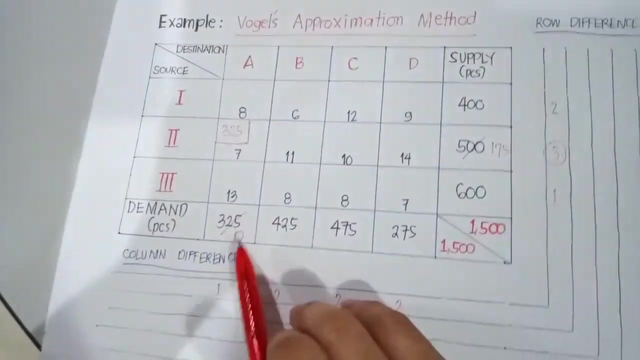 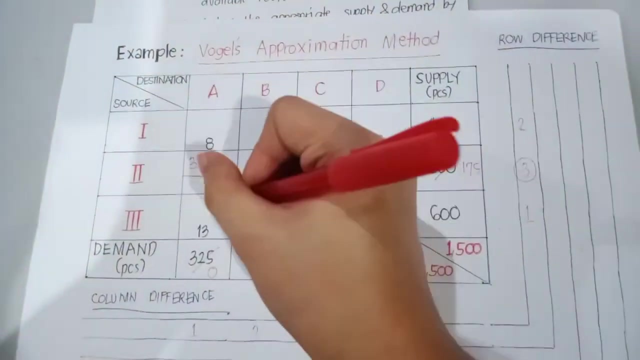 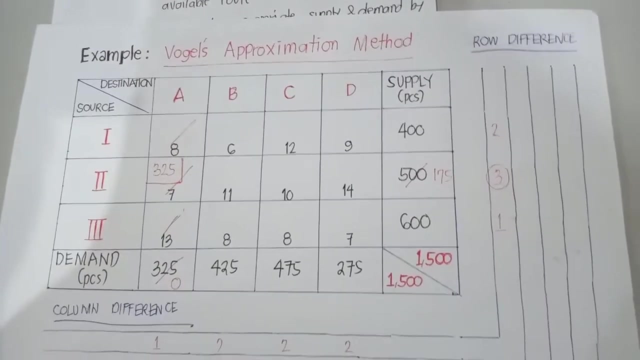 using this one for my allocation. so 325 minus three to five, this becomes zero, and 500 minus this becomes 175. now, since this has been satisfied already, this has been exhausted. therefore, we are now able to cancel the entire column. okay, we will be marking that out because we will no. 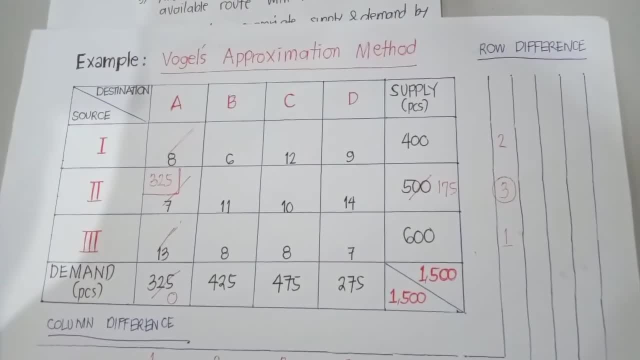 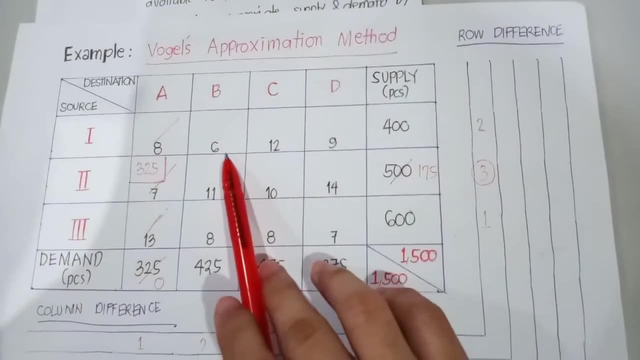 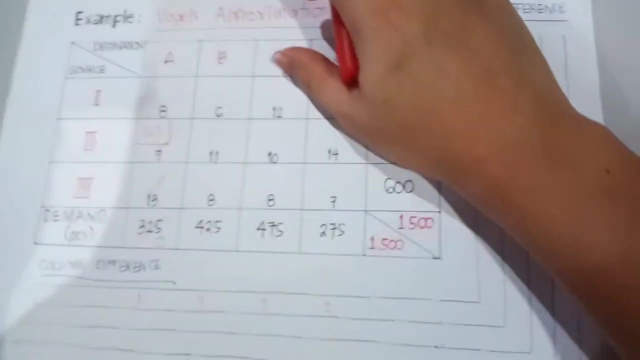 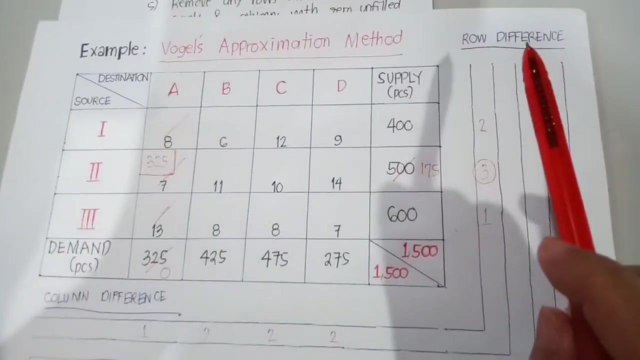 longer be making use of that column now, since we have marked that out already. we are now left with three columns. we have columns b, c and d, and the next step that we need to do is to follow steps one and two. so we need to do the row difference and column difference again, so with 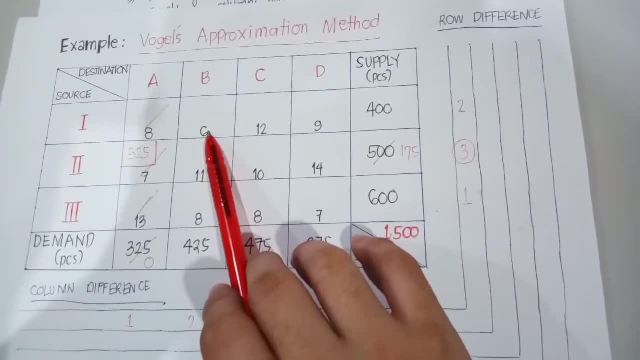 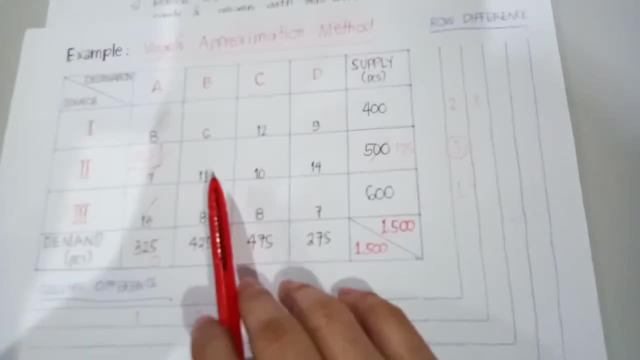 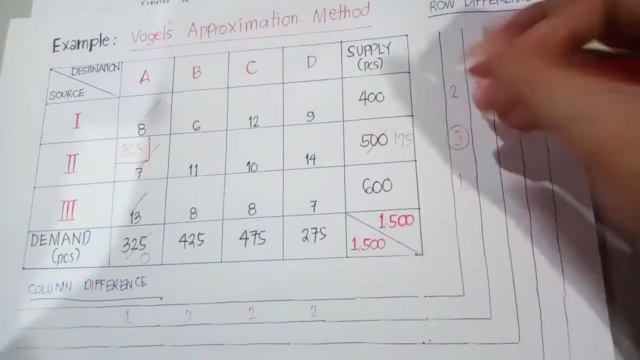 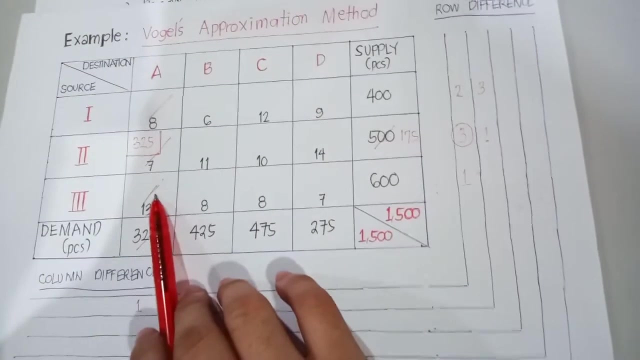 respect to row one, my least cost is six, followed by nine, so therefore nine minus six, my difference is three. with respect to my row two, my least cost is 10, followed by 11, so therefore my difference is one. okay. and next, with respect to row three, my least cost is seven, followed by eight, so therefore my difference is: 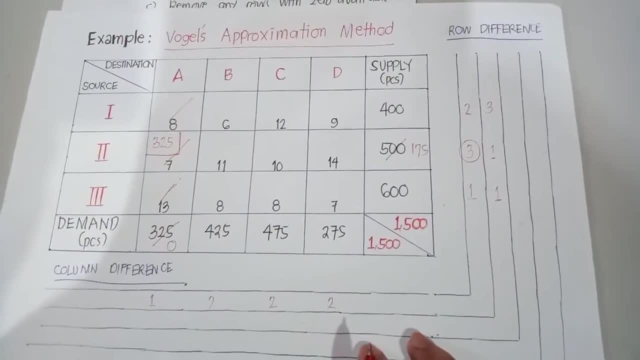 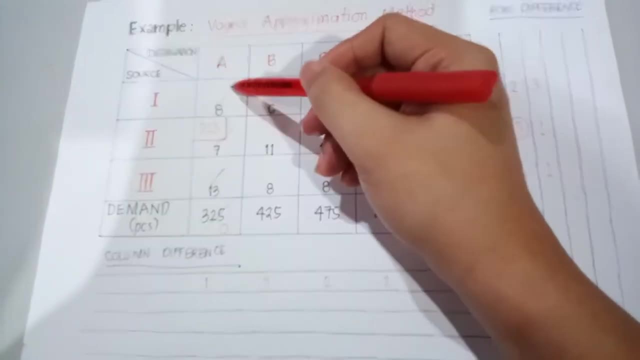 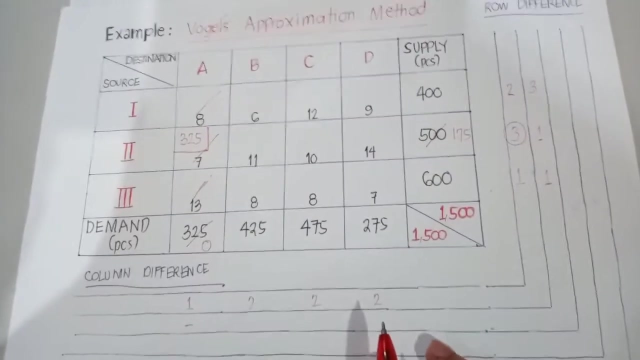 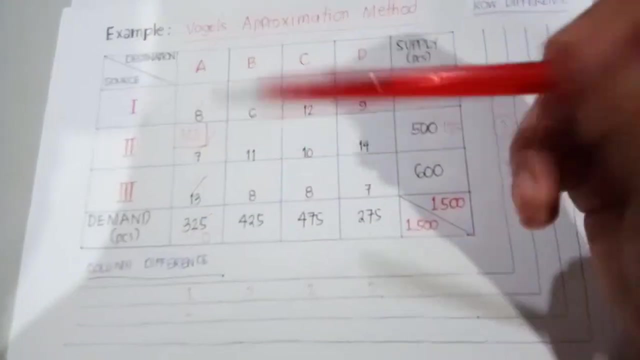 one. okay, that's with respect to row difference. what about in column different? now for column different. since this has been canceled out or marked out already, we will just simply put hyphen okay, because this is no longer applicable. so, in terms of column b, my least cost is six, followed by eight. so therefore my difference. 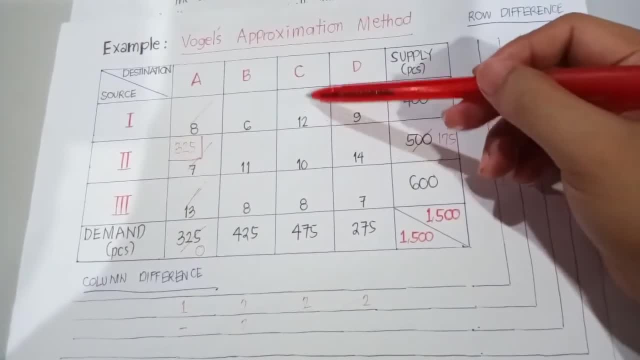 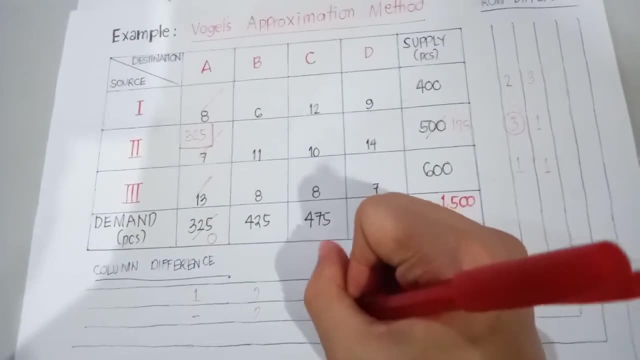 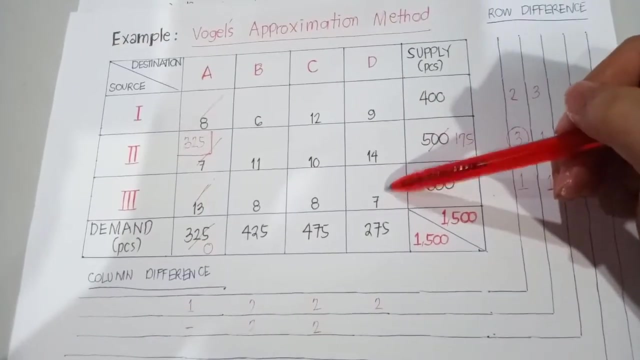 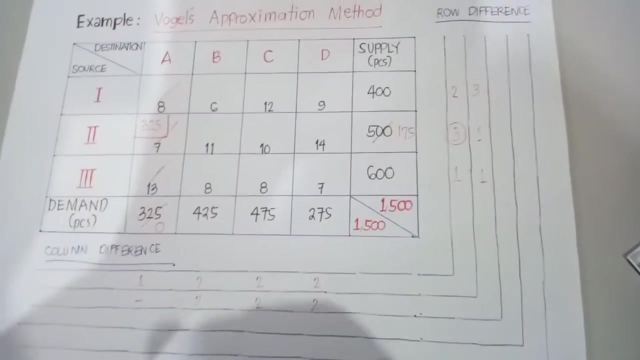 is two, and with respect to column c, my least cost is eight, followed by 10, so therefore i have two as my difference. and with respect to my column d, my least cost is seven, followed by nine. so therefore my difference is two, and again we will need to select the value. let's 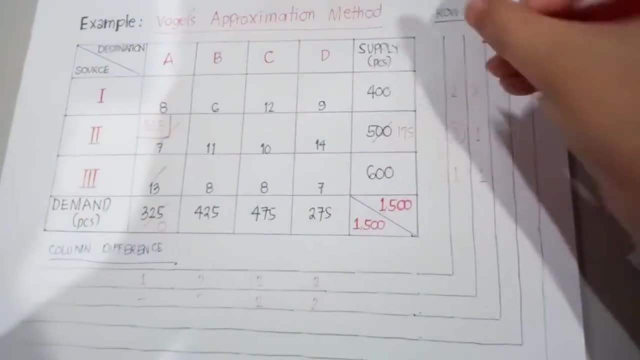 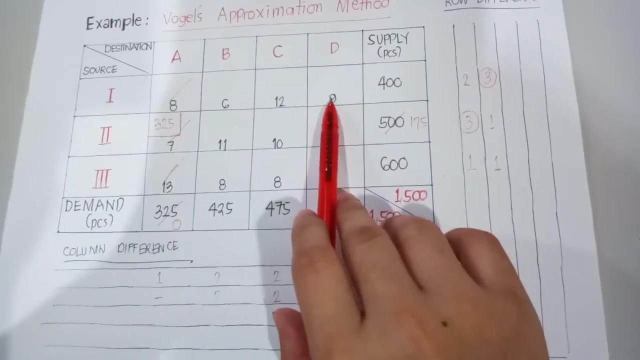 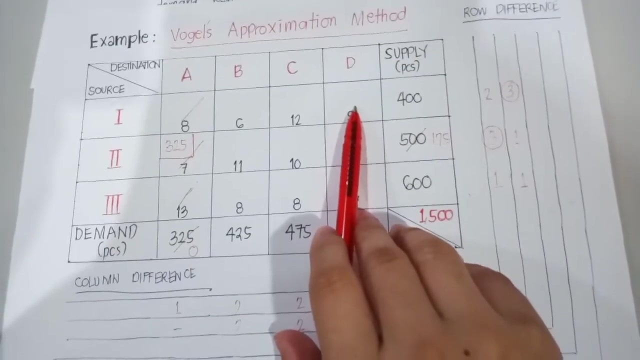 consider as the largest. so, in this case, our largest value is three, and three is under what row? it's under row one. so, since it's under 1, we need to select the cell that has the least cost, and that would be this cell because it has the least cost. so, therefore, i will be doing my next. 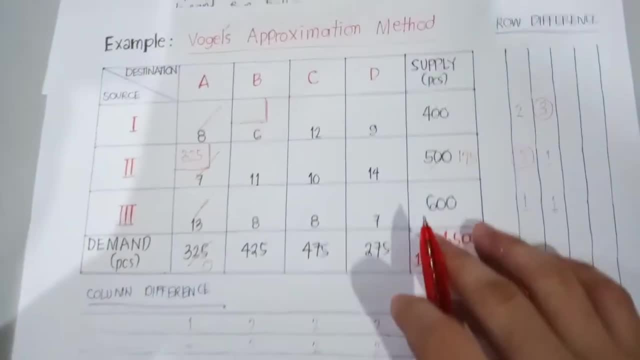 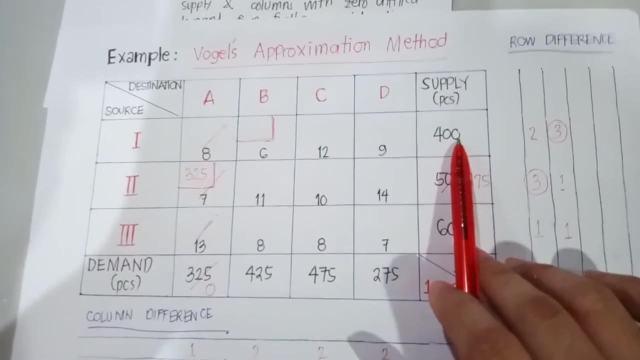 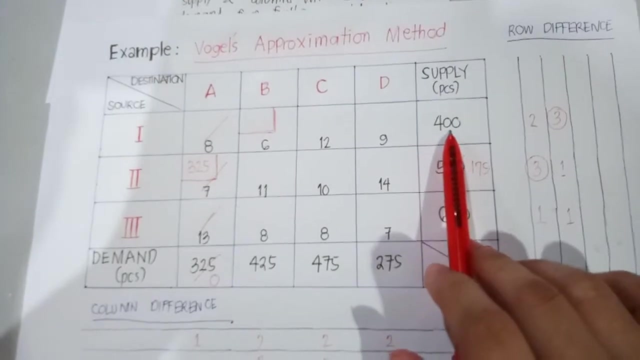 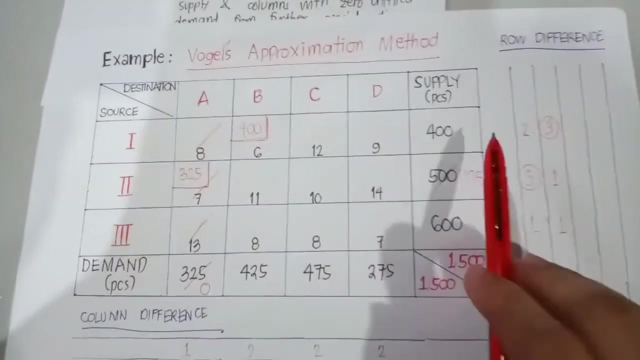 allocation right here, and in doing so i need to match again the quantity of my demand versus the quantity of my supply. in this case, my supply is 400 and my demand is 425, and therefore i will be allocating in 400, since this has the least value. okay, so i will be plugging in 400, therefore 400. 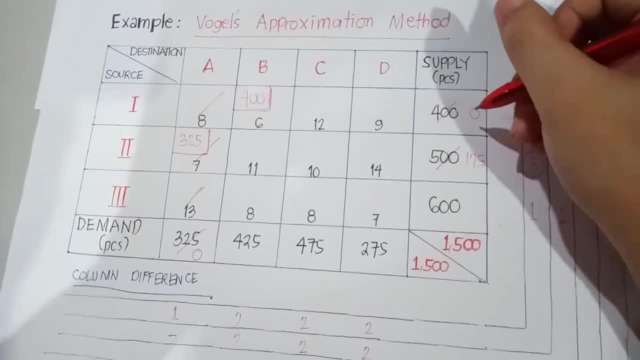 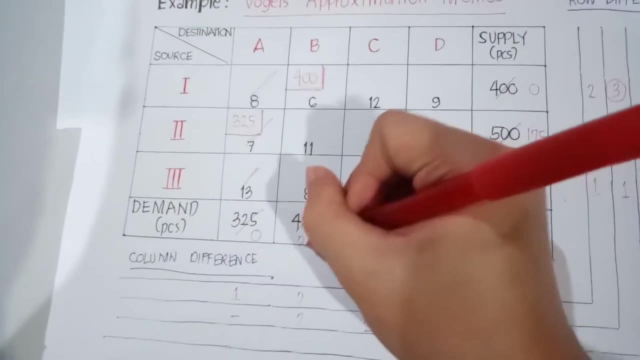 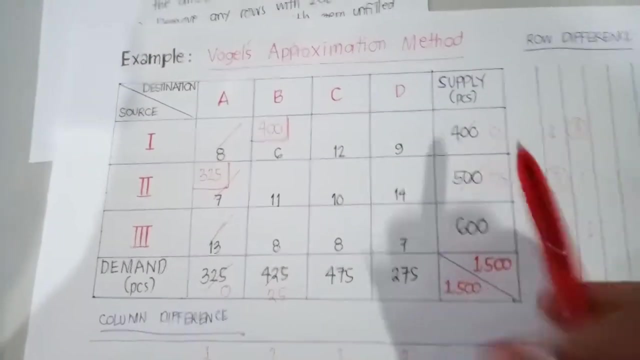 minus 400, this becomes zero. okay, this will be zeroed out. and 425 minus 400, this becomes 25. okay, now, since this has been zeroed out already or exhausted, we can now finally mark this out. okay, now, since this has been zeroed out already or exhausted, we can now finally mark this out. 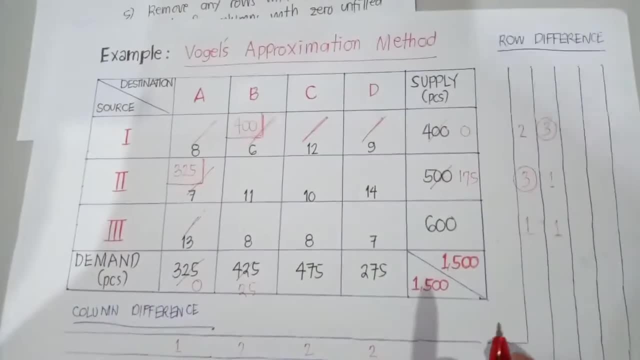 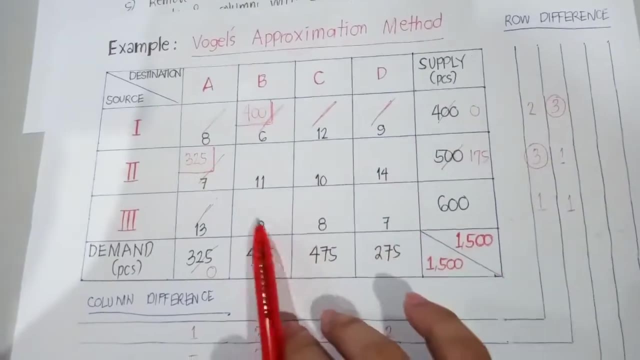 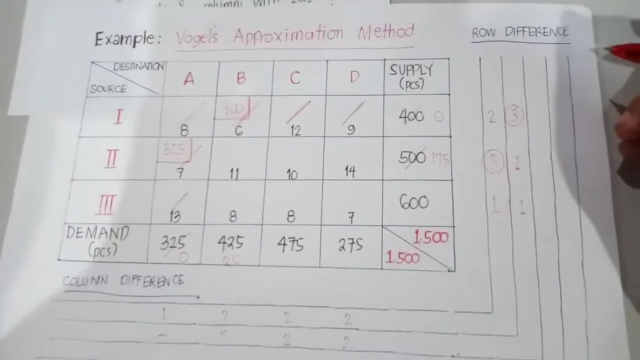 okay, we will no longer be using this row. by marking that out, we are now left with these cells. okay, we have cells 11, 10, 14, 8, 8 and 7. now we will do with the previous steps. so we need to do the row difference again and the column difference now at this point. 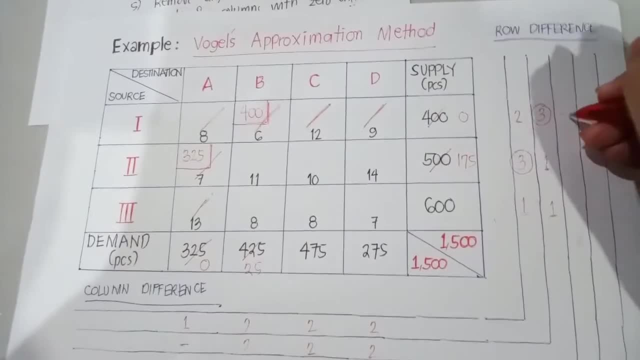 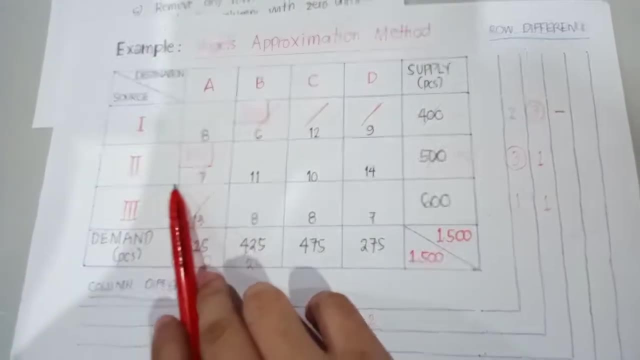 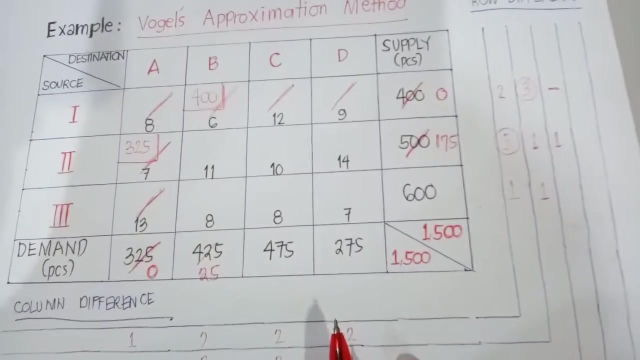 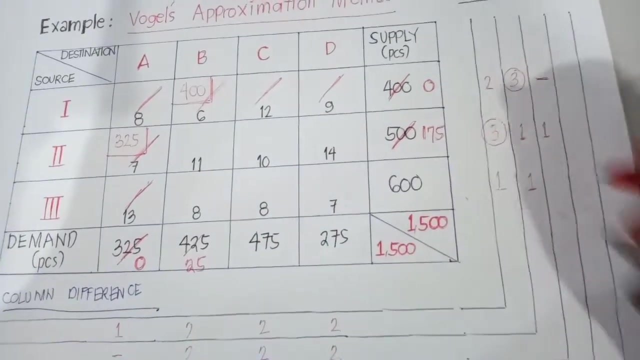 in here. this is no longer applicable, so just put in hyphen because this is already marked out. with respect to my row 2, my least cost is 10, followed by 11, and therefore my difference is 1. and with respect to my row 3, my least value is 7 and followed by 8, and therefore 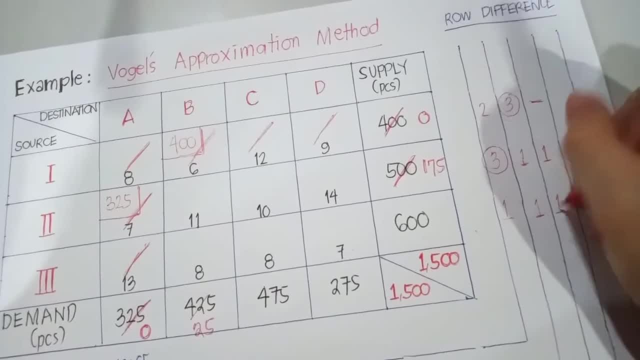 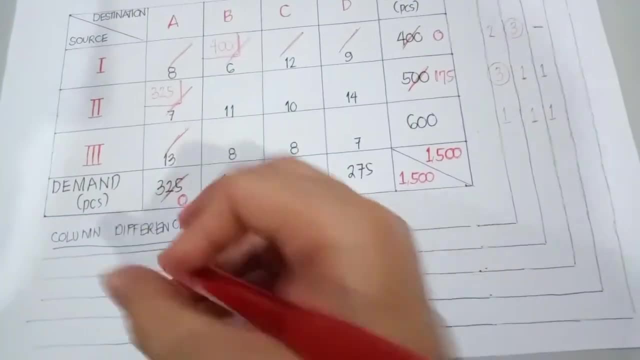 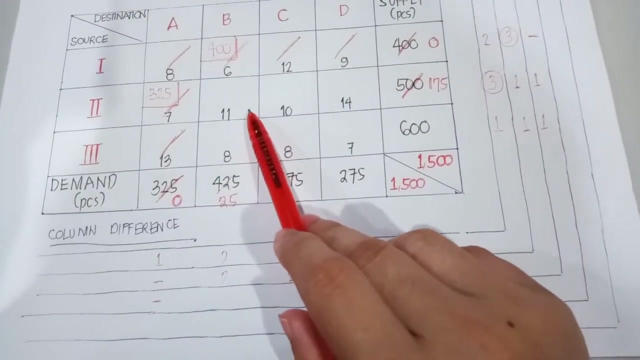 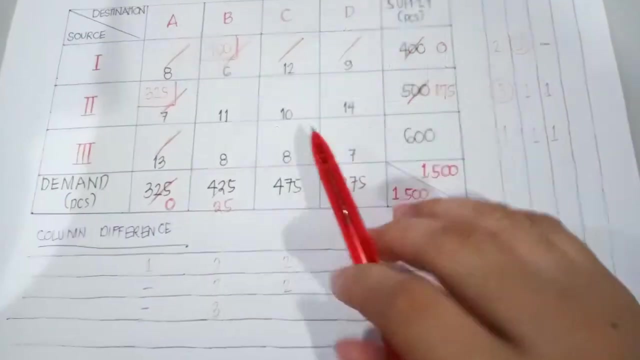 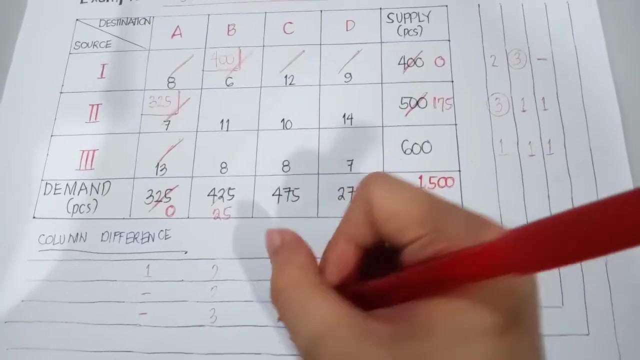 my difference is 1. and moving on to column difference, so with respect to my column a, that's no longer applicable for column b, so my least is 8, followed by 11, so therefore my difference is going to be 3. okay, that's 3. for column c, that's 8, followed by 10, so therefore my difference is 2. 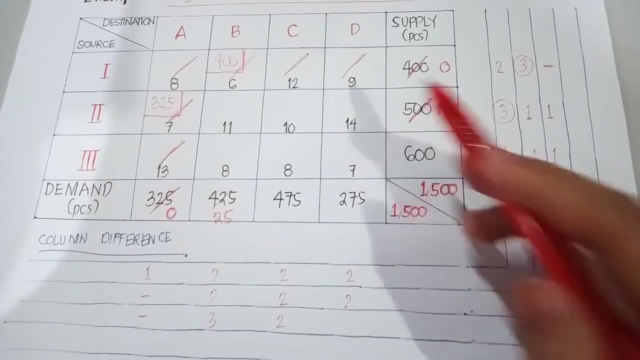 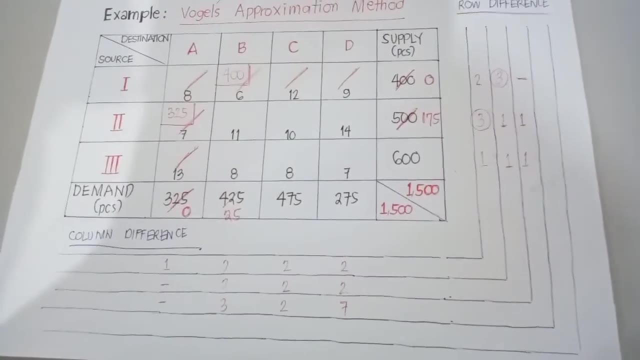 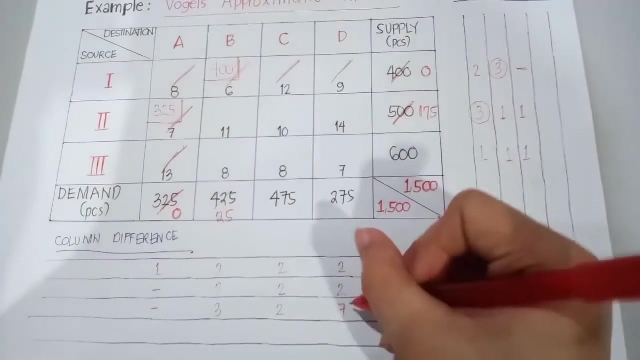 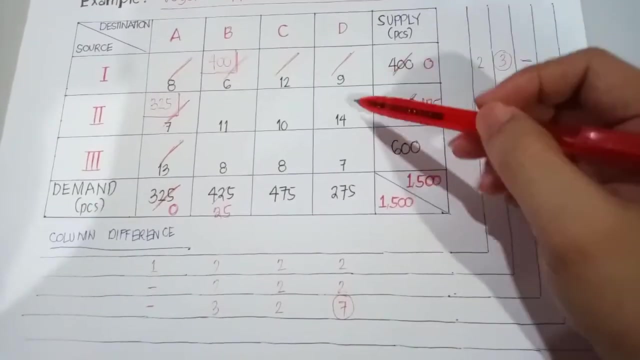 i have 7 and 14, so therefore my difference is 7, and next step is we need to be able to select the largest value, and the largest value among our row and column difference. that would be 7, and 7 is under column d, so therefore in column d and we will consider. 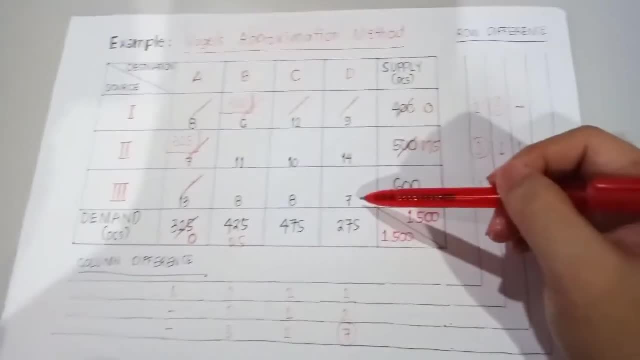 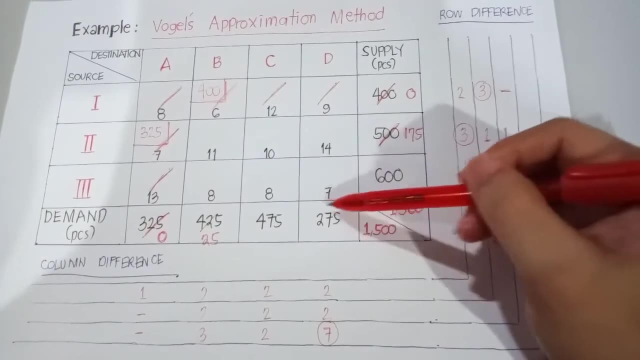 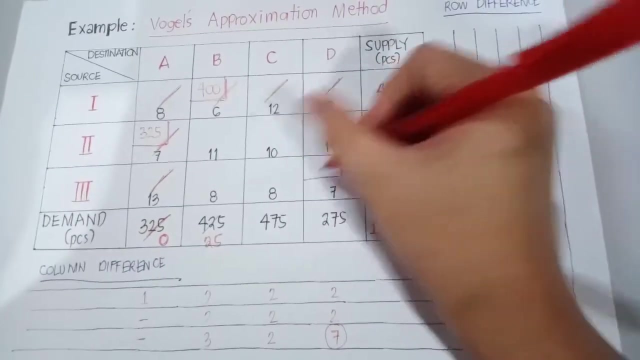 these two cells, 14 and 7, and we need to select the cell that has the least cost value and therefore we will be doing our next allocation right here, because 7 has the lowest value. okay, so in doing my allocation again, i will be matching the 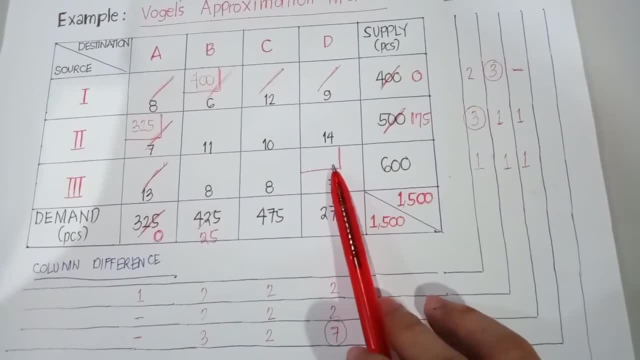 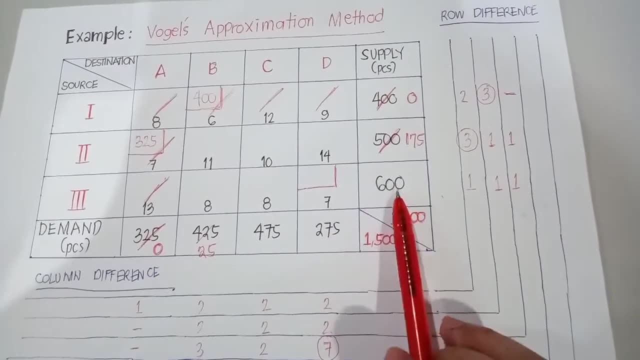 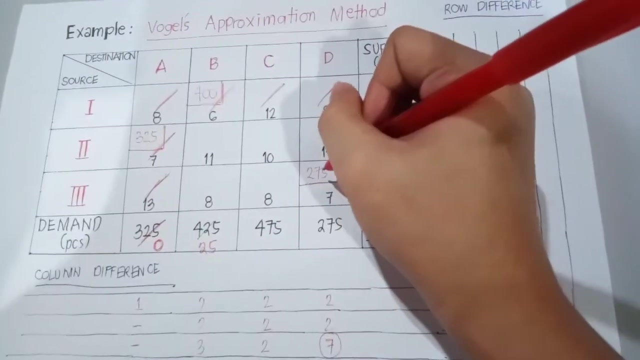 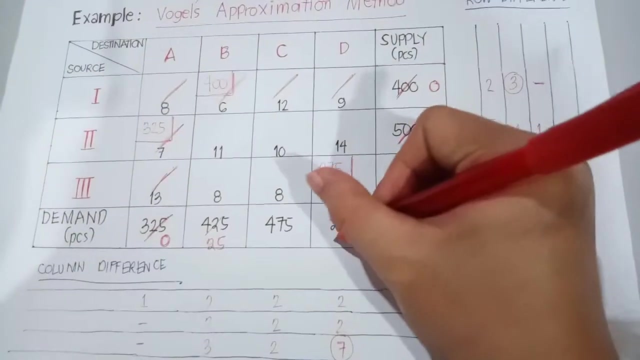 quantity of my demand versus my supply. so, with respect to my selected cell, the quantity of my demand is 276 and the quantity of my supply is 600. so therefore i will be plugging in 275 right here, because this has the least value. so 275 minus 275, this becomes zero. it will be zeroed out and 600. 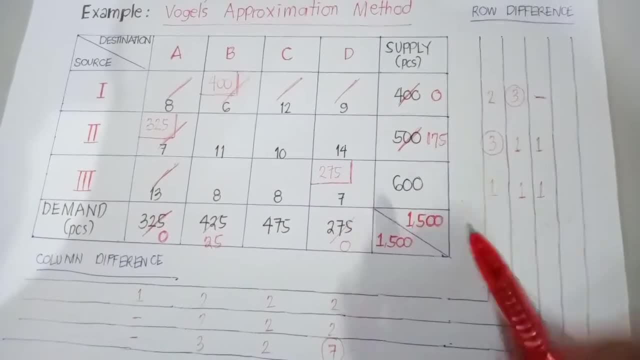 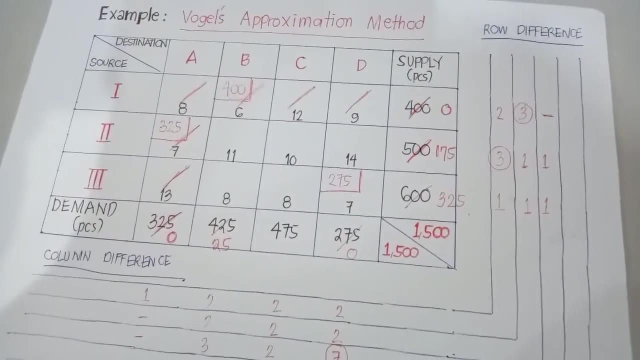 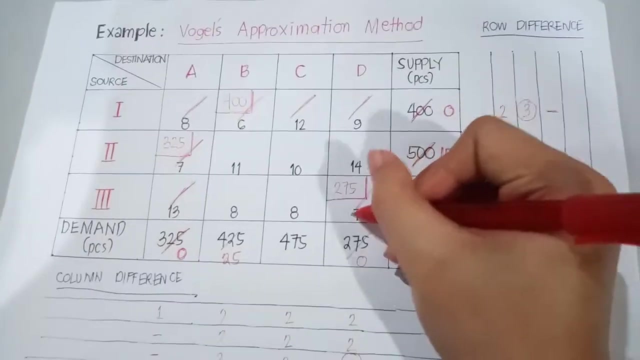 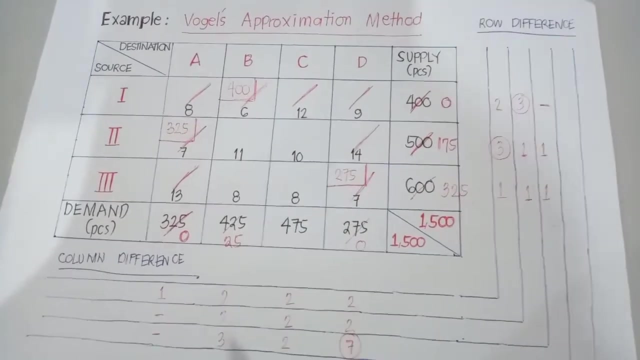 minus 275, so that becomes 325. okay, that's three, two, five. okay now, since this has been exhausted already, then we are now able to mark this out, mark this entire column, as we will no longer be using this column. so, since we have marked that out, we. 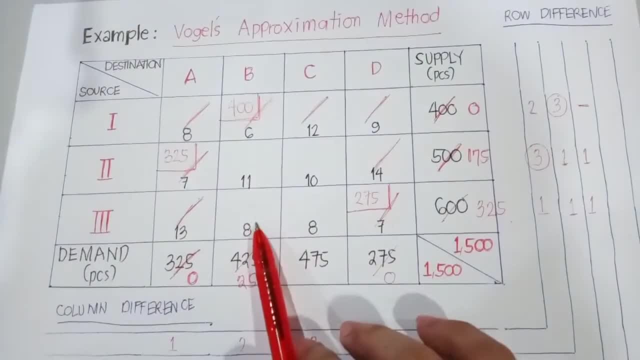 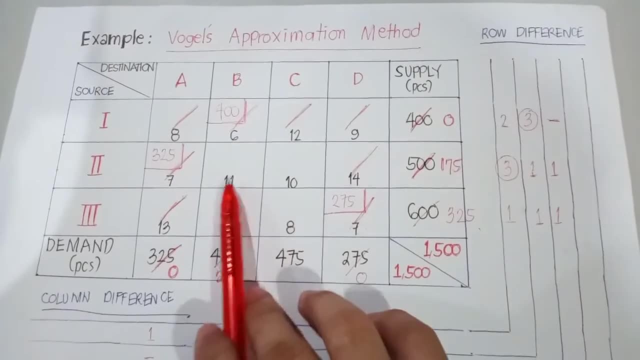 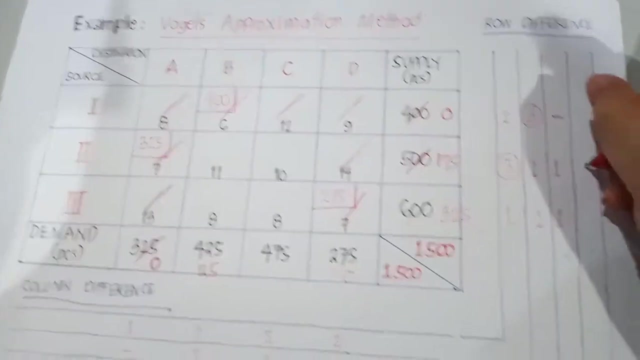 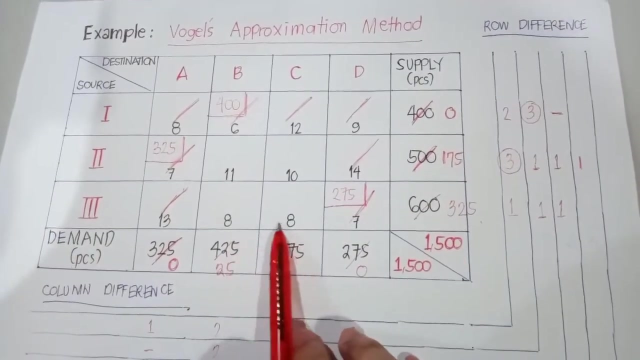 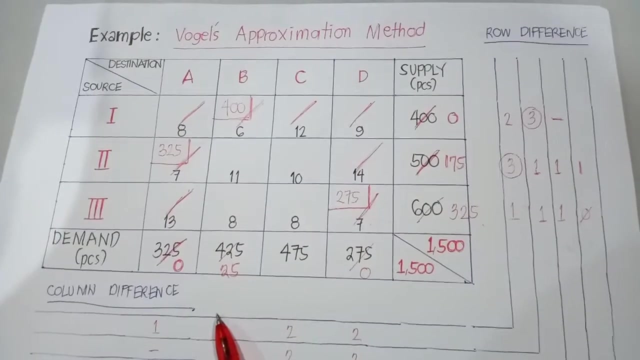 are now left with four cells: 11, 8, 10, 8. so we will now be doing again the row and column difference. so in terms of row two, so i have 10 and 11. so therefore my difference is one. okay, in terms of this row 8 and 8, i have 0 or null, and in terms of column b, 8 and 11, so therefore i 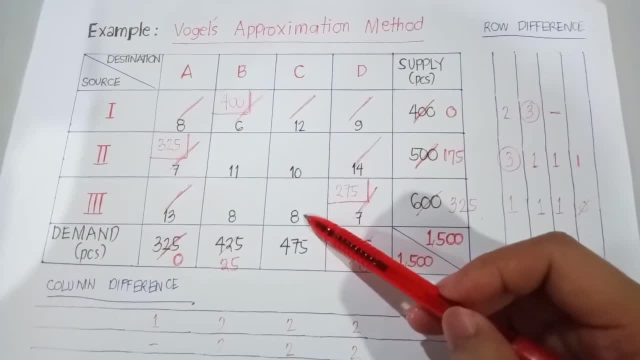 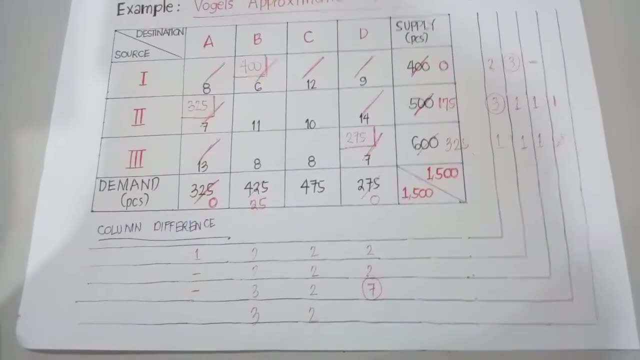 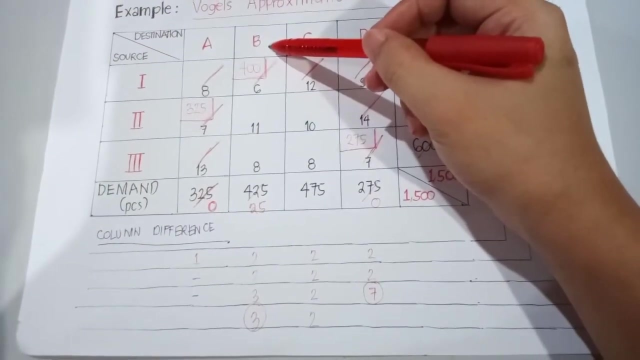 have 3, and, in terms of column c, i have 8 and 10, so therefore my difference is 2. so, looking at the information, uh, the one that has the largest value is three, and three is under column b. so therefore, we will be focusing our attention on these cells. 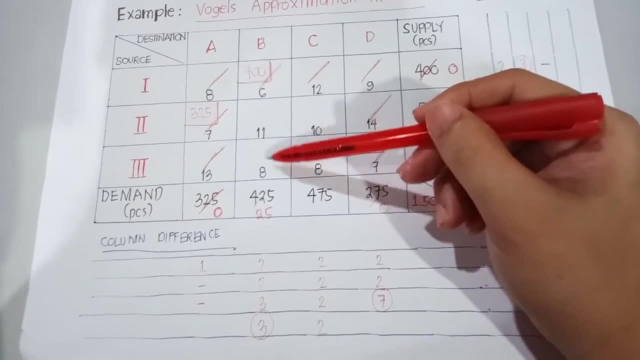 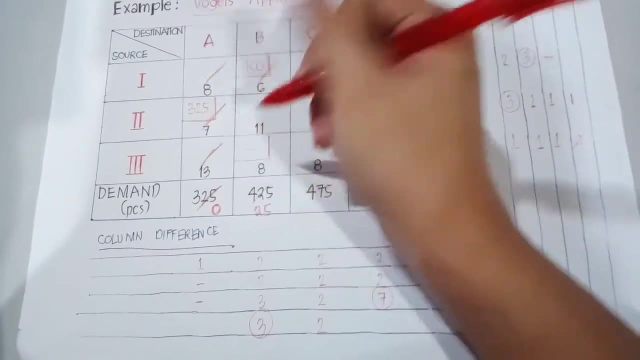 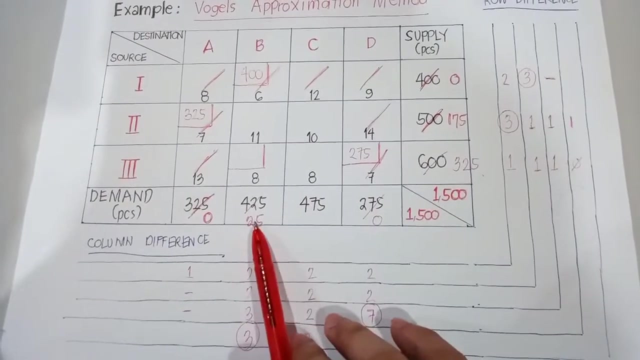 8 and 11, and for this particular cells, 8 is considered to be having the least value. so we will do our next allocation here, and in doing so we need to match the quantity of our demand and our supply. so in this case our demand is 25 and our supply. 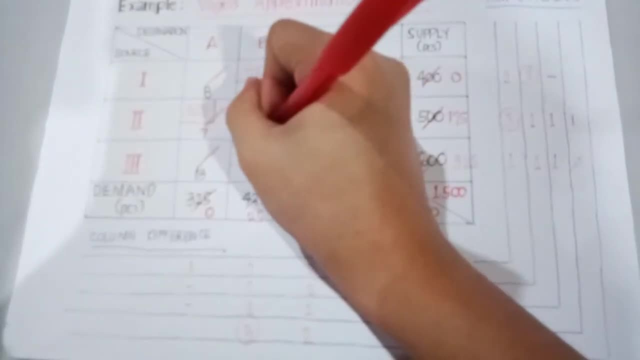 is 3 and 3 is under column b, so therefore we will be focusing our attention on these cells. 8 and 11 is 3 to 5, so therefore i will be allocating the one with the least value, 25, so 25 minus 2, 5 this. 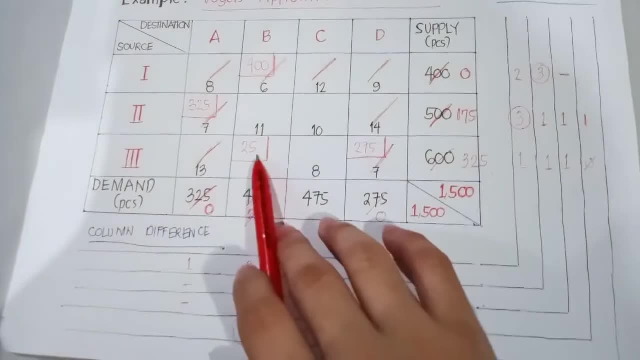 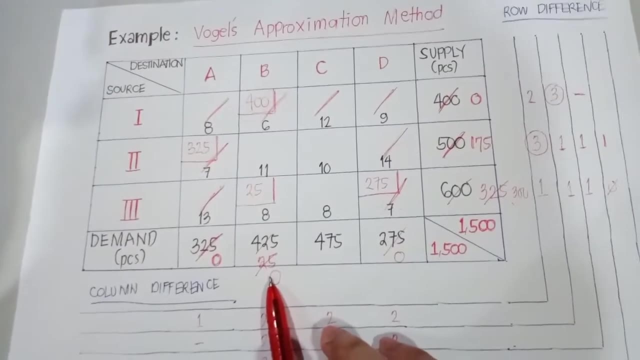 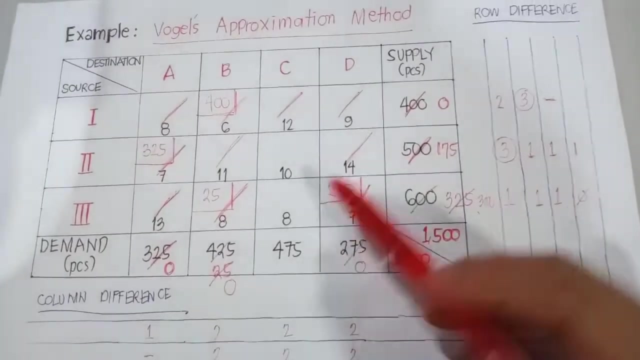 becomes 0 and 3 to 5 minus 25, this becomes 300. okay, so, since this has been exhausted already, therefore, i am now able to cancel out this entire column, and right now i am left with two cells. i have 8 and i have 10. so i am now able to cancel out this entire column and right now i am left with.